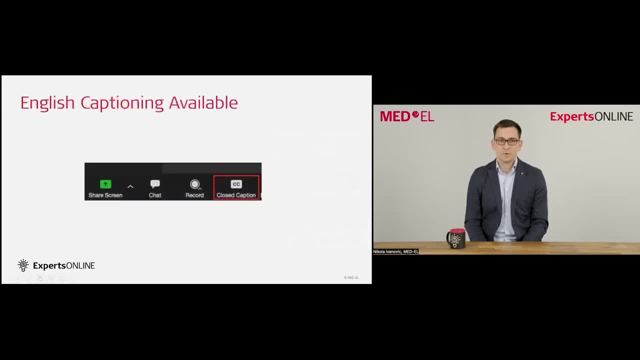 session, and we encourage you to write comments, ask questions, after the official presentations. For easy understanding, we also provide English captioning, and by pressing on the closed caption button in your Zoom window you can enable those and have it visible. Okay, so once again, the topic of today's session is the image-guided surgery. My name is Nicola. 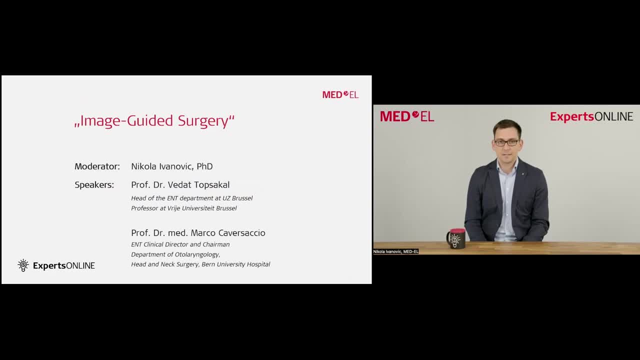 and we have two excellent speakers, experts in the field of image-guided surgery. We have Professor Beda Topsakal from Belgium. He is the head of ENT department at the University Hospital of Brussels and professor at the Free University in Brussels, And he will be talking about autoplan. 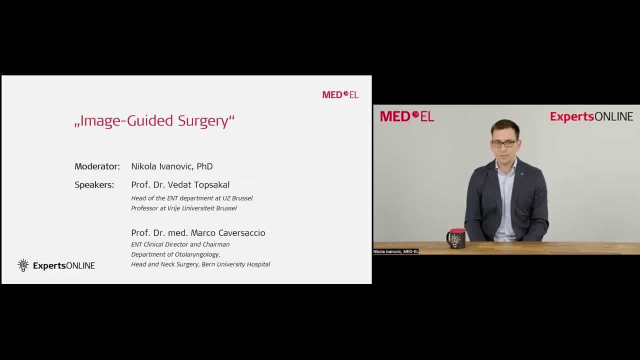 and how he utilizes autoplan as a part of his clinical routine. And furthermore, we have Professor Mako Cavasaccio from Switzerland. He is the ENT clinical director and chairman at the department for otolaryngology, had a neck surgery at the INSA hospital in Bern, And he will be 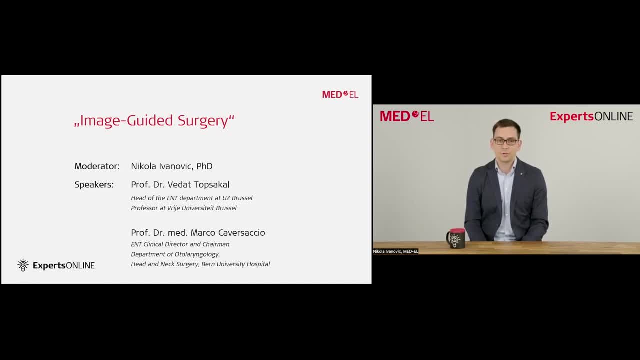 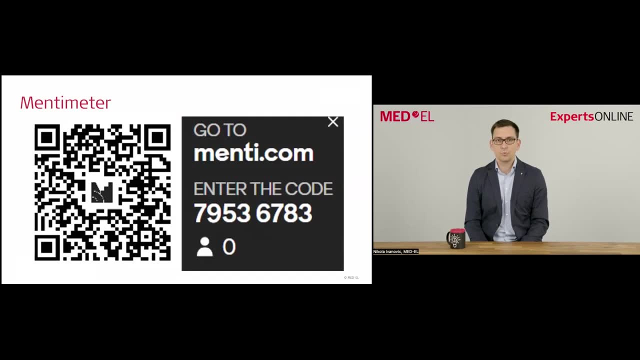 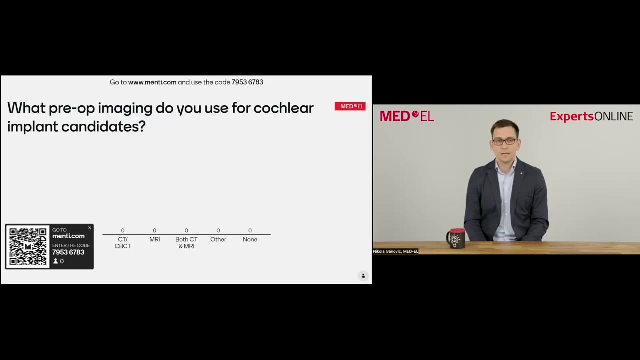 talking about how robotics fits into the future clinical workflow. Before we proceed with our speakers, I would kindly ask you to participate in our Mentimeter questionnaire So you can use your phone and scan the QR code in the top left of your screen or just go to menticom and enter the code. You can use your phone or 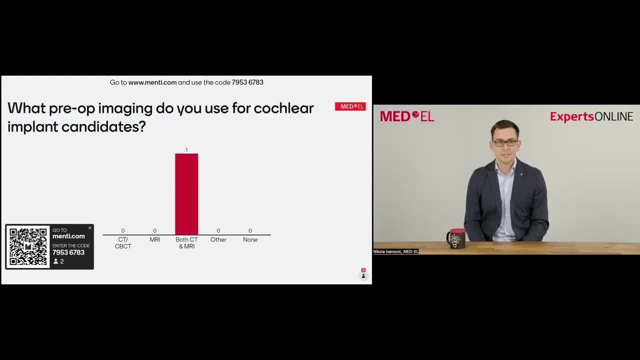 your computer And let's just see how you perform and if you are performing imaging preoperatively for your cochlear implant candidates, just to get a feeling of our audience, As the topic of imaging will be quite present in the upcoming minutes. Okay, so are you performing CT, CBCT scans preoperatively, MRIs or both CT MRIs? 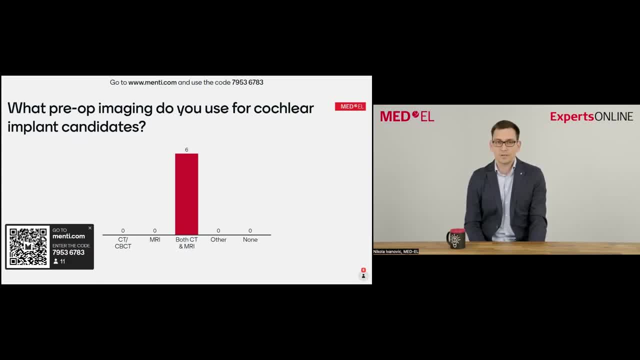 or none, or something else, maybe an x-ray? Okay, let's wait a couple of more seconds. I think this is quite clear. Okay, Let me proceed to the next question. Postoperatively, what kind of imaging are you performing on your patients, your implantees? 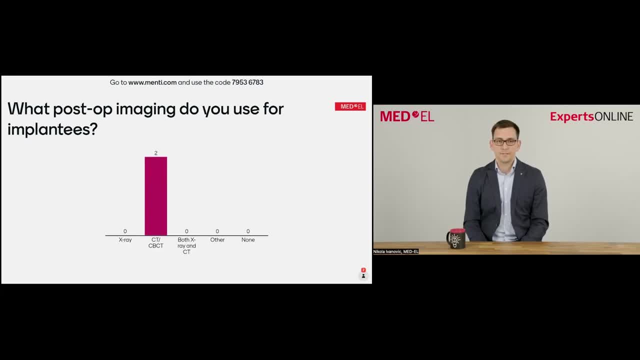 if you are performing any. Again, we have the CT, CBCT, x-rays, both CT and x-rays. What kind of imaging, or none? I think we had nine in the previous. Let's see if we get that. Yes, Okay. 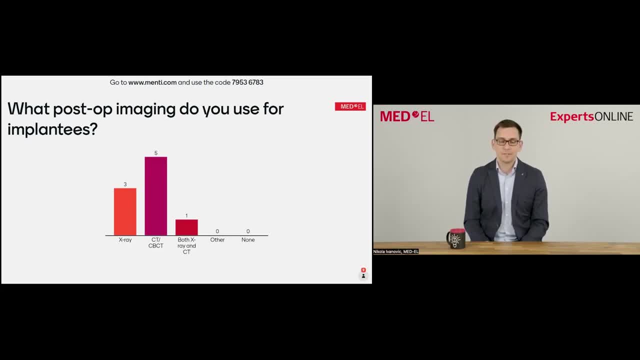 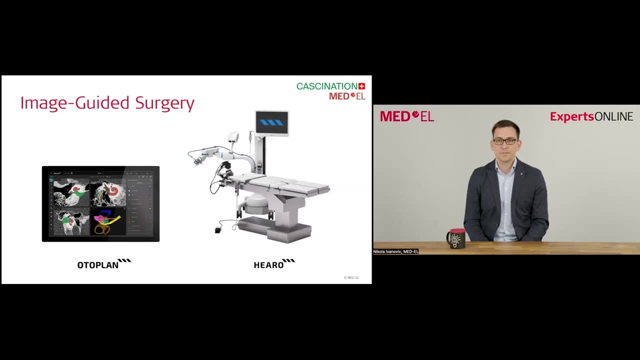 Okay, so most of you are performing also postoperatively, CT and CBCT. Excellent, Thank you very much. We have one more stop before we proceed to the talks of our experts From the MED-EL perspective, when we talk about image-guided surgery. 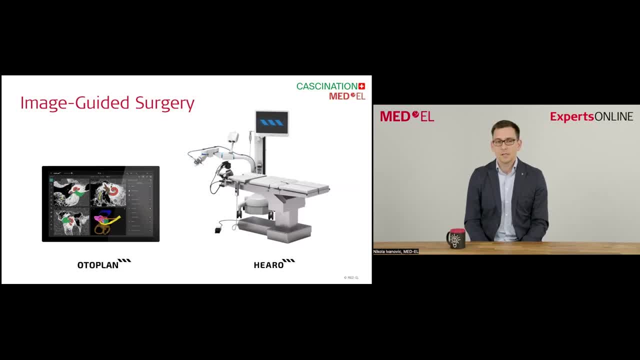 we think? the first thing we think is the Autoplan and Hiero. These are medical devices produced in collaboration with Castination, a Swiss company where MED-EL is the partner in development and exclusive distributor of these Autoplan next slide. 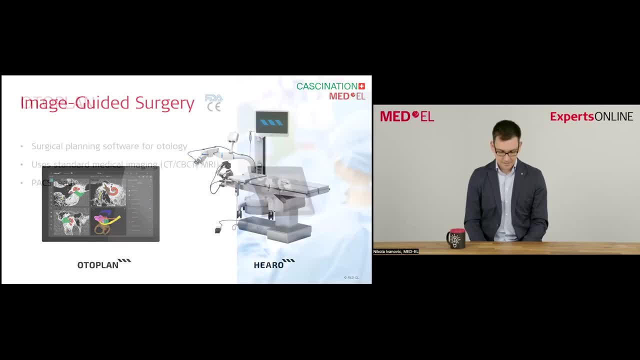 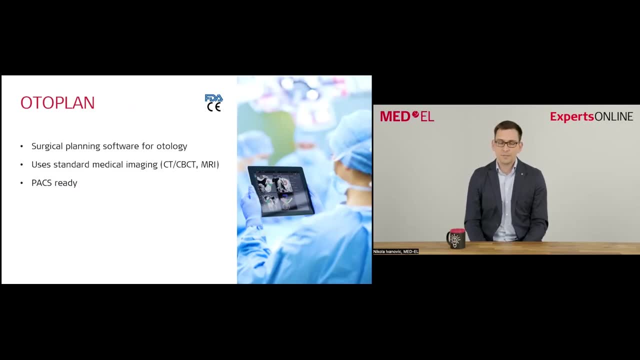 Thank you. So Autoplan is a surgical planning software for general otology. It uses standard medical imaging- CT, CBCT, MRI, so imaging modalities that you were just voting for. so nothing dedicated or special is needed in order to upload to this software And it's. 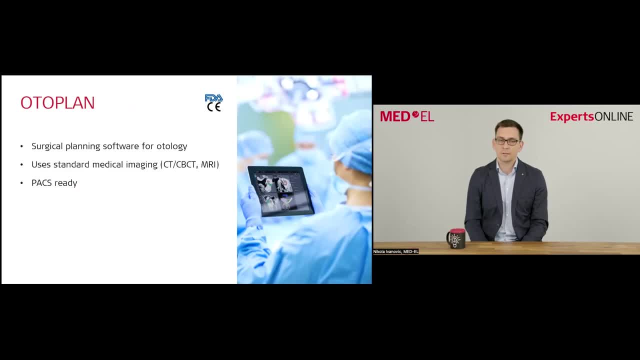 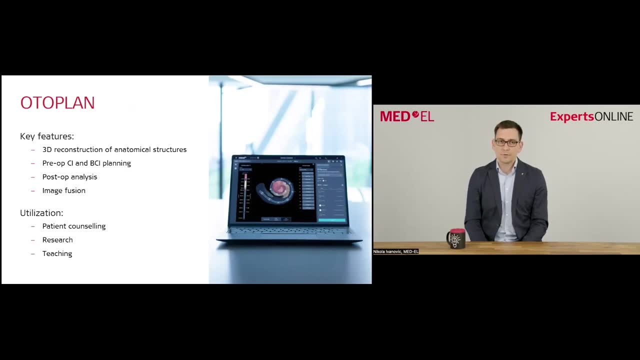 PACS ready, so you can always connect it to your hospital PACS system and pull the data directly from it. Key features of Autoplan are the 3D reconstruction of anatomical structures, preoperative CI and BCI planning- postoperative analysis is also possible- and image fusion. 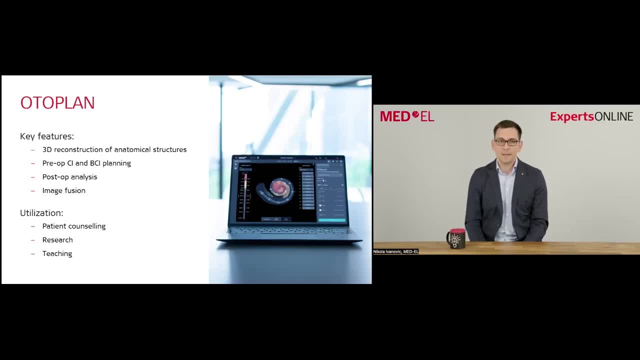 So you are able to fuse the images of different modalities and get the best out of each. Besides regular clinical workflow, which Professor Topsikal will be talking about, Autoplan is also used and utilized in patient counseling, research and teaching purposes. 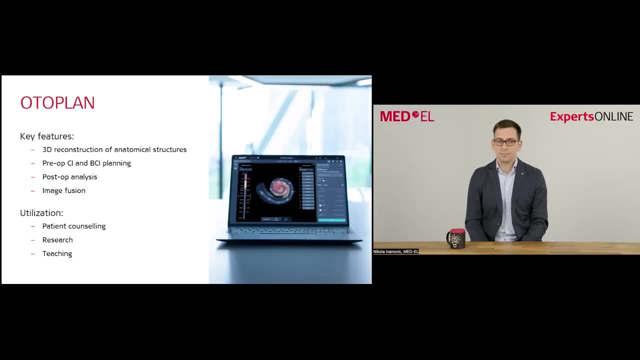 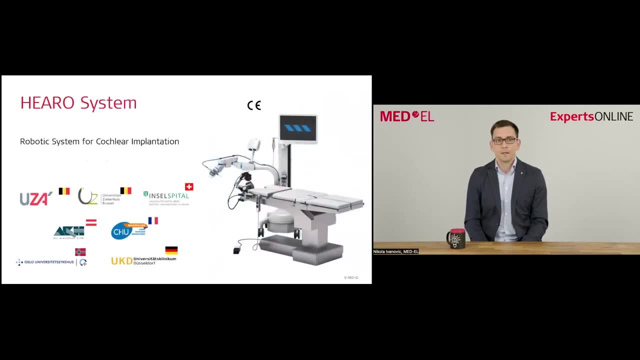 The thing I would also like to mention is CE-marked and FDA approved, And currently we are rolling out the latest version of Autoplan in markets accepting CE-marked. The HIERO system that I mentioned on one of the previous slides is the robotic system for cochlear. 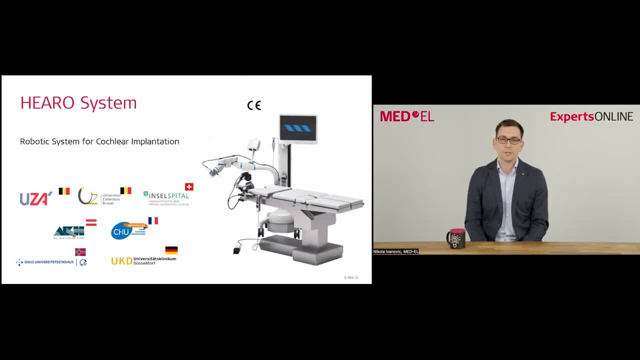 implantation. It uses optical navigation to track the patient and instruments, And until now it has been used in seven clinics in Europe in more than 50 cases. So more than 50 patients were treated with the system And again, we will hear more about it. 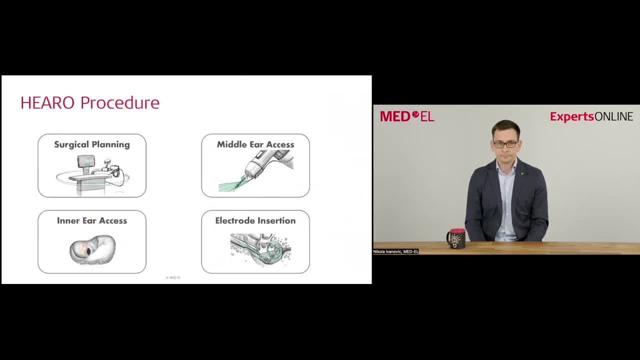 from our speakers in the upcoming minutes. The HIERO procedure consists of four main steps. The first one is the surgical planning, which is done on Autoplan software. Then there is the middle ear access, inner ear access and electrical insertion And the 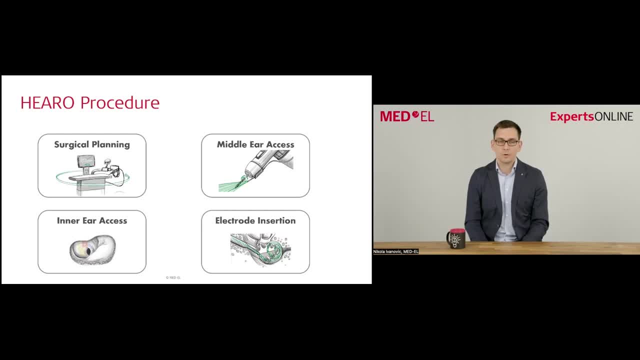 procedure that we have today we have thanks to our experts who will be talking today. Professor Cavasaccio was the first to perform the middle ear access with the robotic system and Professor Veda Topsakal was the first to perform the inner ear access. He extended work of Professor Cavasaccio. 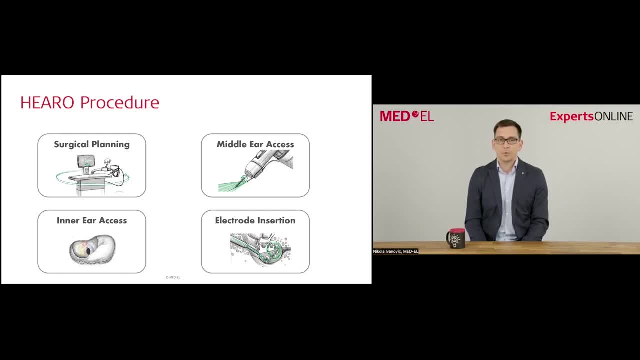 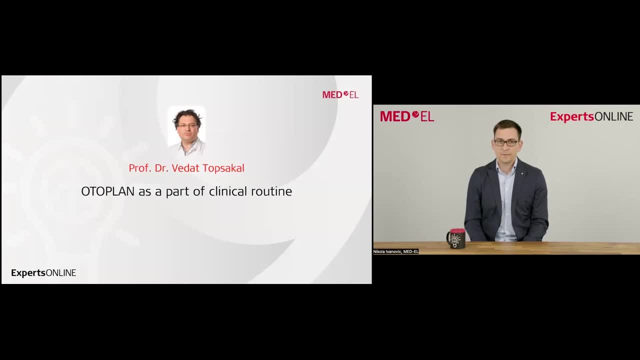 and we use this procedure now in all other hospitals as well. At this point I would like to hand it over to Professor Veda Topsakal, who will give us more insights about Autoplan and how Autoplan fits into his clinical routine and how it's used. 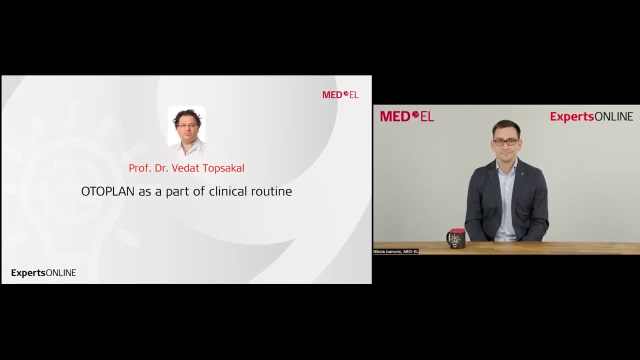 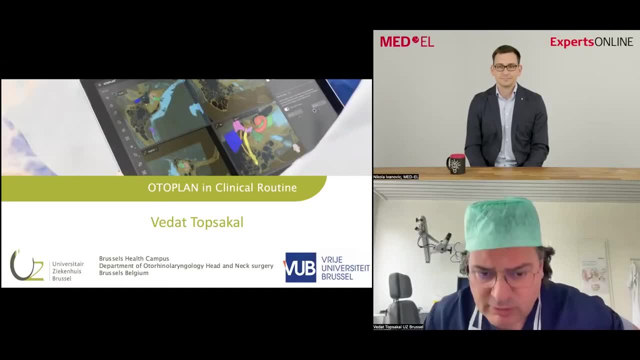 Professor Topsakal, the floor is yours. Thank you very much, Nicola, also for your kind introduction. My name is indeed Veda Topsakal. I work in Brussels and I would like to thank also MED-EL and the steering committee of these online. 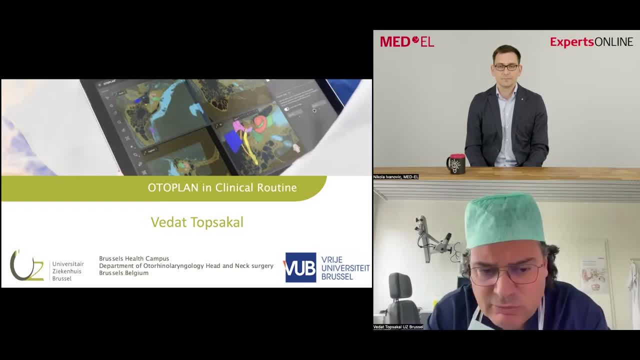 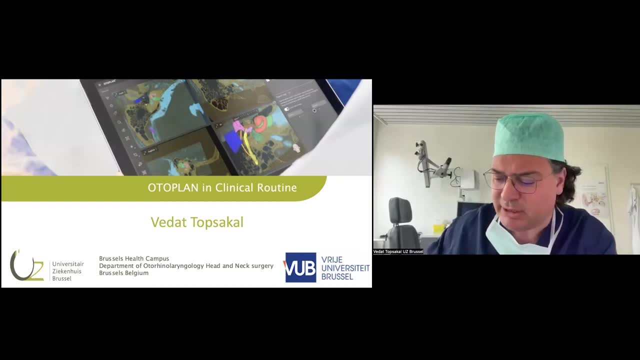 sessions for inviting me. together with Professor Cavasaccio, It's really an honor to speak also about our, let's say, first experiences of Autoplan. I guess we could say we were early adopters to this, to this new technology, and I have to recognize in this my colleagues from Antwerp. You see here, Professor, 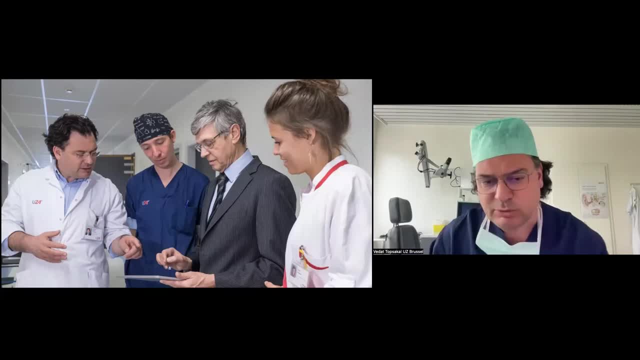 Paul van der Heijning, who I pulled into robotic surgery before he was retiring, but he was also one of the first to say that Autoplan should be a standalone in clinical workflow, because this tool is also of benefit of general autology on itself and not only for robotic and image guided surgery. as you spoke, 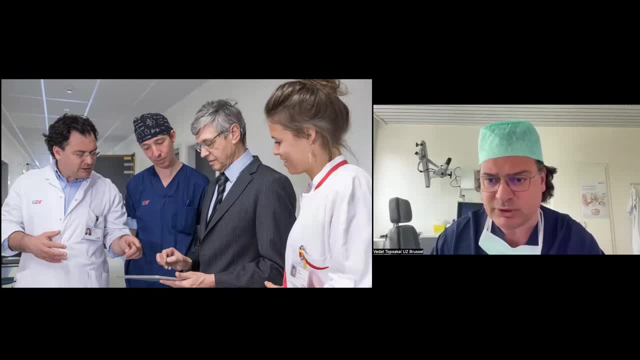 about just a minute ago. So I have to recognize also Giet Mertens, on the right side, who did a lot of, let's say, audiological, electrophysiological work with Autoplan, who was together, and also Vincent was very supportive in Antwerp. Now, one of the first things we already 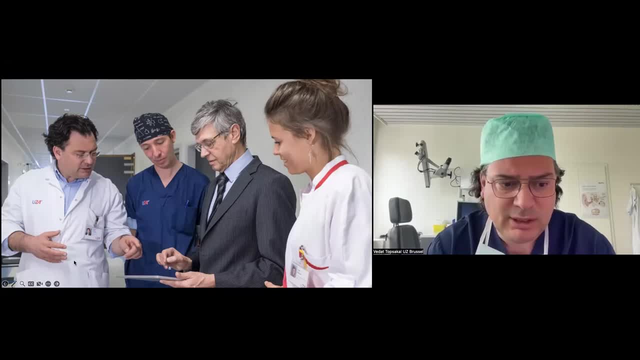 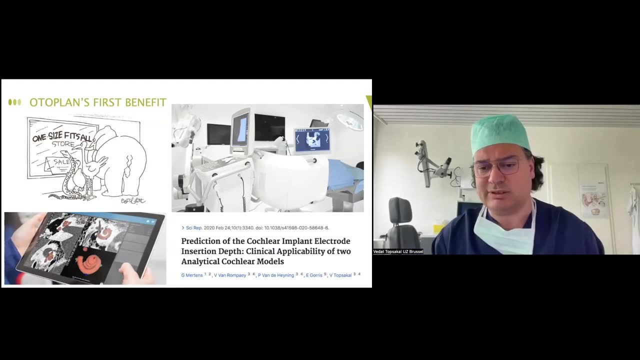 I have to admit a lot of people into this meeting. Let's see if I can proceed to the next slide. Yes, one of the first things we would have to acknowledge that Autoplan puts our nose to the fact that not every cochlea has the same size. This means that maybe somebody else can let in. 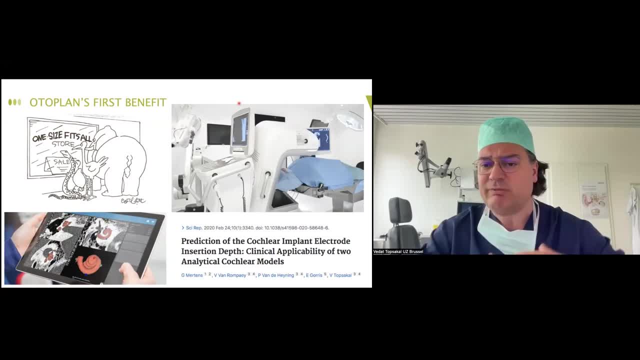 all the other listeners. This means that when you have the high tech, you know the jet set technology to image the cochleas- you should also recognize that you know one size of an electrode array does not fit all. So this was one of the first works. I think it was one of the first versions of Autoplan. 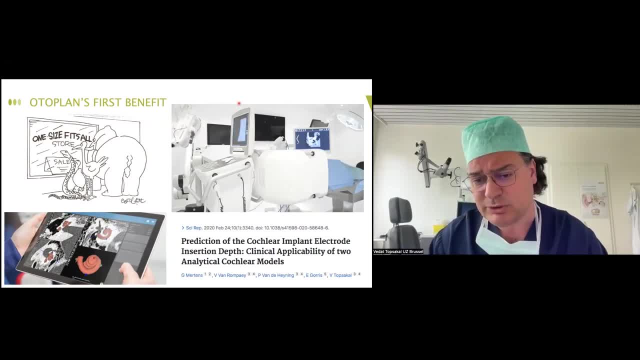 maybe even a research version, where we, with our research group in Antwerp, try to find out what is the inter-observer or even intra-observer variability of dimensions of the cochlea we could measure, and was this feasible for clinical purposes? and we could conclude that it was. 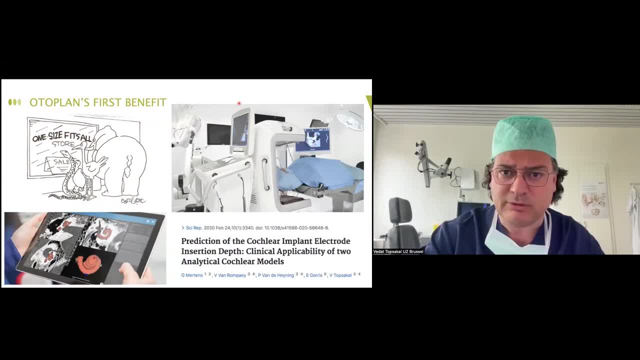 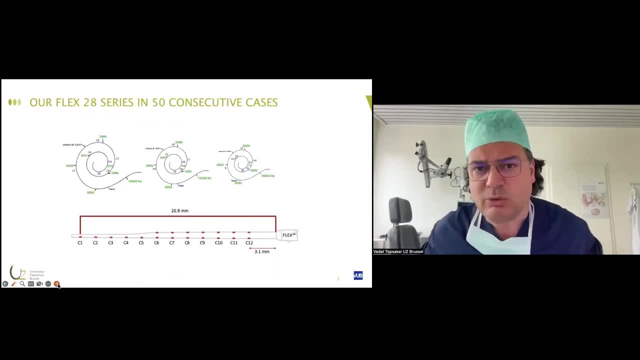 feasible for clinical purposes. So from there on we continued So, and immediately a new study came up into our minds. I mean, we took, let's say, about 50 consecutive cases from our clings where we placed the flex 28 electrodes, because in those times we had the 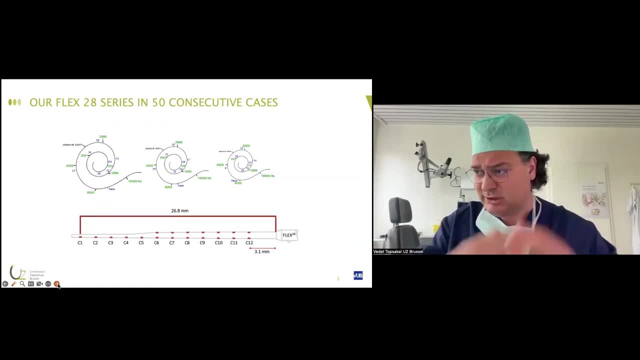 idea that 50 percent of all cochleas were on average covered with 28 millimeter because of the early work of Hardy that she measured the cochlear duct length. But it turned out not to be really true because if you look at these 50 consecutive cases, you can see that some of these cochleas were 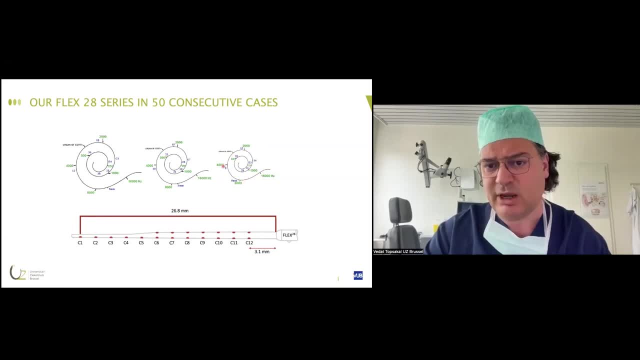 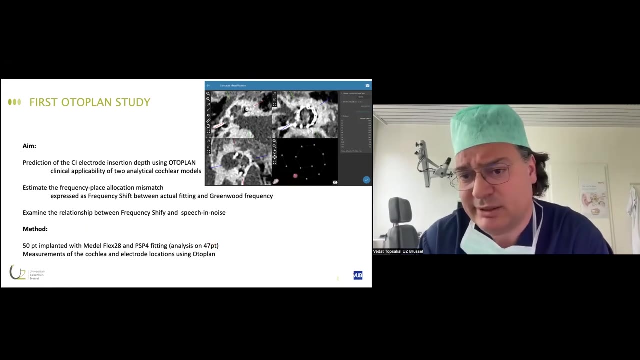 even shorter. So here we had, with the flex 28, a rather deep insertion, and whereas the cochleas were longer, we had a rather shallow insertion. And if we looked at those data together with Geert Merkens in that time, I have to also say that Autoplan was really in a version that we 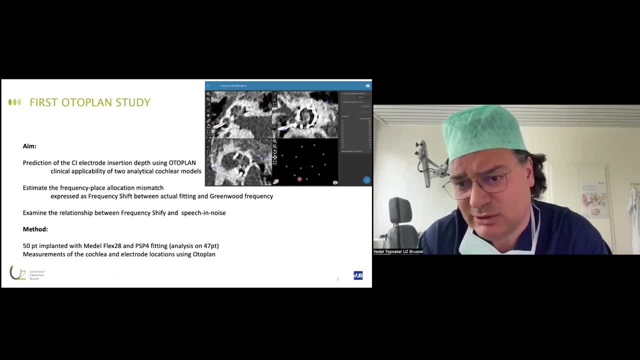 needed to find, together with Geert Merkens, the error of the cochleas, And that was in the case of Autoplan electrodes in the cochlea, depict them and point them out and segment them, so to say. But I will get back to that in the latest version of Waterblende. We could conclude that, yeah. 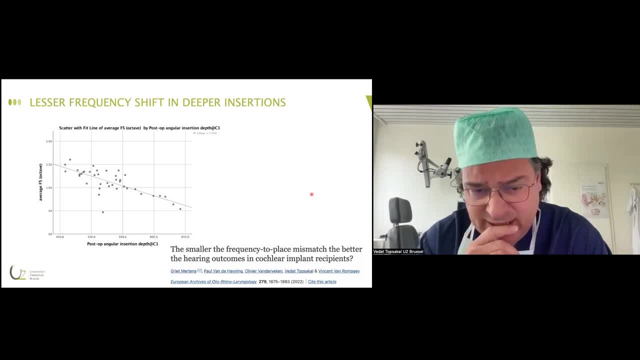 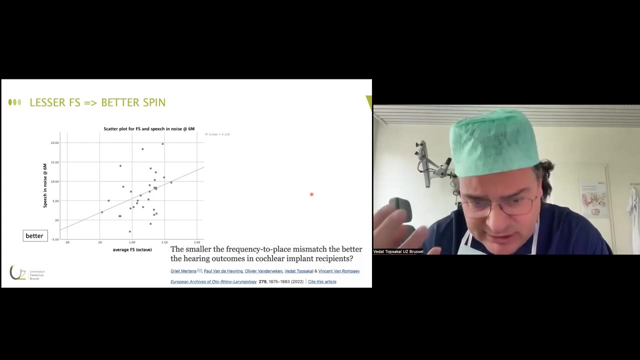 there's more frequency shift when there is a more shallow or less deeper insertion, And keep this in mind, because also our latest research on this topic hints towards the same. Well, what does that mean? If you also look at these data sets, the lesser the frequency shift is actually also the 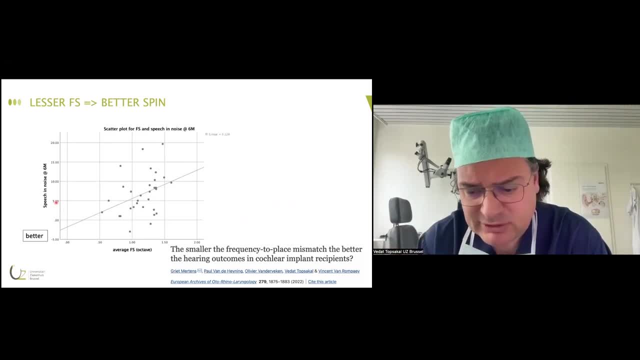 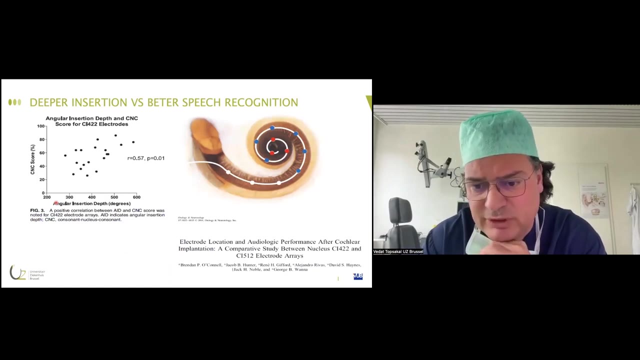 better the speech and noise scores were, And this is not a new finding In this series. we could also only substantiate this for the first six months with the ABF we did. But it is also known in literature that the deeper the insertion is, the more cochlear coverage you have, the better. 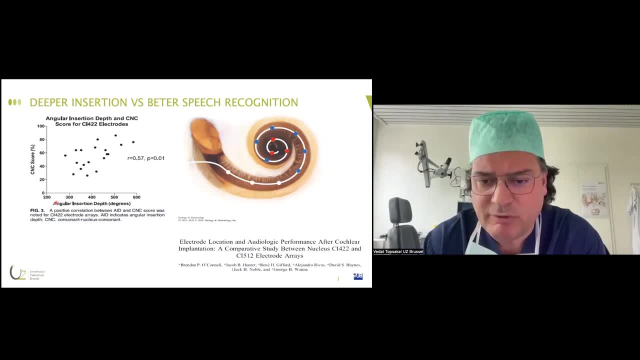 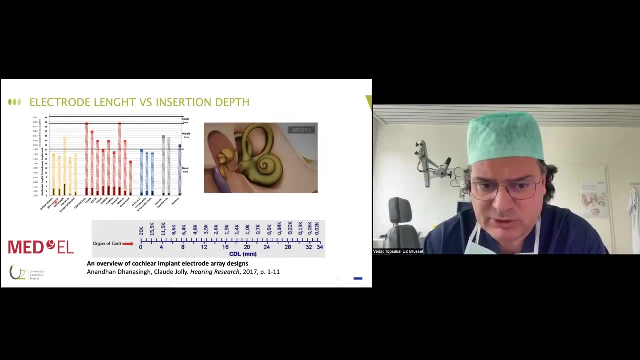 outcomes you could have, or let's say, speech performance you can have- from your cochlear implantation. So it's a bit surprising that not all manufacturers jump on this. but you can see the, the, the gamma of, let's say, the portfolio of all manufacturers, how much they cover of. 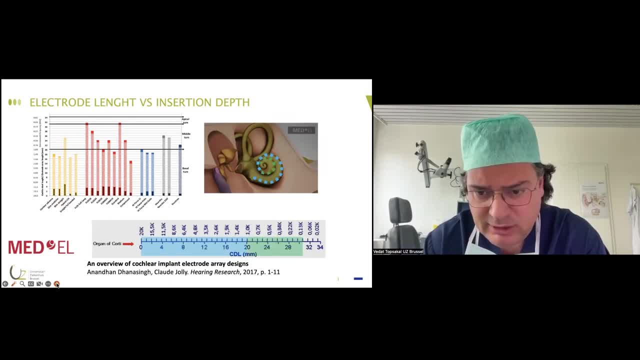 the cochlea, And you see here also a little bit of an outdated slide, but because in between the Med-El portfolio has been extended with the Flex26. even So, the manufacturing supplier supplies what we would demand for, but what is in demand, And this is something. 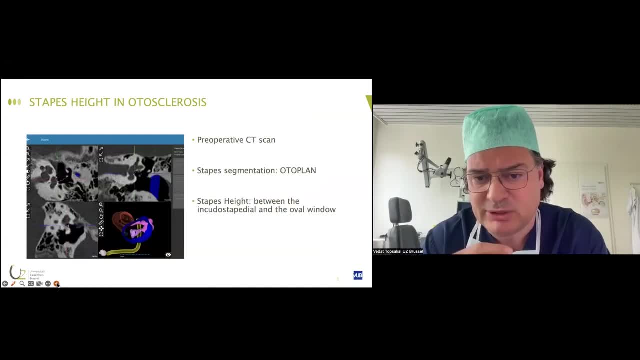 that's a decision between you and, of course, your patient and how your patient presents itself with the hearing loss. Again, that fact- I will come back to Another clinical study we actually are performing at this moment, very moment right now- is that we also look into the 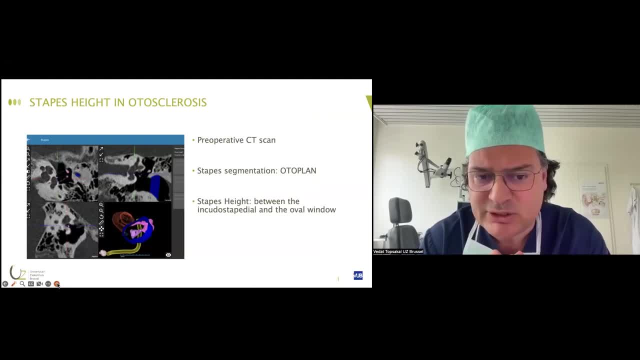 ossicles with Autoclan. I mean Autoclan provides also information on other temporal bone structures. One of the things you could measure is the height of the stapes. Again, here, it was with the oldest version that we have to, let's say, segment or point out three points of the stapes, and it could give 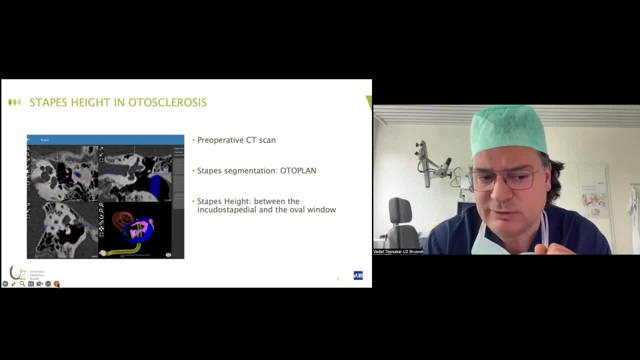 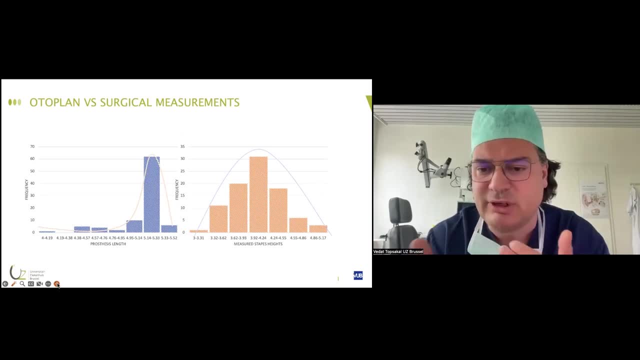 us the height of the sphagus. Why would that be important? Well, of course, for the people who are into stapes surgery, it's always a bit of a burden to measure the length of of the stapes or the length of the prosthesis you would want to choose. We took, let's say, 90 consecutive cases of the course closely. 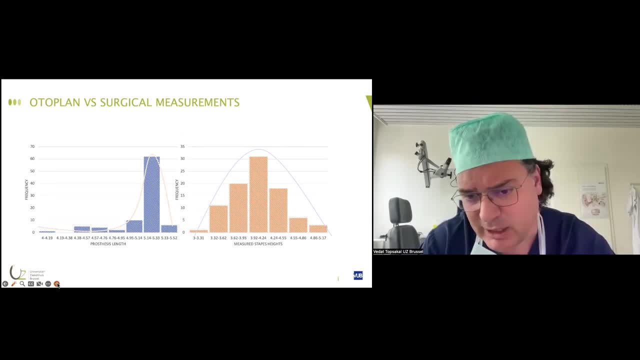 of my predecessor, Professor Frans Kortz, and we measured on the preoperative scan- because he always performed the preoperative scan with autoplan- the height of these tapestries And you can see a quite normal distribution with the average length on around four millimeter. And 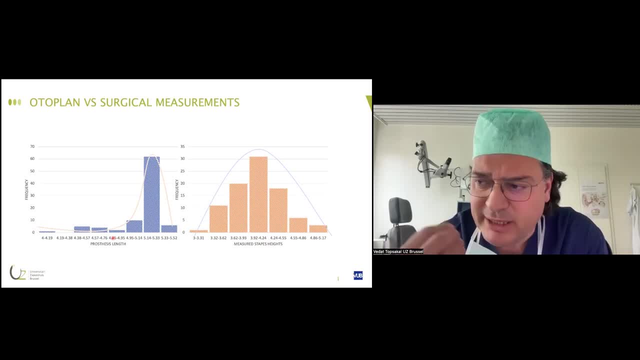 we also looked at what he measured and placed. Unfortunately, not all the operation reports report on the fact what he measured. but it also was for us surprising to see that he had a, let's say, preference for a 5.2 FISH prosthesis, which he used most of the time. So this was a bit 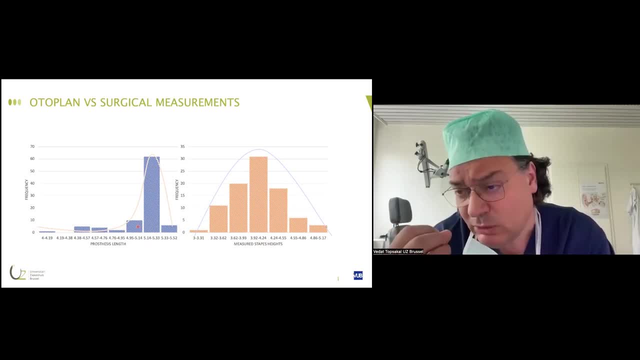 of a skewed distribution. It only shows that autoplan is quite accurate in measuring the length, And it was also reassuring to me that my preference as a stapes surgery is a 4.6 millimeter prosthesis of what's called a loop that I cut. So here you see the normal distribution and the 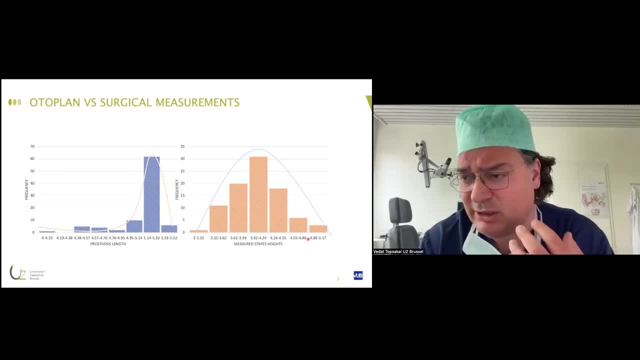 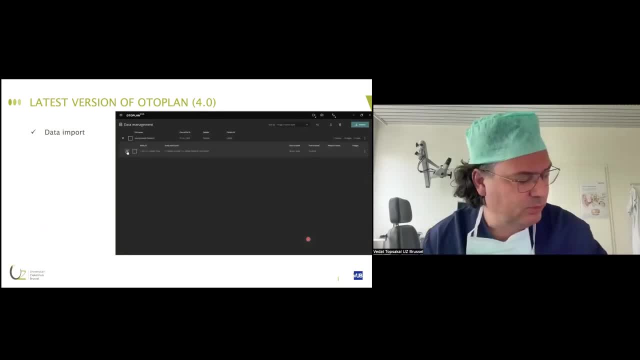 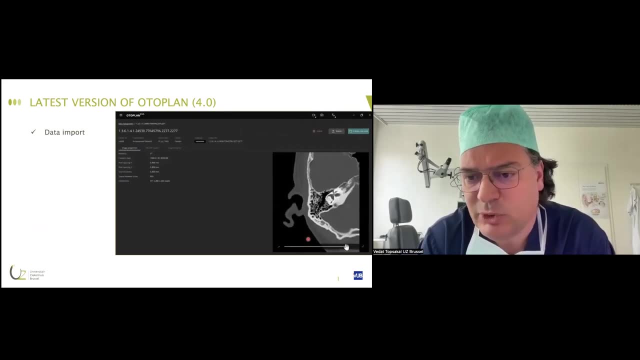 cochlear implant surgery. Coming back to the latest version here, you see how fast it could go if your autoplan system is connected to your PACS, that you can, let's say, upload or download whatever you want to say, take the images from your PACS system and put them on autoplan. This 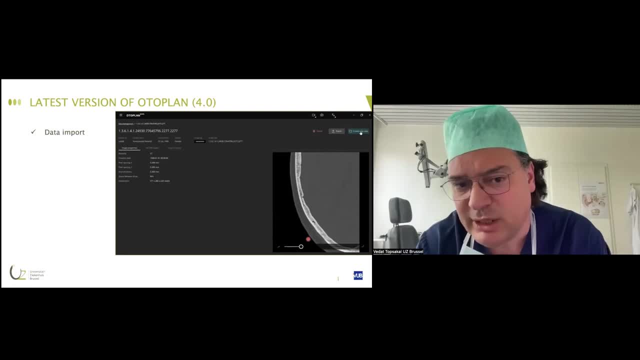 is really faster than in the beginning days where we had to, really unfortunately, go to radiology, radiology and connect a device. All these efforts are there to make us a bit more into independent of the radiology department. We can do this now ourselves. We don't need to, you know. 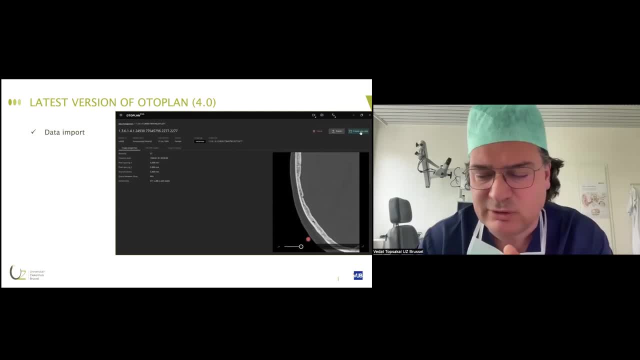 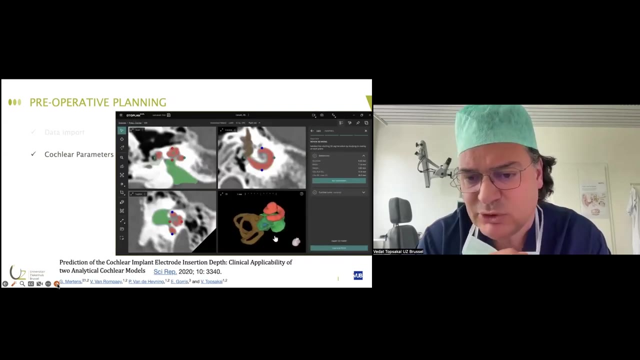 be a burden to radiologists and please ask and demand: No, no, Even our audiologists can do this or residents can do this in training. Now, in the next slide, you see something very spectacular. I mean, this is the newest version of AutoPlan that really segments the crucial anatomy fully. 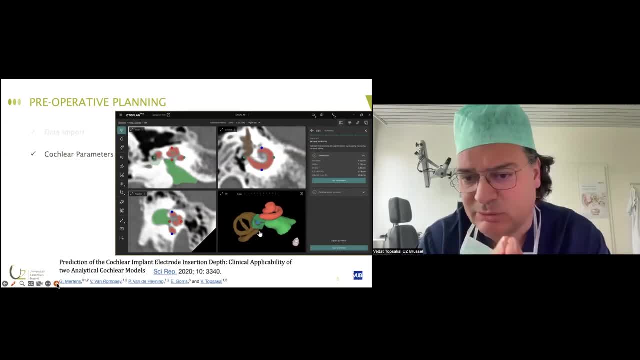 automated. I mean, you can say it's a calculating algorithm, you can say it's artificial intelligence, whatever you want, but it's for sure something that has less inter or intra-observer variability. So it really outperforms our first study and it outperforms the, let's say, human segmentation. 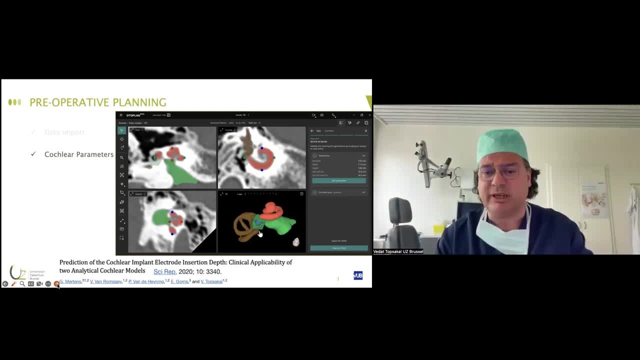 of dimensions and the calculations of the cochlear duct line, because it's based on a mathematical formula to depict the points for the calculation and it does every time the same or with a much more higher accuracy. And this is perhaps a game changer, Not only 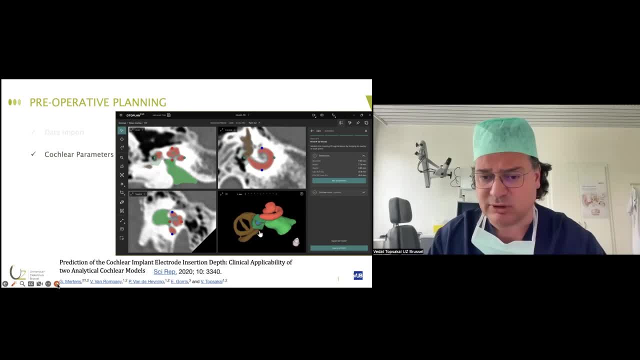 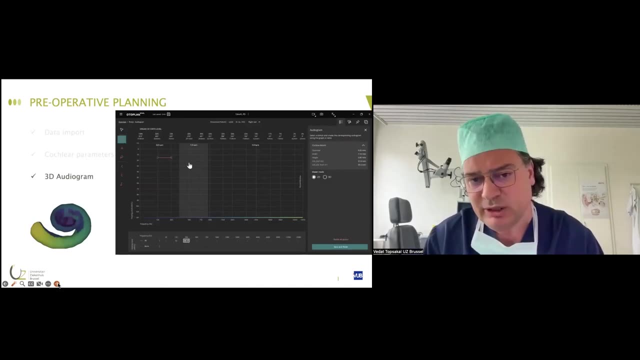 does it require any more radiologists or a trained autologist? no, audiologists can do this. but it's also a game changer on a different dimension. I will get back to that as well in a minute. It also gives you the possibility, the AutoPlan version, to show or put in the data of your 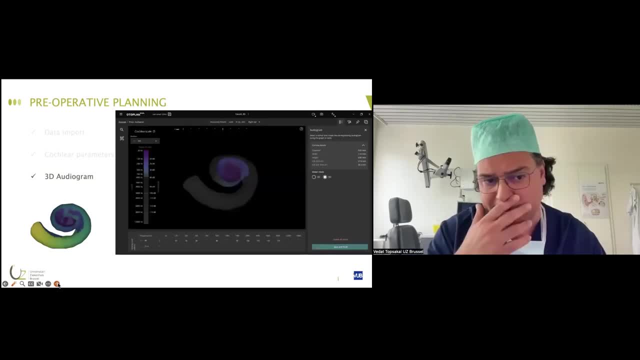 audiogram And you see on the left corner a cochlea. that is a normal hearing cochlea but you see in within the picture centrally. you see the audiogram we put in. there is a high frequency hearing loss. there is some residual hearing there. that was represented. 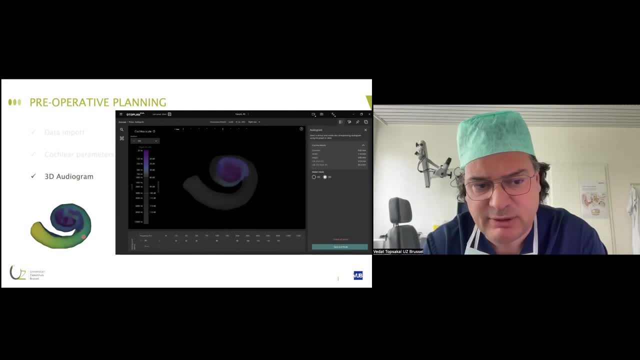 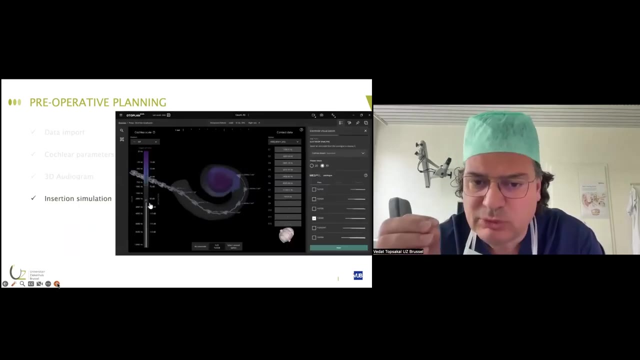 by the intensity of the colors and the frequencies are represented by the colors that are changing. So this is a 3D audiogram that you can put in. Why would we want to give you this feature? Well, for the basic reason that it's also up to you, together with your patient, to decide which length 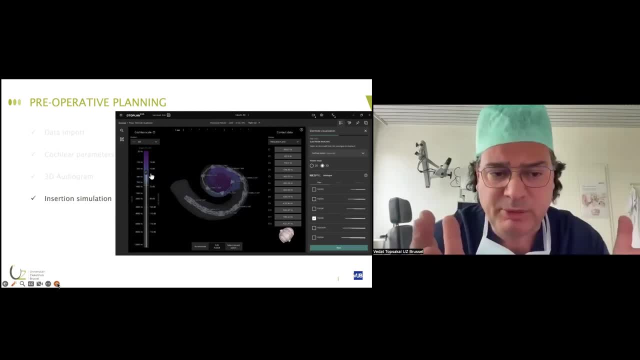 are you going to use? You know, it's not that you measure 32 millimeters and you say, okay, I can fit in the Flexsoft, No, no, The residual hearing is also a parameter that you need to discuss with your patient. What do you want? You know your hearing loss is perhaps very. 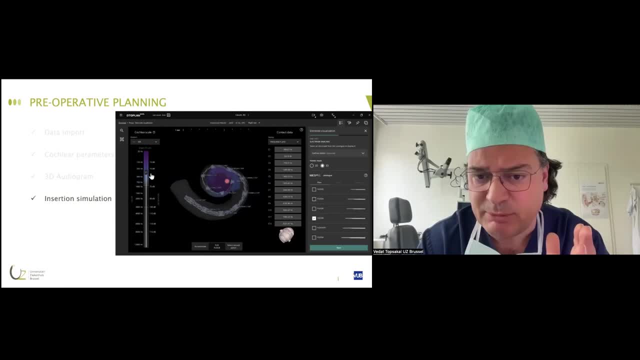 very progressive. But you can also use it to measure your hearing loss. So you know, if you have some residual hearing here, but probably it will be gone next year or in within two years, we will go for a full coverage and a full length, Or you will say, no, your hearing loss has been. 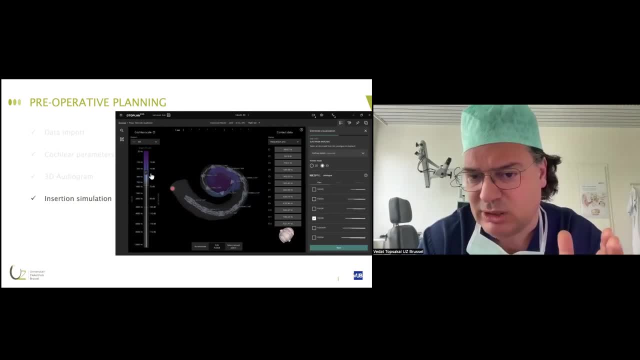 stable over the last 15 years. Maybe we can even try to preserve that hearing loss, or even, if it is a better residual hearing, we can go for electroacoustic stimulation. These are all very nice counseling- I mean moments- and you can use the AutoPlan as a tablet or even on your desktop. 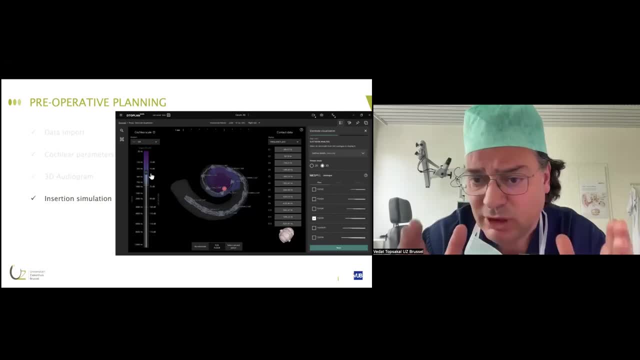 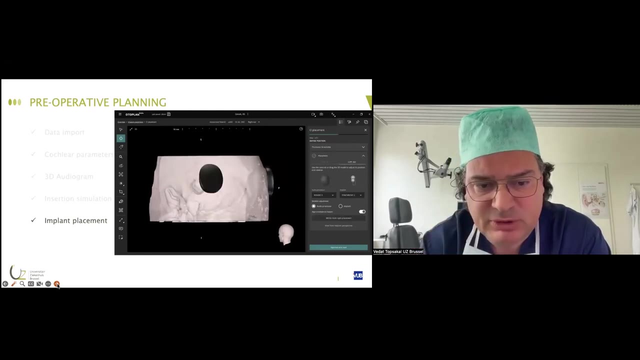 Together with your instruments in your outpatient clinics to counsel and to see what that patient wants and what would be the best for that patient. Now, other new features are also that you can segment where the implant placement is. Why is that important? Well, it's another. let's say: 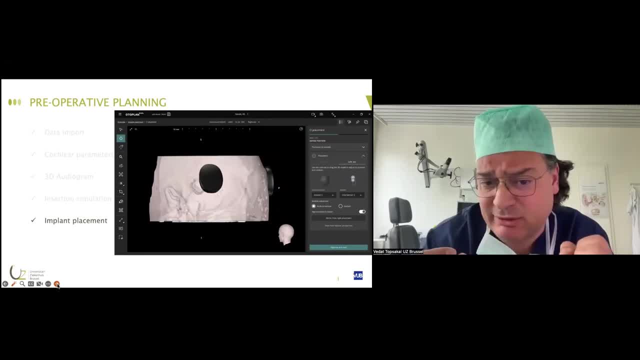 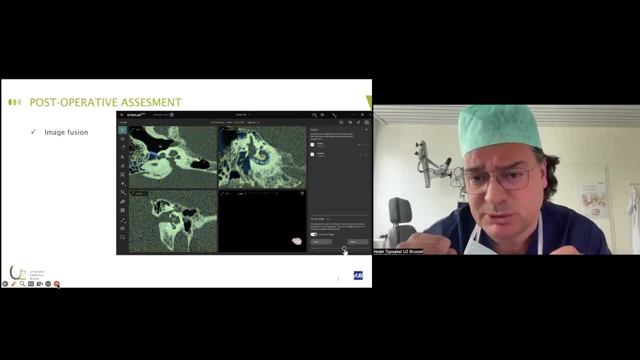 standardization or quality parameter, especially in bilateral cases. You know you can try to work as symmetrically as possible because these are the smallest things that the patients really very much appreciate. Another very nice feature is you can fuse images- the pre-op and the post-op CT, but you can also fuse the MR images with the CT. So 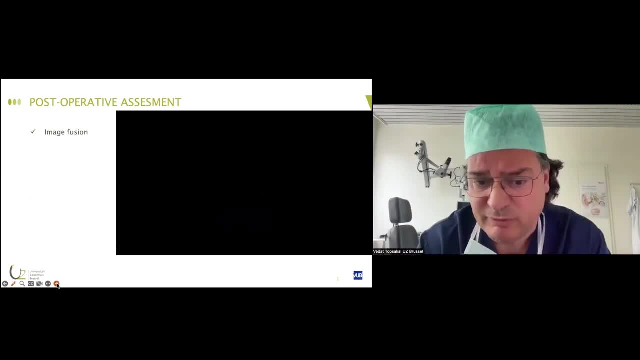 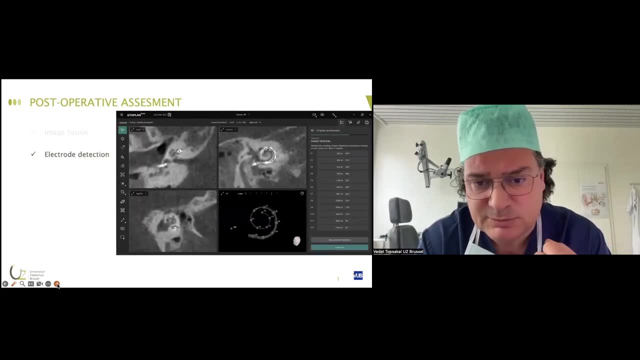 as I said before, use your imagination, because this tool is too powerful to think of whatever possibilities there are in terms of research to pursue actually better care for our patients. The electrode detection I pointed out in the beginning, which we did manually, now is also 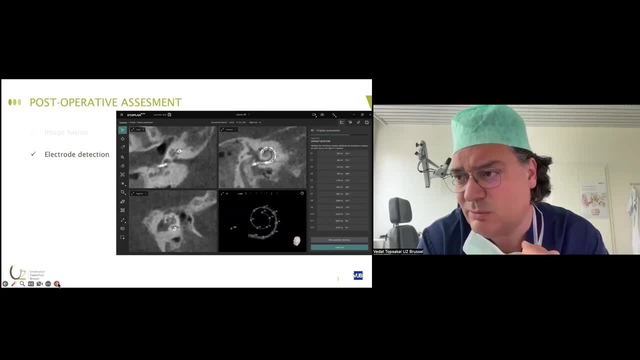 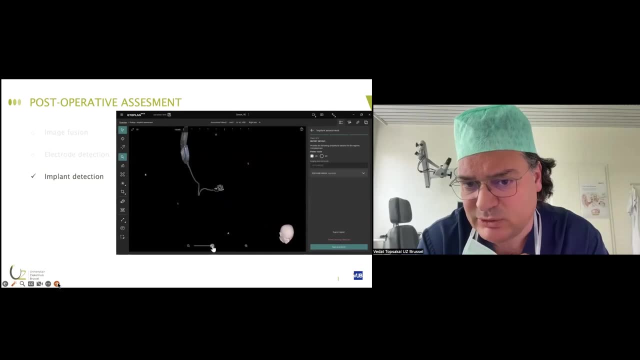 fully automated, And this enables an audiologist to segment post-operatively where all the electrodes are and even continue with anatomy-based fitting. Not only that, it also detects the implant, and it could be in the near future that your audiologist say, oh, but you should take care of. 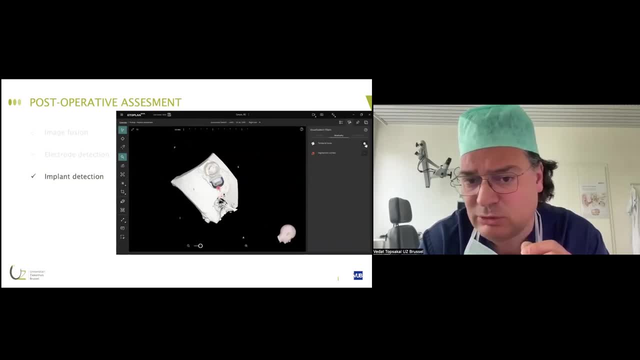 the fact that you should perhaps guard two centimeters between the implant housing and your mastoidectomy. or you know another parameter to standardize: standardized the surgical outcomes to help us to perform even better care for our patients In terms of anatomy-based fitting. I have to apologize for the chaotic slide here, but 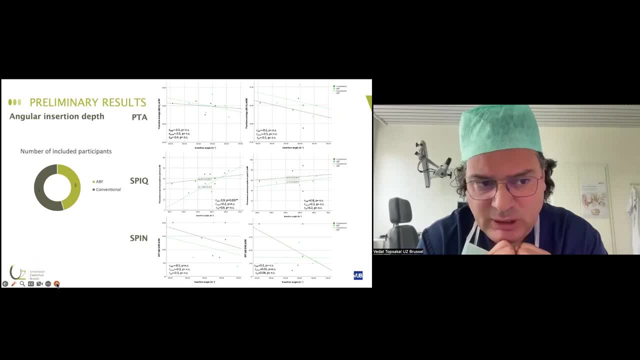 these are very, very preliminary results of the limited numbers of cases. We've put five patients into a study in a randomized controlled trial, actually with anatomy-based fitting, and we compared them to conventionally fitted cases. And all of the slides you can see in pure tone average, but also speech and quiet and 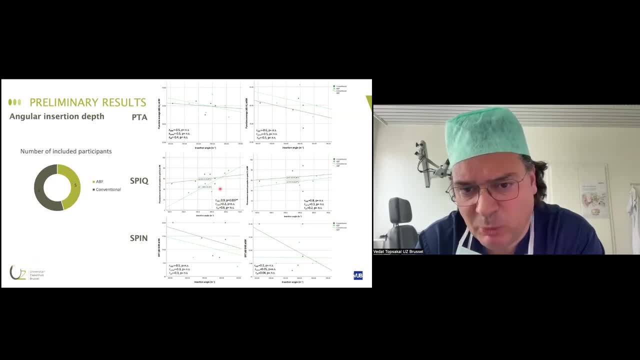 speech and noise perhaps not so much, but there is an overlapping moment. So, as I said in the first slides, in our first studies, the deeper the insertion, the more cochlear coverage you have, the better the performance. It also shows here that anatomy-based fitting probably is even more likely to perform better. 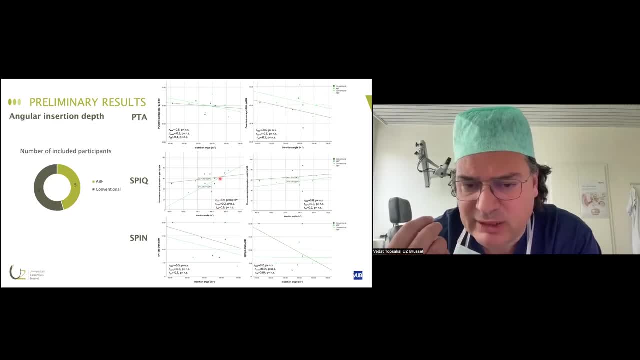 when you have the right anatomy-based fitting. So you have at least over 600 degrees of insertion. Again, this is only in effect for, let's say, the first six months of follow-up we have. but we want to enlarge this group and we will surely get back to you with these data. 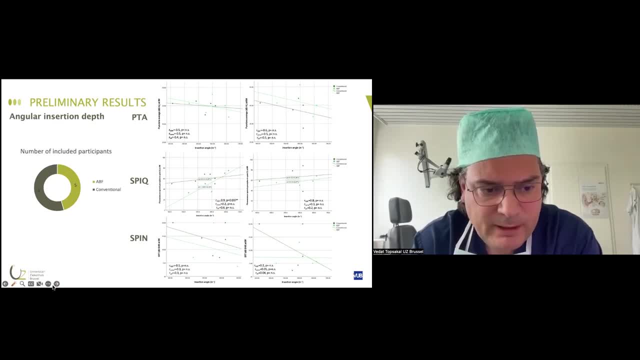 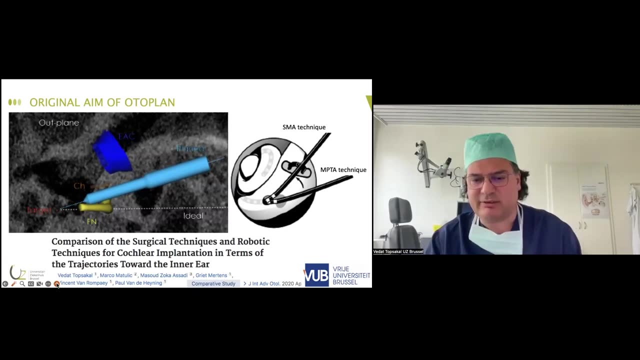 in the near future. Now to come back to why AutoPlan was designed: it was designed to enable image-guided surgery Also. this we've studied- and I have to admit that I did my share- of supermedication and supernatal approaches. 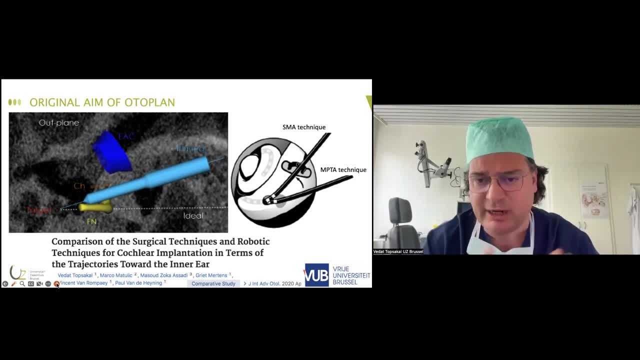 We also compared that, how the trajectory or the insertion angles would be when you compare to the more, let's say, standardized or the golden standard of posterior tympanotomy. And yes, for the moment you have to enter the cochlea through the round window. 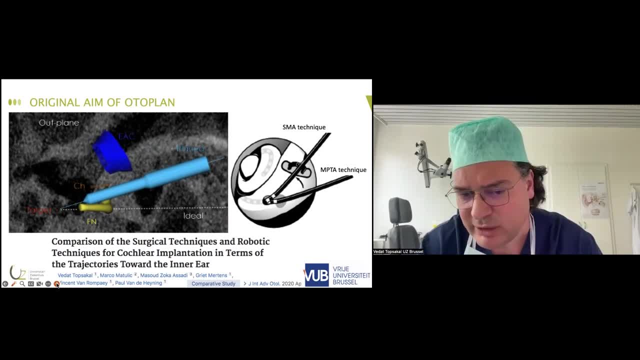 We don't perform any cochleostomies anymore and you have to try to stay as long as parallel as possible with the basal turn. Well, if you define it like that, the facial nerve is in your way, so you have to adjust. 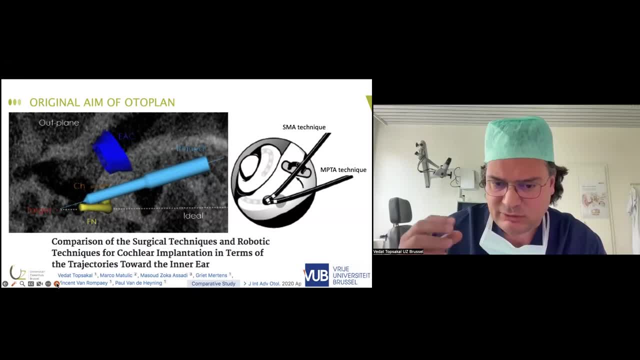 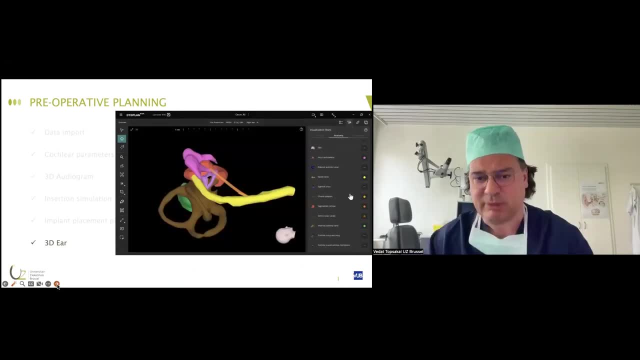 adjust it. Now. it's one thing that the surgeon segments all the anatomical structures, but with the latest version we have now AutoPlan that's fully segmenting the 3D anatomy of that case. So it makes another leap towards the future. 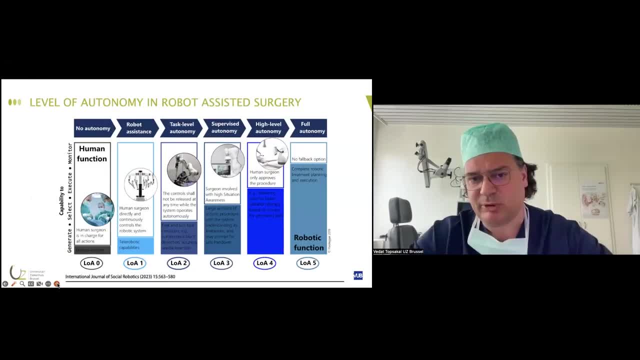 It may even facilitate a leap from, let's say, in terms of level A3 autonomy, where the surgeon segments And supervises the trajectory, that AutoPlan now is at level A4 of high-level autonomy, where surgeons only approve the trajectory. 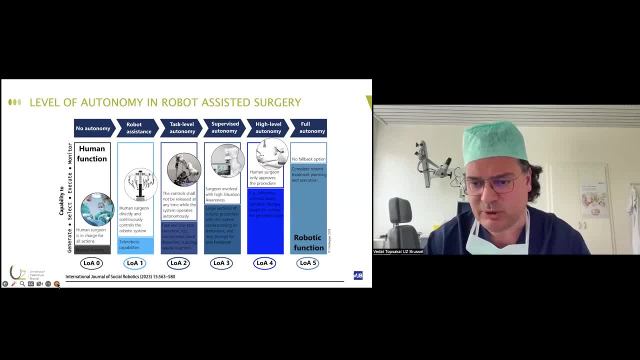 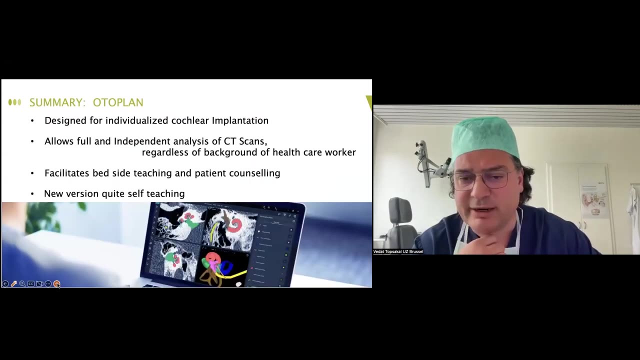 And I'm sure Professor Cavazzaccio is going to tell you about what is a safe trajectory. but I just want to point out that AutoPlan, with the latest version and the automated algorithm, is just another step forward to standardize higher care or a higher level. 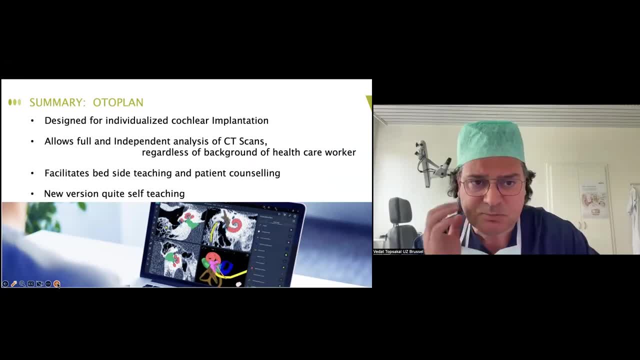 of care To standardize also our outcomes. So to summarize, it really is a tool to provide you with parameters for individualized, custom-made, tailor cochlear implantation for your patients. Next to that- also Nicola nicely pointed out- it's also good for counseling pre- and post-operatively. 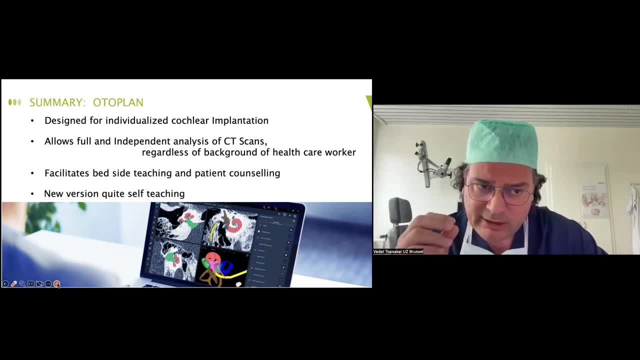 but it's also good for teaching for your residents. It allows a fully independent analysis of CT scans regardless of the background of the healthcare workers, So an anatomist can upload easily the images and come back with a plan for anatomy-based fitting. The new version is actually quite fun and quite self-teaching. 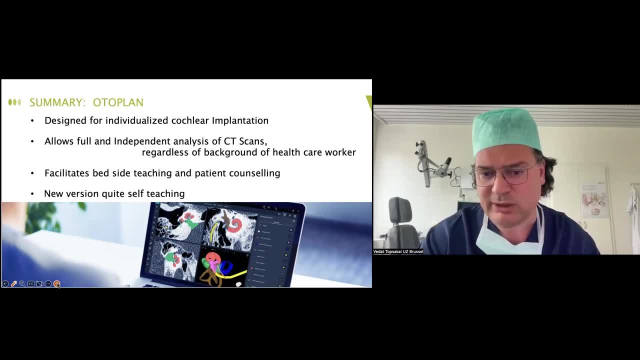 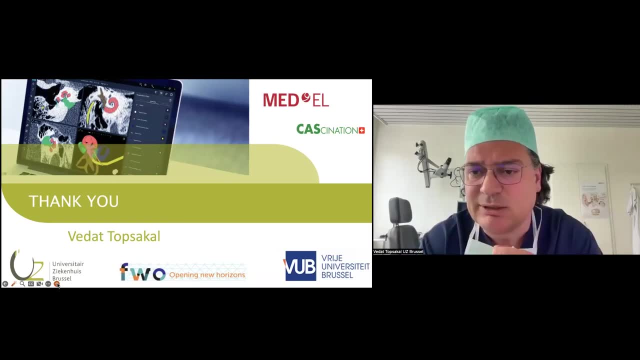 This was, in a very short amount of time, What I could share with you. I would like to thank you again for your invitation and show you my disclosures, and thank Madeleine. Thank you very much, Nicola. Thank you so much, Professor Topsagal, for this comprehensive presentation. 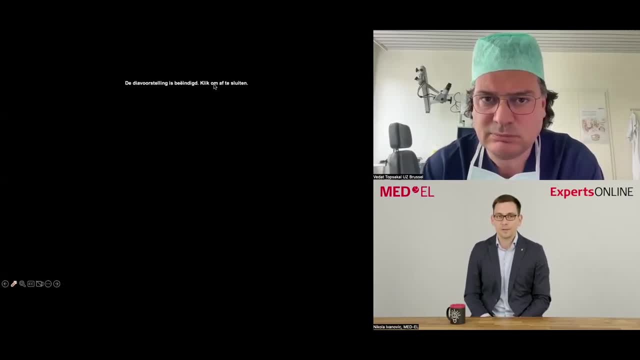 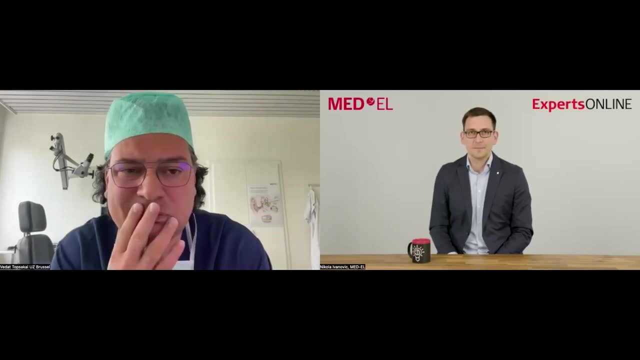 Thank you. Thank you for your presentation, not just only on autoplan, but the journey through the whole topic of robotics and your experience with it, Highly appreciated. I guess- I don't know, we don't have any questions yet, but at the end of the session I'm sure. 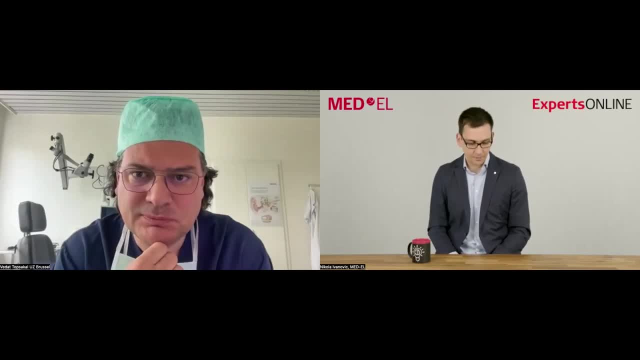 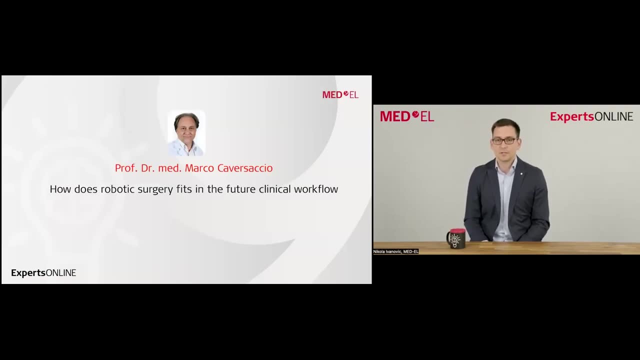 we'll have some and we can answer them. Thank you, Thank you again. Let's switch to our next expert, Professor Marco Cavasaccio. Thank you, Thank you, Thank you, Nicola, Thank you, Professor, and thank also for today's presentation. 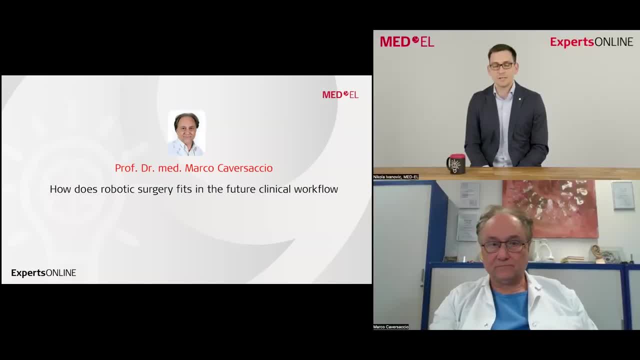 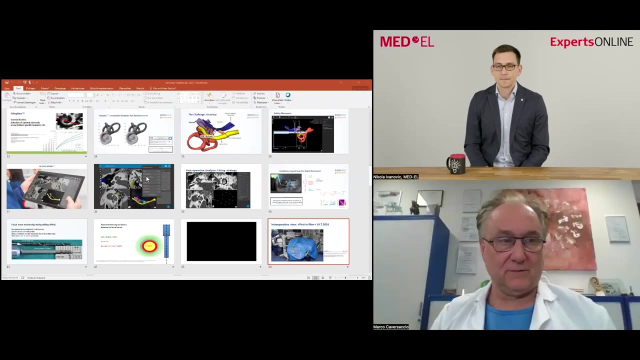 Thank you also to all the panelists who will, I'm sure, extend what Professor Topsagal already mentioned and give us some more insights into how our robotic surgery fits in the current and future clinical workflow. Professor Cavasaccio, please. Thank you very much, Nicola. 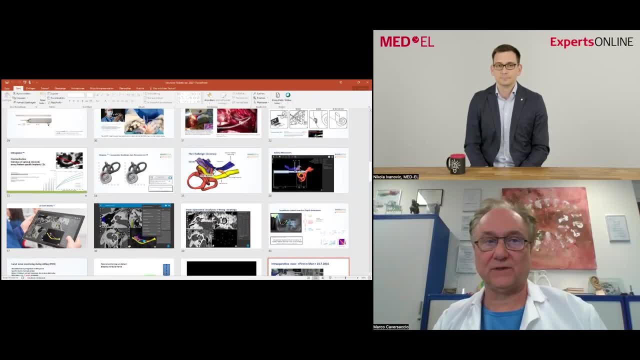 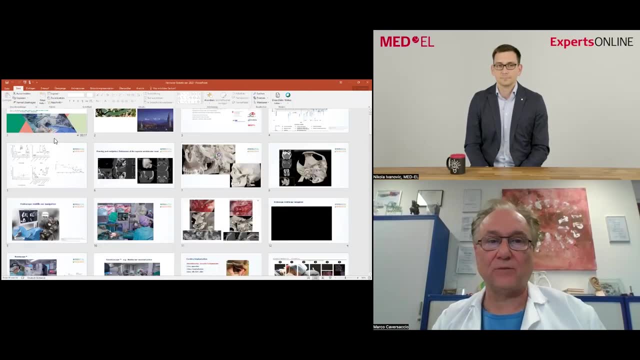 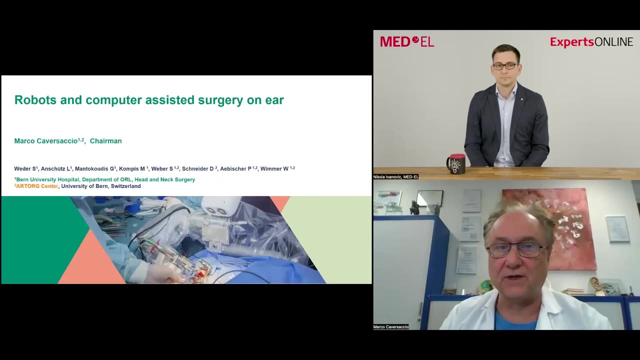 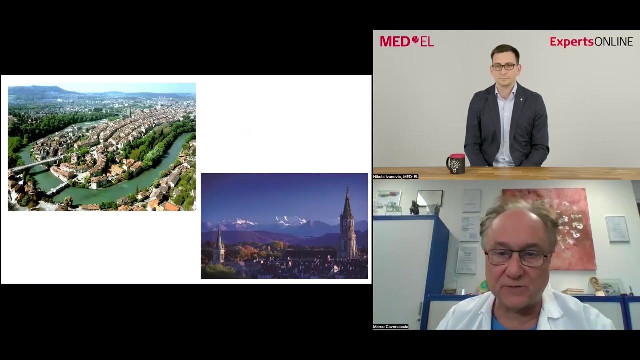 Thank you, Professor Topsagal. We will start. I have moved here a little bit. Okay, my topic is this afternoon is, it's a little- the robot and especially the computer assisted ear surgery. I start with computer assisted surgery. First of all. I'm from Bern, from Switzerland. we have disclosure and acknowledgement that 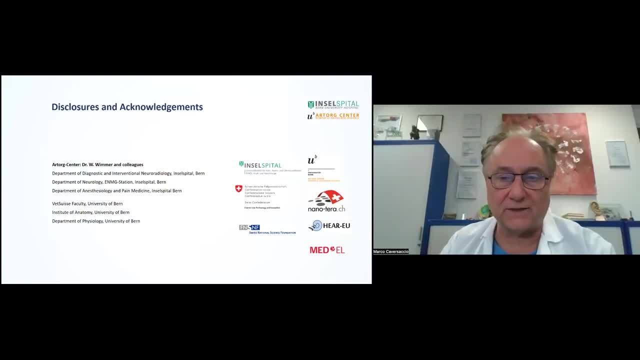 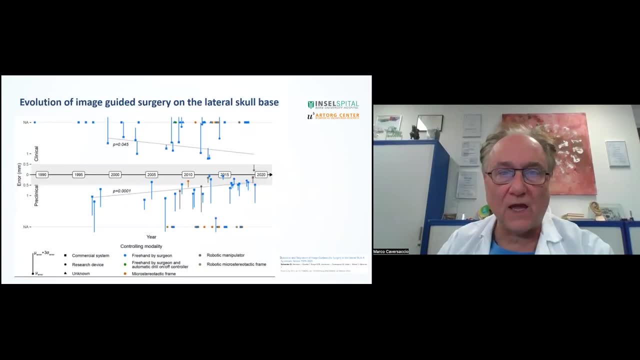 you can read on the right side: supported by different institution from Switzerland, from European Union as well from Medell. When you look about the evolution of image guided surgery, you can look about, especially on the lateral skull base, that often they are not very often used because we have is. 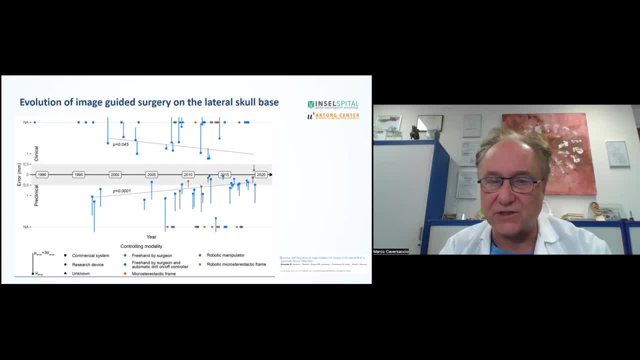 a delicate structure and we have not a high precision on this image guided surgery. One of the first about navigation surgery was in Freiburg, in Breisgau. where they have started to use it For cochlear implantation is then more than 15 years ago. why we have this? not too much. 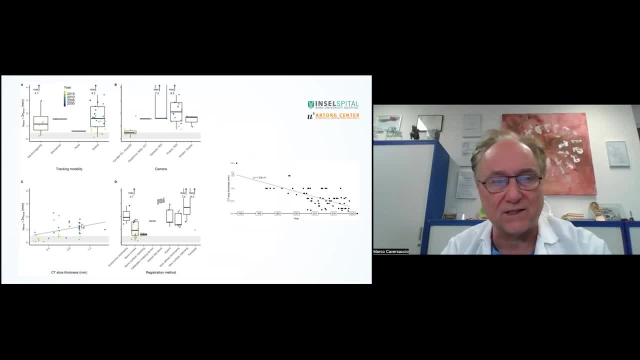 use image guided surgery on the lateral skull base. it depends a little bit on the tracking modality on the different camera that you can see. what we have at the moment is this: come vr be one is this. this one is access 3d. where is really low open one millimeter? 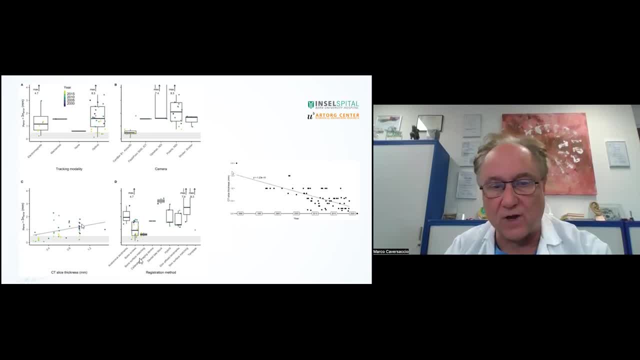 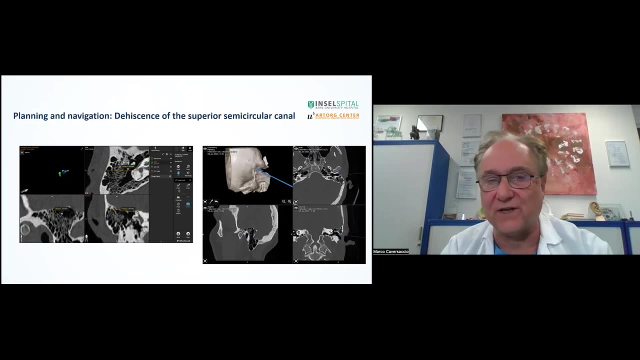 we have this, Cities like The thickness, was these nowhere better? and the different registration modes, methods, as you can see, and we have a high precision, high accuracy, especially when you have bone screws. When you look about what we have today, we have on the microscope, you have the possibility. 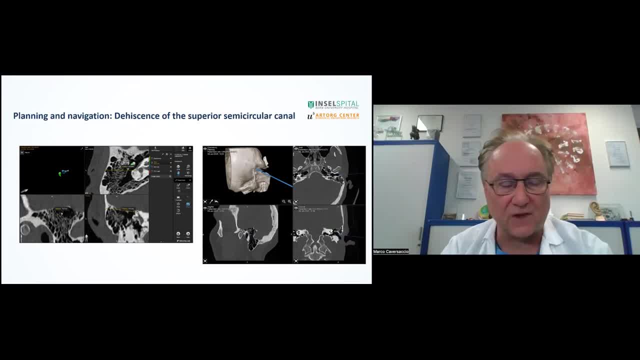 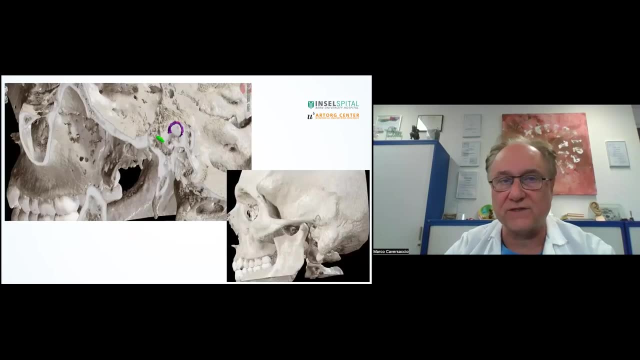 to make an injection in one of this- What I mean in the, in inside the imaging, and you can visualize Not only The CT scan, but you can also look about segmentation, what you have performed before, what you see here is one of the situation. 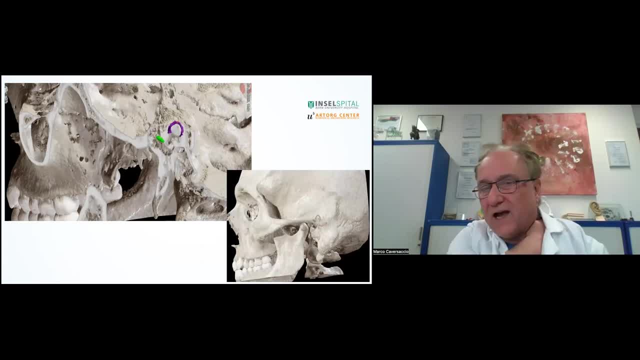 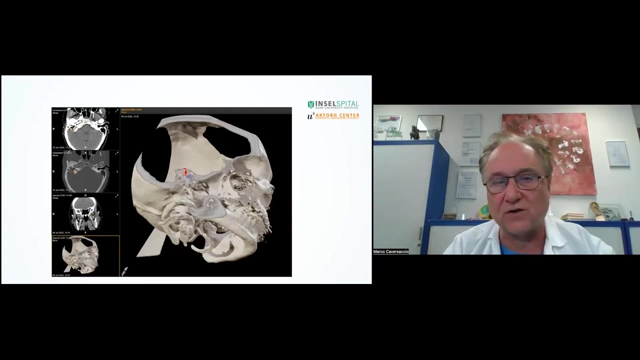 Technology of the brain, that system that you can see. you can show here at the essence of the superior canal. you can also make a plan, a plan on the different obstacle visible here in green. and, to look around, in 3d, reconstruction of the head is what you find at the moment. 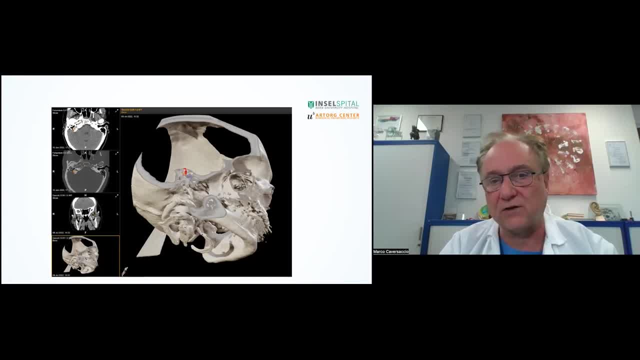 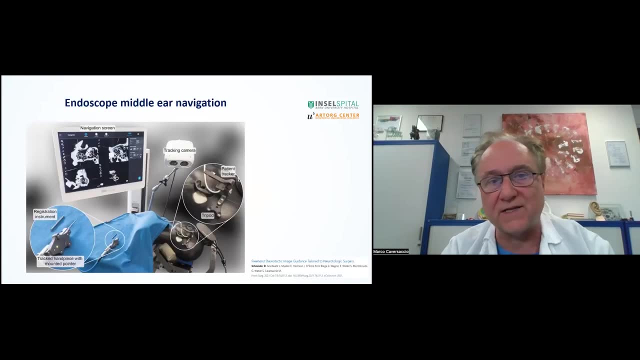 you can see And you can also see. you can also make a fusion of CTMR and the segmentation technology that you can use inside the microscope for navigation on the lateral skull base. Another possibility is, in fact they also the last 1015 years to make endoscope middle ear. 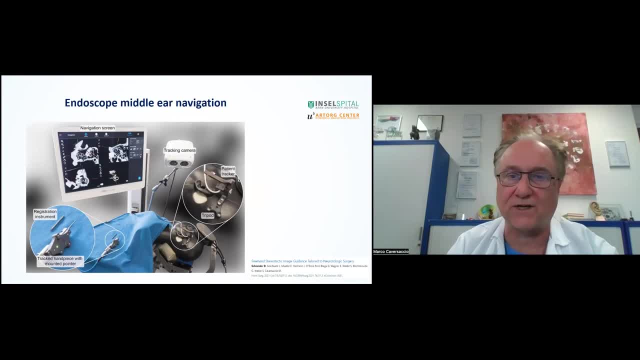 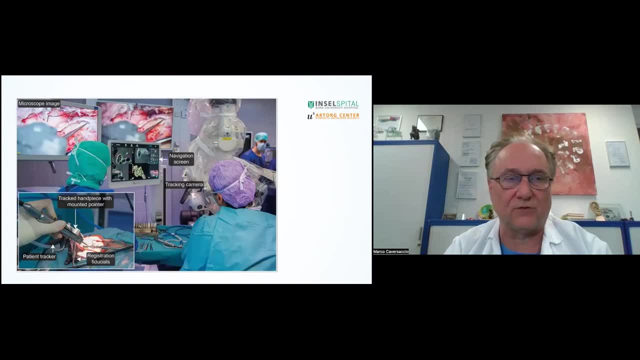 navigation. you have started with this one. if you're tracking camera, patient tracker is like a satellite They share and to use it for some experiments during surgery, that you can visualize this not only on the microscope but also in the endoscope and on the monitor. 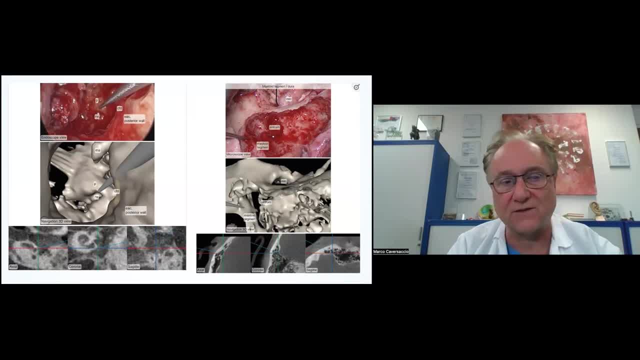 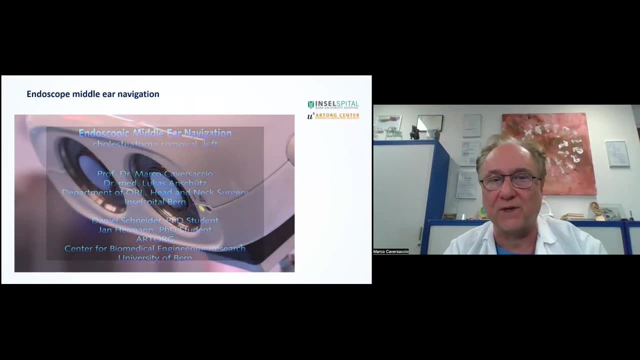 Here you can see the different possibilities to visualize on 3d, on the CT scan, the exact position of the middle ear, the promontory on the round window, on the court, that company and so on. And I Quickly show you this on a video: the endoscopic middle ear navigation. or do you have performed? 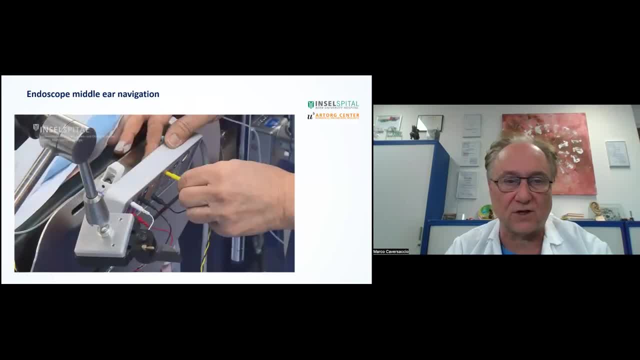 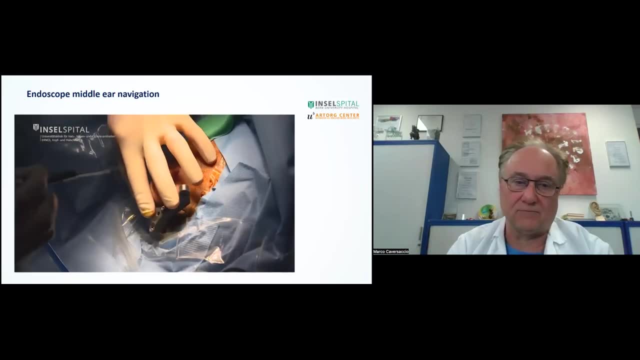 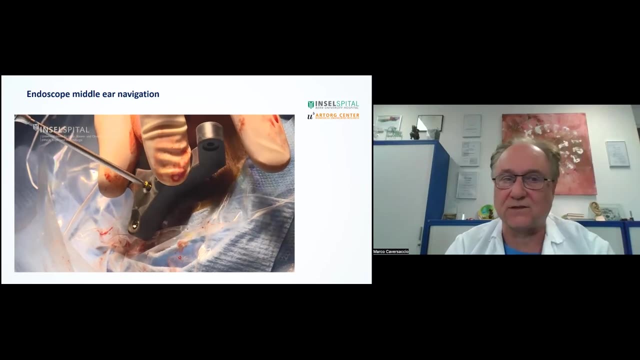 together with our coworker, Professor Lucas, answers here in burn to look about what is also possible- because the topic is here During this session- is also robot, not only robotic surgery but also computer aided surgery, because computer aided surgeries and since 1996 is also possible to make a computer aided 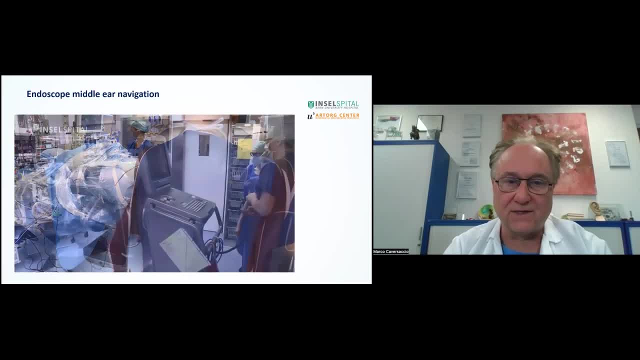 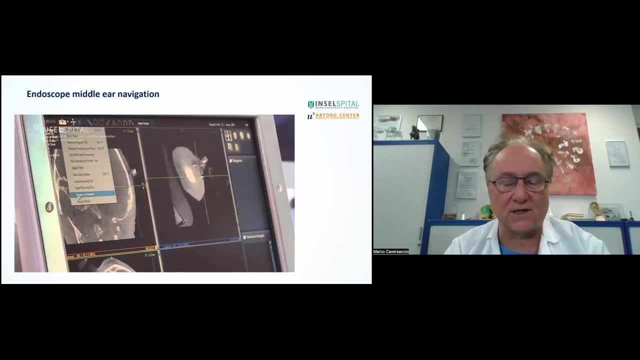 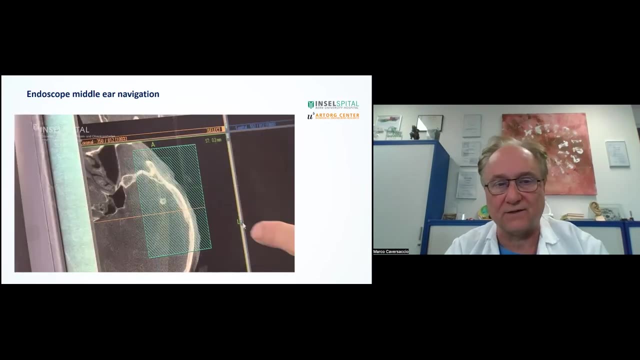 surgery. So we're going to talk a little bit more about the endoscopic surgery. on endoscopic surgery, It's great. We have already seen by Professor I better topsock color interoperative imaging, the cat that you can see it here, And what is necessary. what you have seen just before is a satellite dish, in fact, or a dynamic. 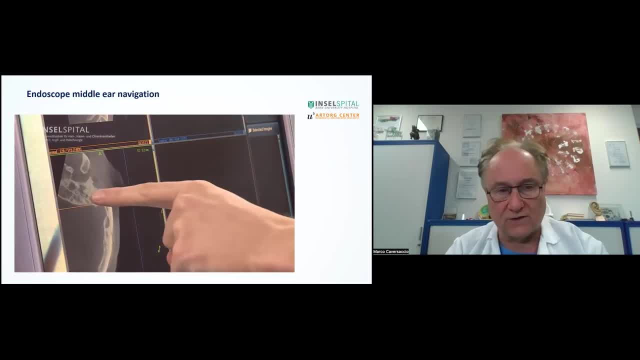 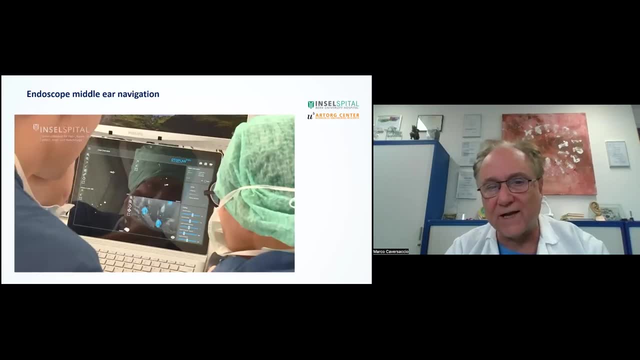 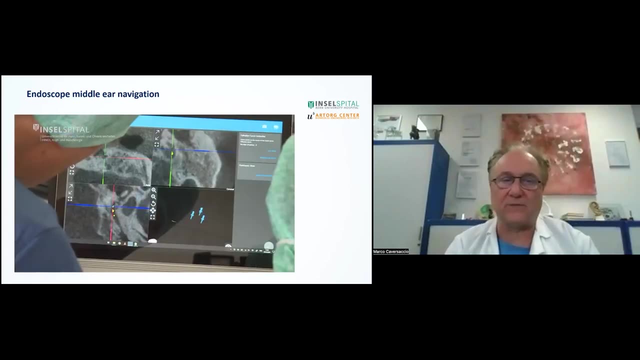 reference base And here is the data you can hear. you can make them that the segmentation to visualize on this auto plan. Okay, We have also an ultrasound system. This is the elder version, is not the newest one. 4.0 here, especially for the fashion or 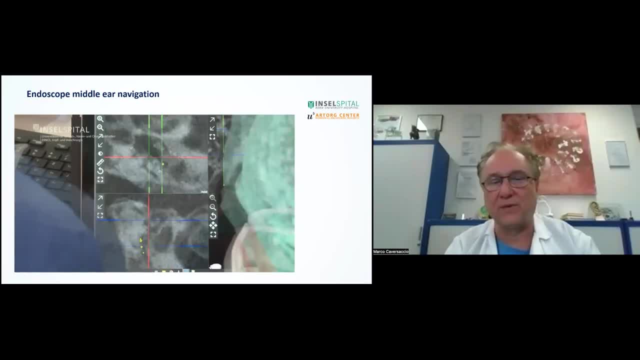 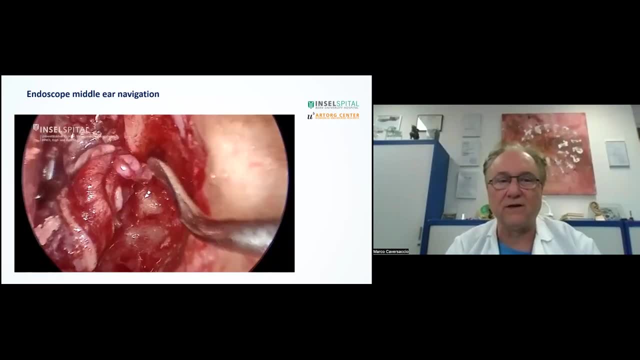 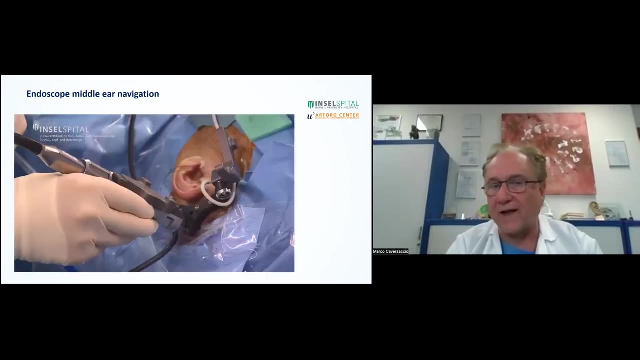 for to visualize here in yellow, visible if you perform this with your medical engineers is also important as well. me for radiologist here. this is only to visualize. this is colostomy surgery and the topic surgery. These are new ideas, what we have for the future to integrate and navigation. 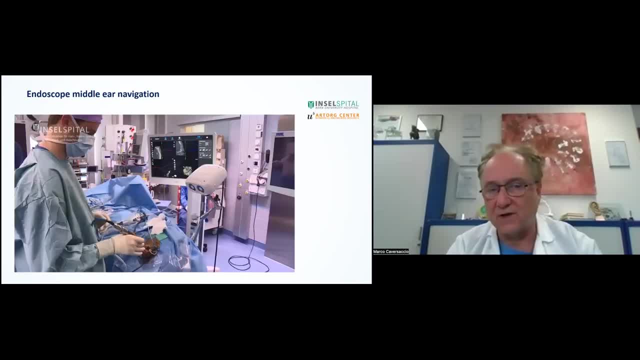 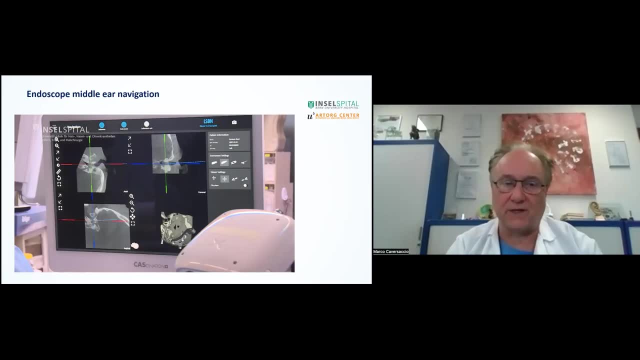 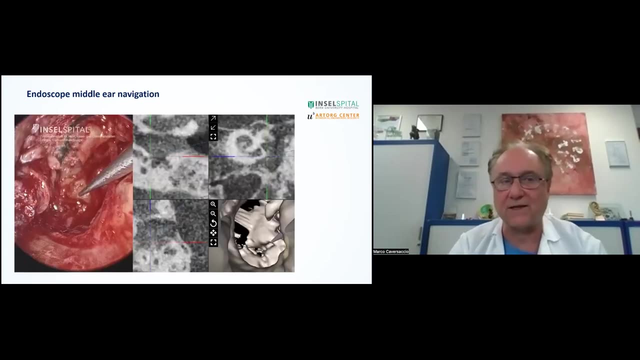 clear. what is important is also that you have at the tip is perhaps 0.5 millimeters, especially the registration technology that you have seen in the beginning, that the best thing is to do this on screws, and here you can then visualize on one monitor where you are exactly. this is for middle. 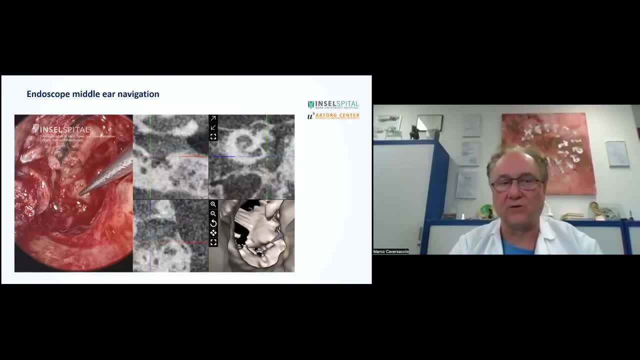 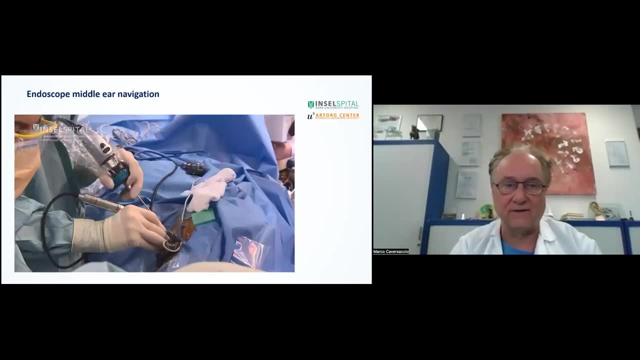 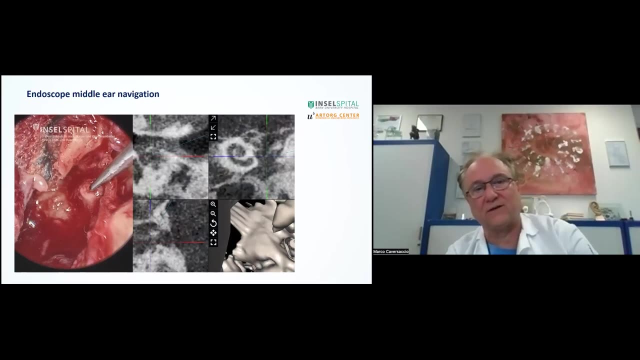 ear surgery round window approach that you can see it here here. the different structure is also visualized here on 3d on the right side and it's clear. you can do endoscopic surgery with a drill. here is the star base ahead that you can visualize on this screen. these are the different possibilities. 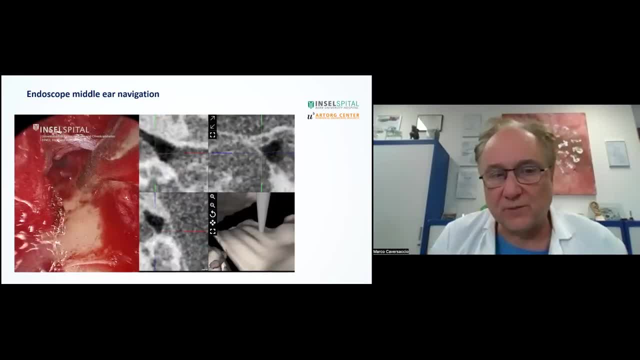 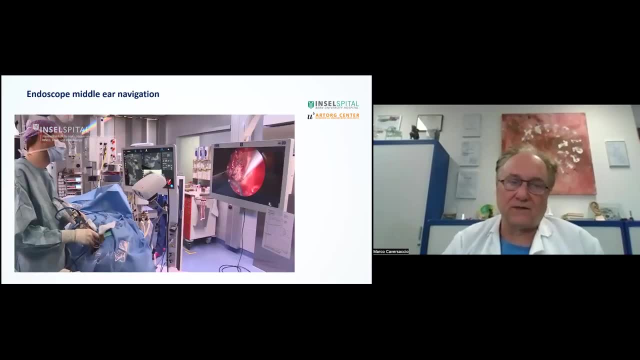 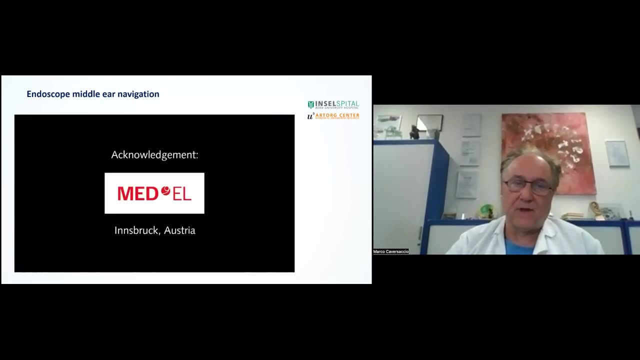 that also in the future, not only in microscopy, can make a navigation surgery. it's also the possibility to make endoscopically. it's clear not, uh, these are prototypes and there's not world wide you can see something like this. another thing is, what is also a little bit in its 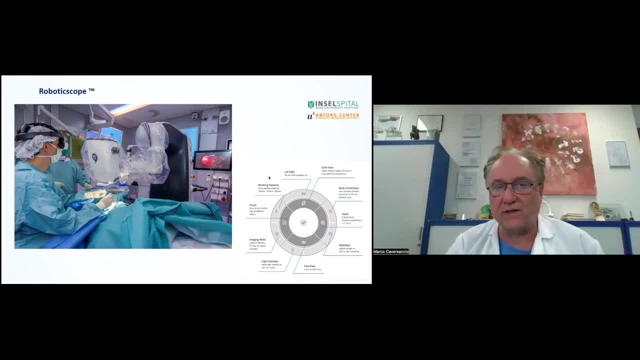 progress. this robotic scope, this is a paradigm change that you can move a little bit your camera, you can make imaging mode focus preview. this is another possibility of robotic surgery where we enter now in the details in the next 15 minutes. this is a one possibility, not only using for a. 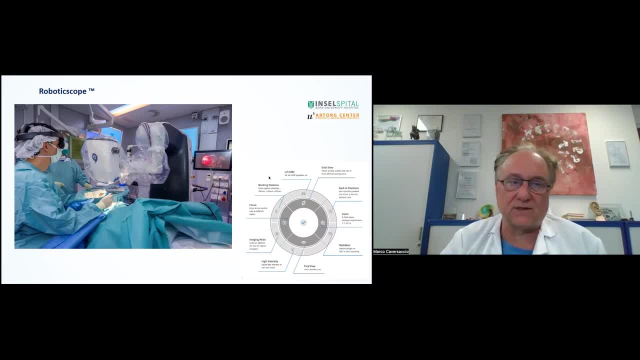 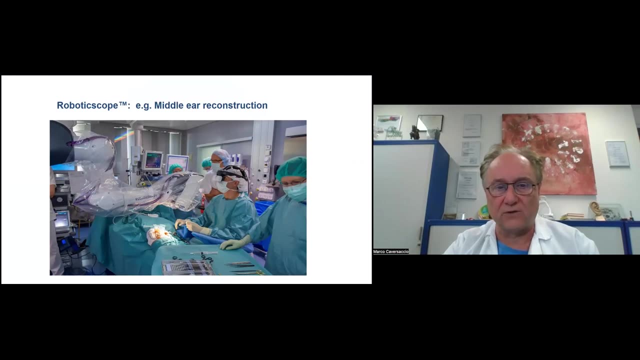 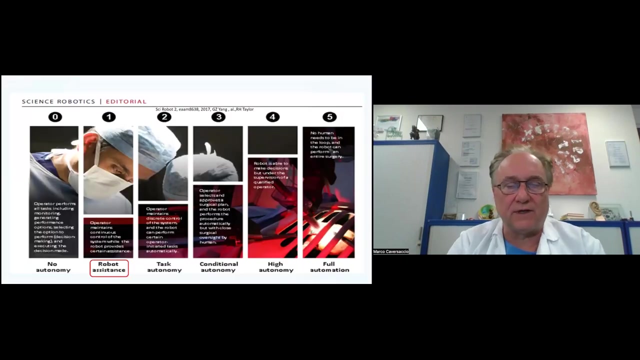 surgery, but as well for moving system, like here, the the robotic scope. it's also possible today to make on the exoscope surgery. here you can. we show you where we perform this on middle ear surgery with this robotic scope. now move to the robotic surgery and you have seen one of the last slide. 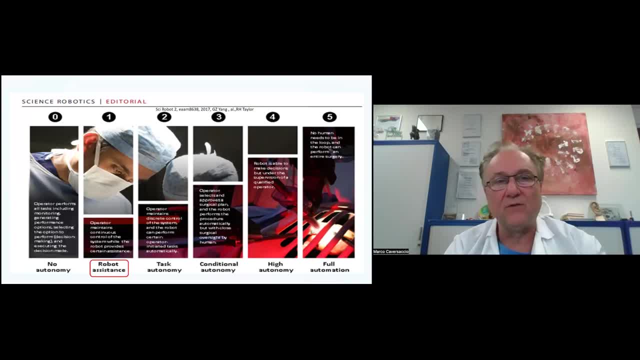 from professor veda popsakal is a bit the same where we are speaking what. what we do normally for robot we are often and what is accepted worldwide is a little bit robot assistance and what we perform at the moment is a certain task: autonomy. what i will show you with the hero: 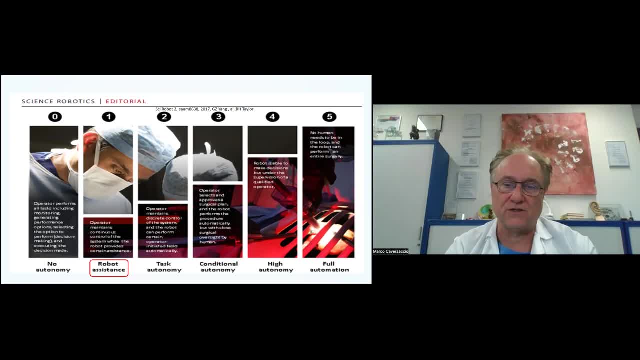 system. it's clearly the market. you have also davinci that you use more in the ent area, especially for the course that's our robotic surgery, for, in fact, for the base of the tongue or something like a far injector- me, you can perform this, uh, with uh da vinci, but they especially for the skull base. 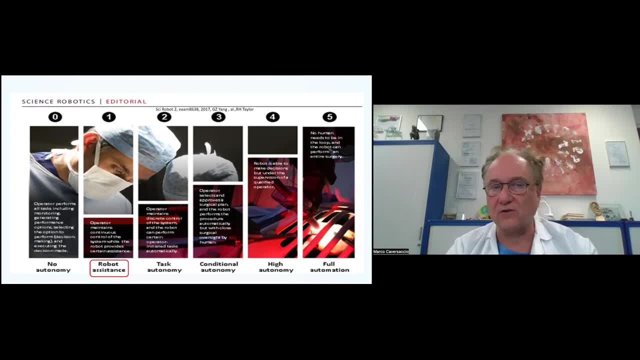 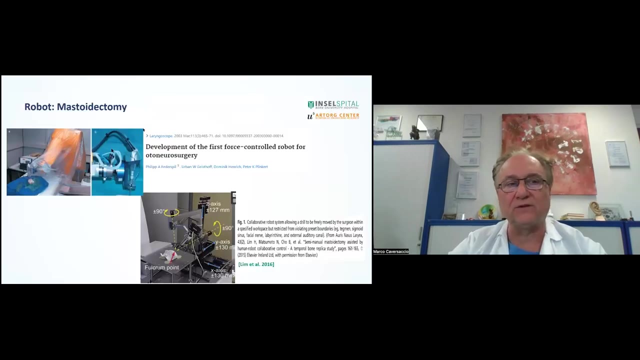 as well for uh the ear surgery. we cannot use this davinci system, but what we do is to perform this robot assistance with a certain task autonomy. this is uh. level two is uh. this was proposition is in fact uh, uh from 90s, uh, 2017. uh is from russell taylor. when we look about the robot system, 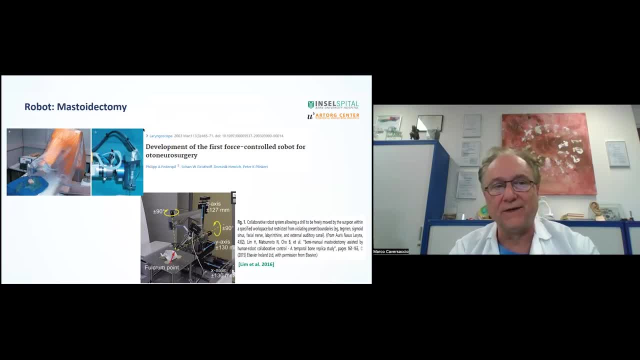 when you perform a surgery for cochlear implantation. the question is if you make a tunnel procedure, keyhole procedure or we do it like for machined, a cat cam technique, computer assisted design to make a mastodectomy, and what we see there are. other groups worldwide have started to look about controlled robotic, only for 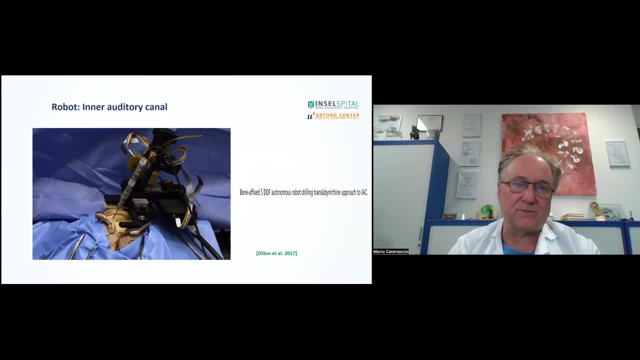 mastoidectomy and also possible, but only is remaining still at a certain cadaver level- is to the inner auditory canal for small acoustic neuroma surgery. but until now we have no robot that can be used in clinics. when we look about now what is important, what was already mentioned, 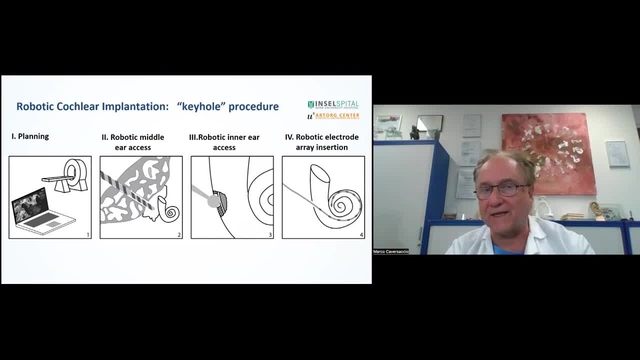 by professor topsakal. it's very important the planning system, because without planning you can perform nothing. it's the same when you use tesla, when you have chatbot, when you like. now big data management, artificial intelligence, et cetera is all going in the software, but this need time and this need also. 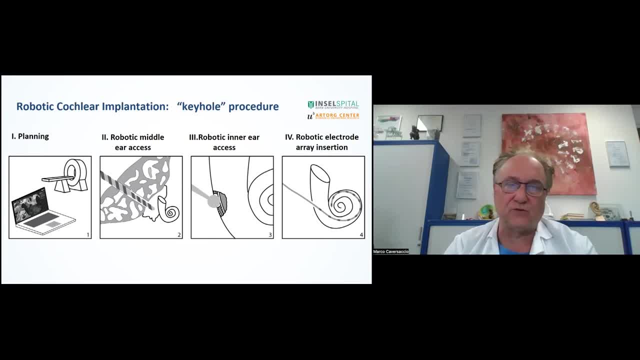 that you you looking a little bit, what can offer you the system? then, the robotic middle ear access, the inner ear access and what is important, especially when you hear. for the step four, the robotic inner ear access is for hearing preservation, and i will show you here a little bit. 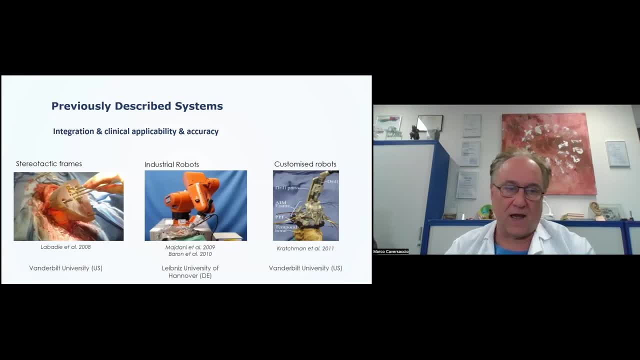 what is already on the different market. uh, one of the first was professor lover from the vanderbilt university, who have started 2008 eight, then watching the industrial robot with much tani and uh crutchman take over from the us to the hanover school. la patty rob has performed. 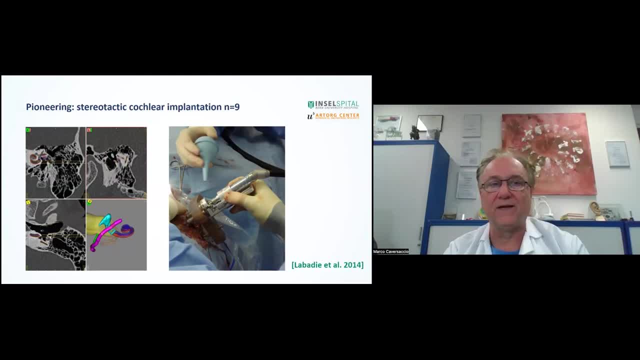 2014 and presented laryngoscope and nine cases. what we have, what he has performed with the stereotactic uh system or you can use uh, see it. they've also used a planning system. it's two to two here to plan this. This was one of this procedure. Again, it's a keyhole procedure. It's important. 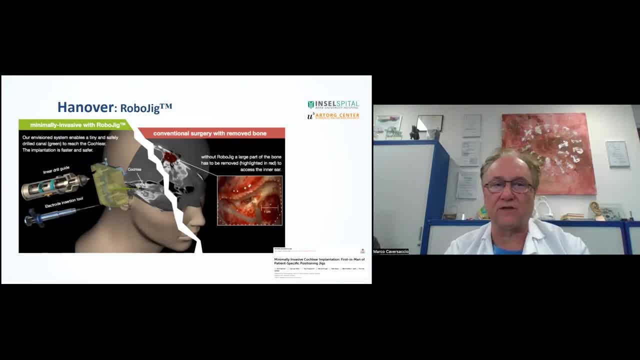 The Hannover group have made also a different cadaver study with this robot chick. It's a little bit- yeah, it resembles a little bit what was performed in the US and they have also made some publication at the moment, but they have not used it completely in human. 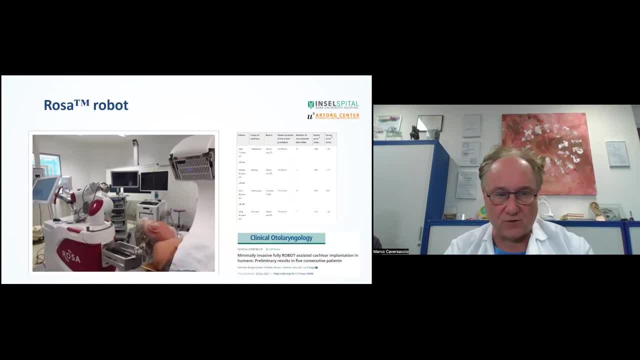 surgery. Another system is the ROSA robot system, One that is used often for neurosurgery, and they have made five cases. Unfortunately, like also the group in the US, they have had the problem with the facial nerve, and in this program they have stopped it. On the other, 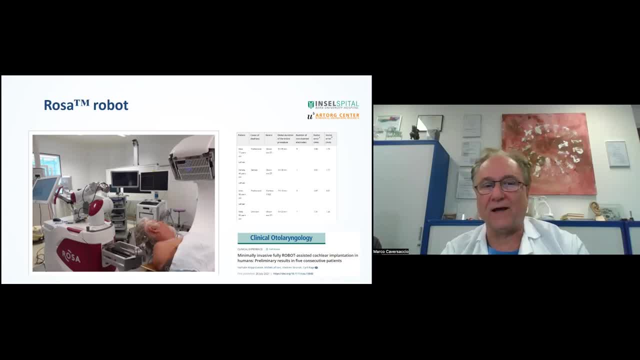 one on the US. what they have had is more a high-speed drill And the high-speed drill. they have not touched the nerve, but what they have performed is the high. the heat has damaged the facial nerve, but transitory, what I know from the US. But in this case, 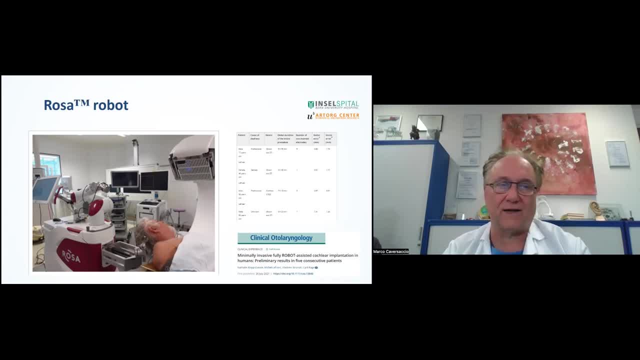 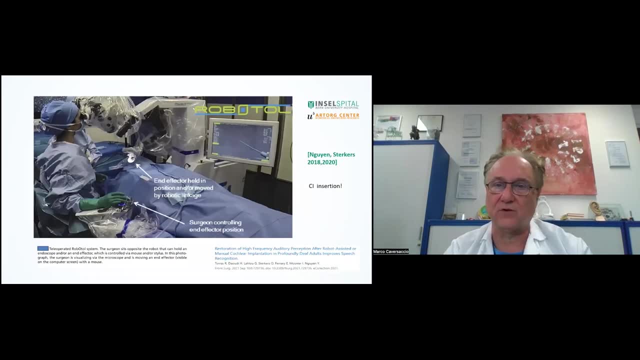 they have reached, in fact, the facial nerve, and therefore it's very important to have a high precision for the robot system. There exists another one. It's this robot from France, from NBN, and especially from Oliver Sterker, where this machine can perform. 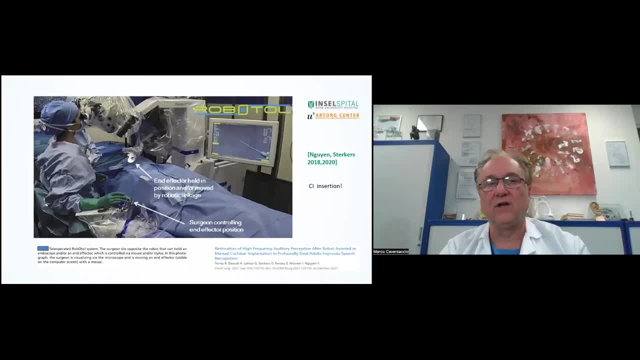 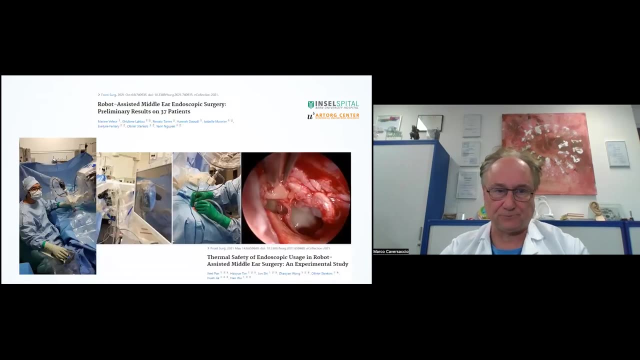 Different things. You can use it as endoscope holder. You can make laser surgery of stop as surgery, but you can also use it for introduction of the electrode inside the cochlea, especially when you have cases with hearing preservation. And here you see also the possibility or used. 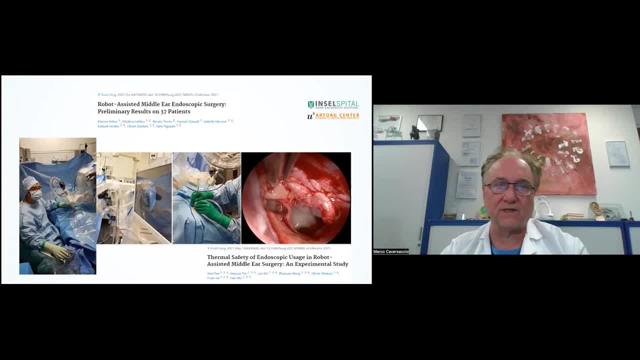 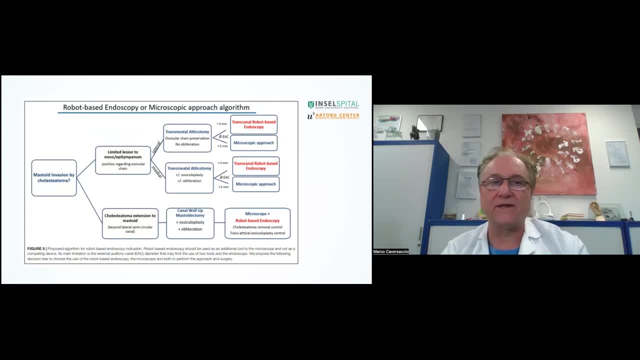 by a young gun to use it for middle ear surgery. but they can also use it not only for middle ear surgery but then also for cochlear implantation, And he has made also a proposition to use it when. to use it for transcranial robot-based endoscopy, when it not worse if transmittal. 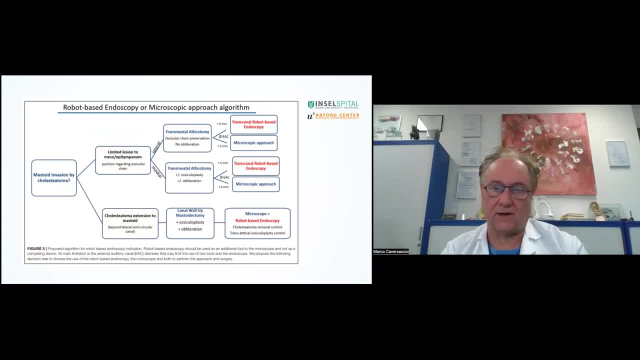 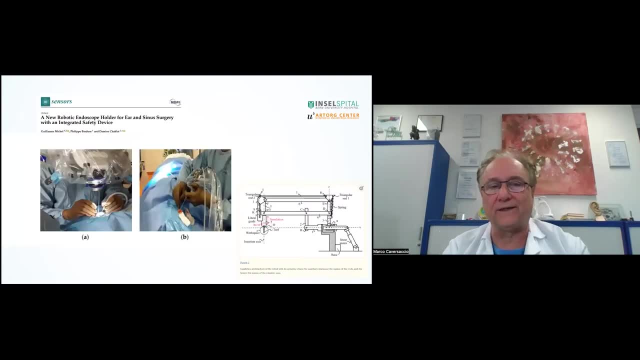 normal at dichotomy and in microscope robot-based endoscopy. When you have looked about the holder, especially when you will now use it for the future of for endoscopic surgery and this we perform a lot of hybrid technology also here in Bern. 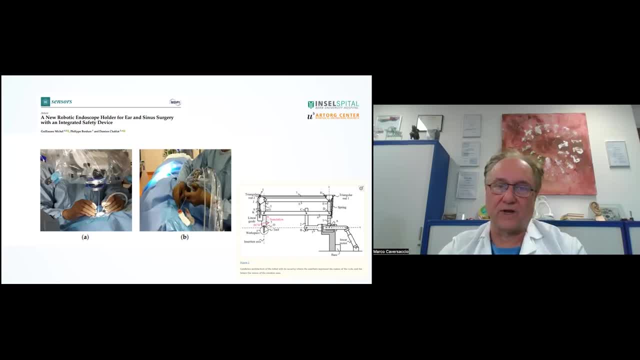 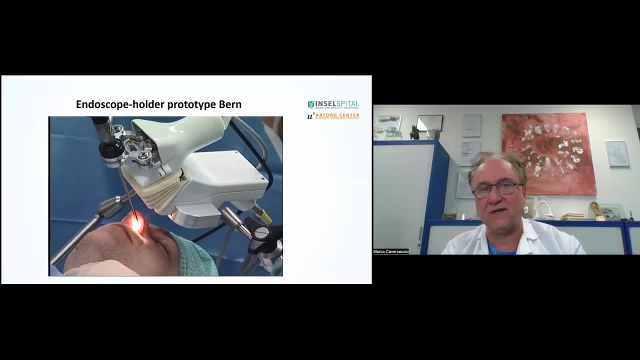 it's clear you will find more and more new prototype for endoscope holder, And we have also looked about endoscope holder also in Bern- not only for the nose- what you can see here is also the one of this prototype- but you can also use it not only on the nose. 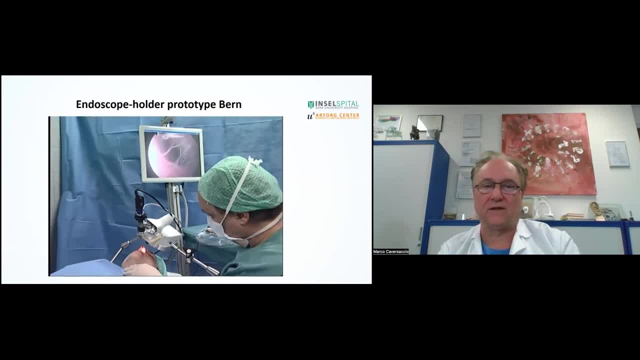 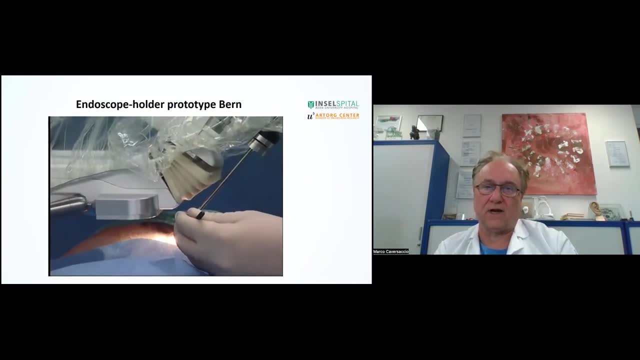 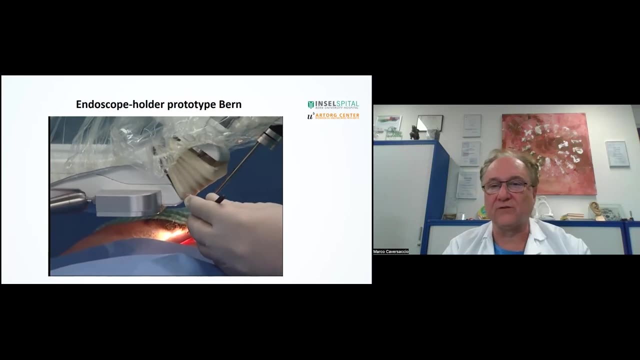 but also on the ear And here then you can move it. This is also only a head holder. Here is the ear and you can use it. The only problem, what we have is that he's four millimetres or three millimetres and we have not enough. 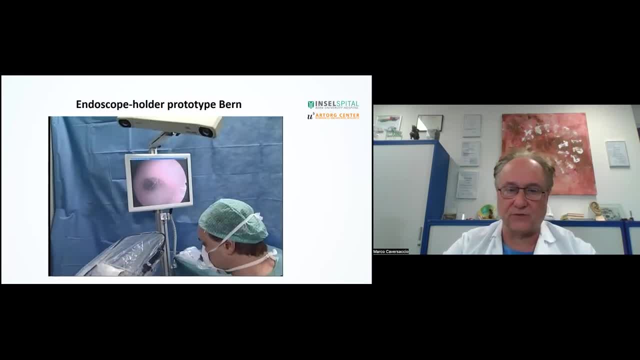 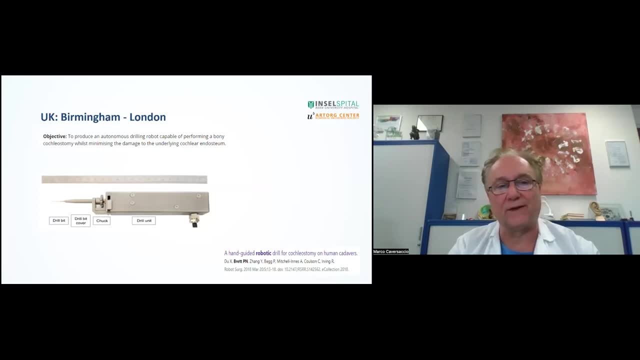 place, But it could be also helpful for the future When we go now back to the cochlear implantation. what we can look about is a different group worldwide. One was also for the UK in the Birmingham hospital, Birmingham and London technology, where Peter Brett has looked about to drill for the cochlea. 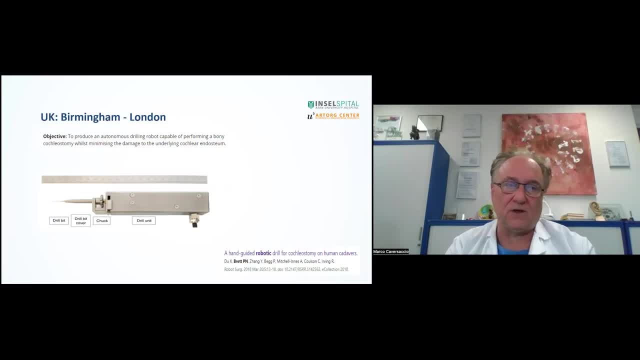 stomie on human caudaris, Cochlea stomie or what we want is to have for hearing preservation round window approach. But this is very important. One of these group also in Birmingham. they have looked about also for robotic cochlear implantation. 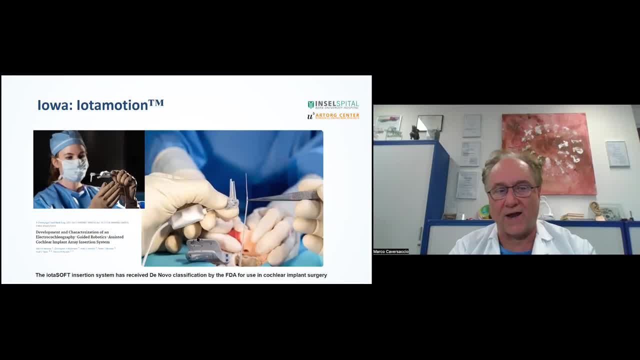 Now, another philosophy is only from the US. It is. It is Hansen and especially Bruce guns in Iowa. They named this also I jota, I jota or Iowa motion. They concentrate them only on the last step. We have had four steps, and one was for hearing preservation. 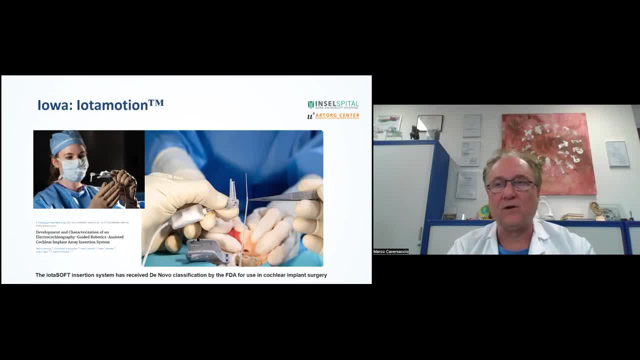 They use this technology to put in with 0.1 millimetre per second to 0.3 millimetre per second to put in the electrode in still hearing person, And I think this is could be one possibility to concentrate all of this robot on the last. 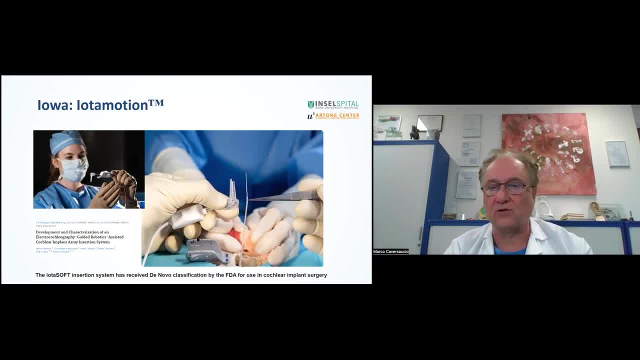 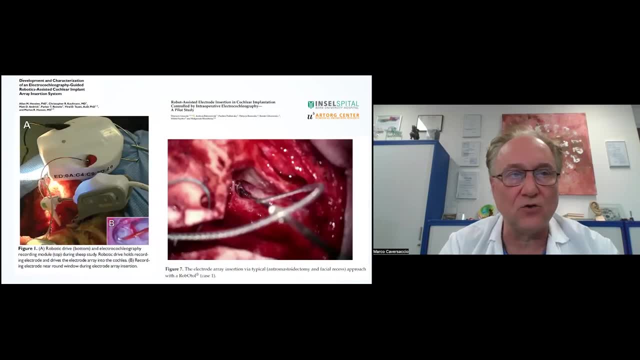 step And, what is also important, that not only this group have looked about this, but what is also possible in the future is to look to put in electro cochlea graphy together with this robotic assist machine or array, And this could, Especially for normal anatomy, could be helpful and is especially for hearing preservation. 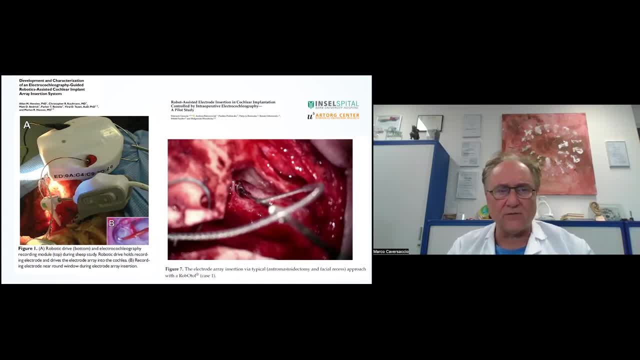 technology And you see here one of our head. but they have also started what I had noticed from the US also on the clinical side. There is another group in Poland that have used this only for cochlear implantation, for still hearing preservation technology with the robot. all in Poland, but you can see on. 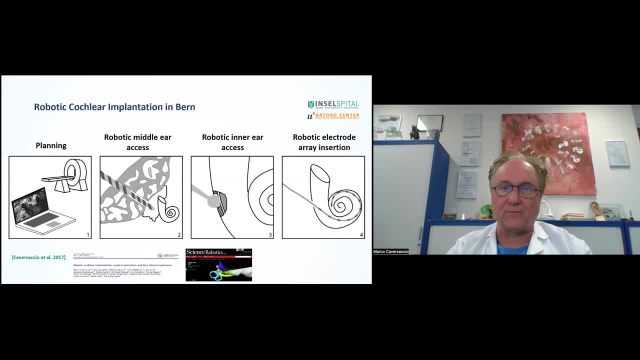 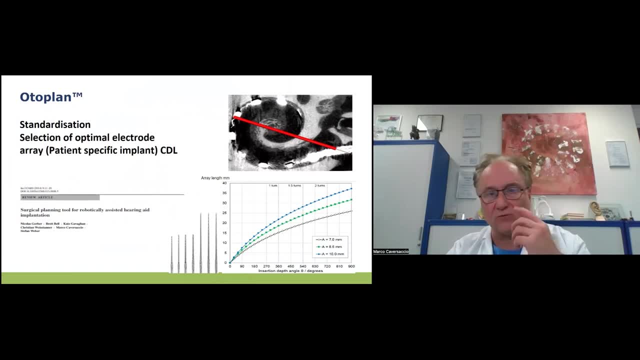 the right side. Now go back a little bit what we have performed: the auto plan: you have already heard. This is really the basic. when we don't make a plan system, forget it, don't make nothing, but is sometimes it's time consuming and it, but it gives you some standardization selection. 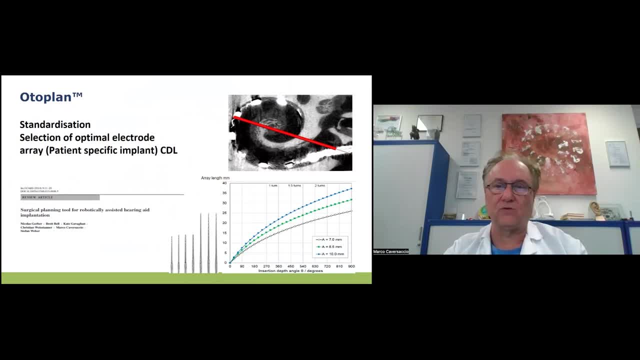 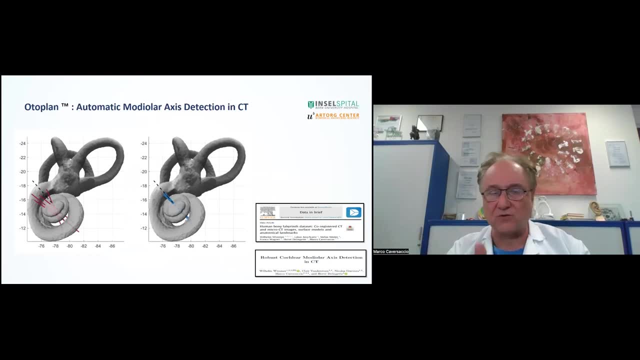 of optimal electrode, And especially you have then the different possibility to measure here to conducting duct length. Another possibility is also we have semi automatic segmentation. This mean you have some interference by a medical engineer, but what you have seen is also possible to make a complete automatic one. but again, but it also must be an error. 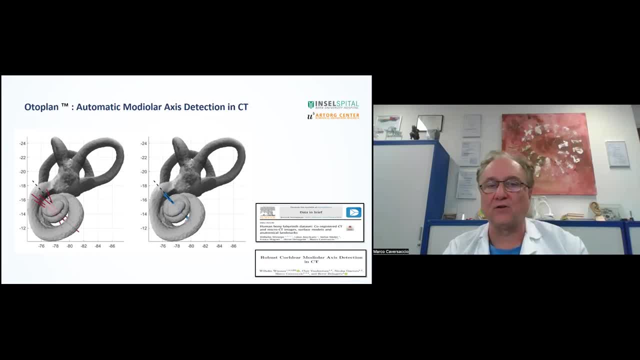 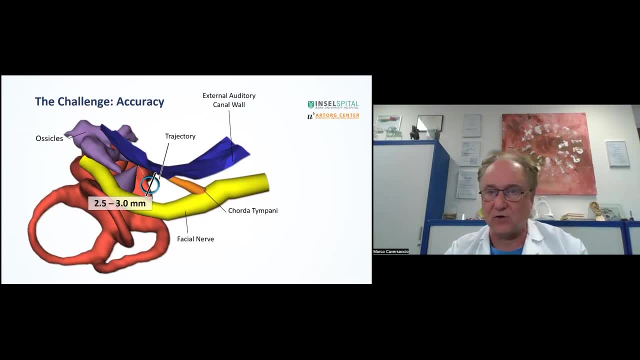 inside. Someone was know what kind of algorithms are inside. It's clear one of the challenges this accuracy and especially when you make this keyhole procedure- what is performed with the robot or what is performed with the, with the Yota motion- You have to make sure that you have a complete and normal mastoidectomy and they don't go. 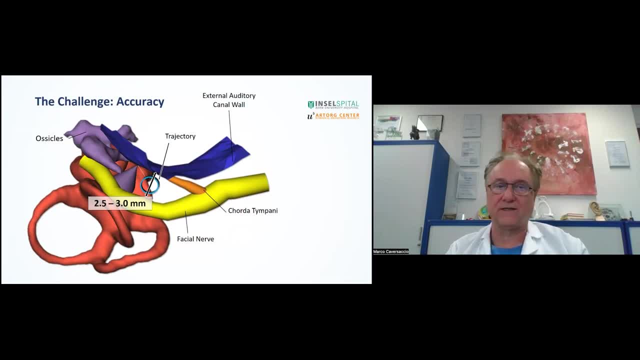 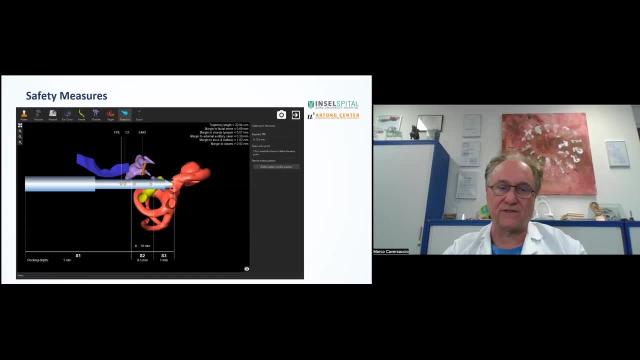 through this challenge, this special quarter recess, And in this case we have about 2.5 to 3 millimeter, and is cleared during the search. You have these different steps: that one to the posterior tympani, Tommy, step two, then you go through it. 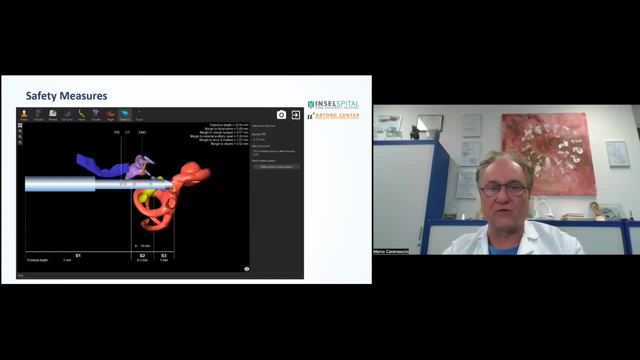 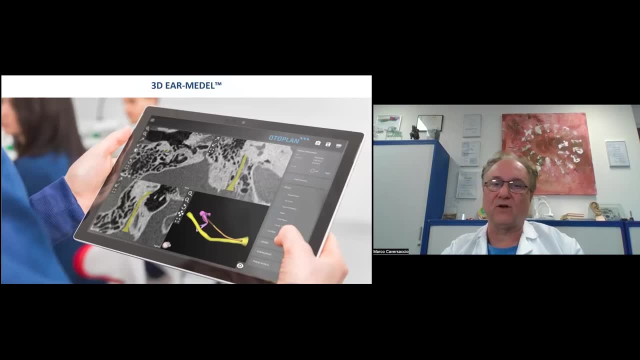 And step three, you will touch them, the endoster. and step four is the insertion. what also the other group in, specially for hearing preservation We perform all the plan you have already heard about by Professor top soccer is very important to look about this. What I can only say is the quarter tympani you cannot every time visualize on the CT. 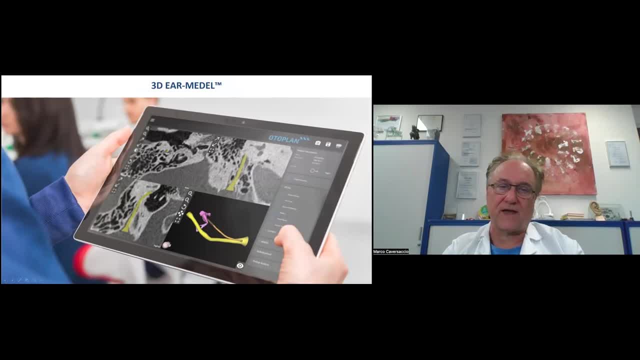 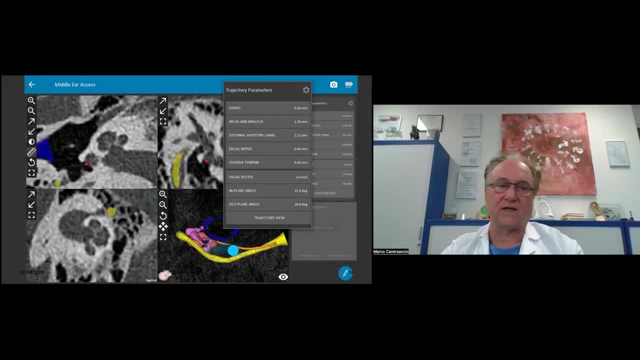 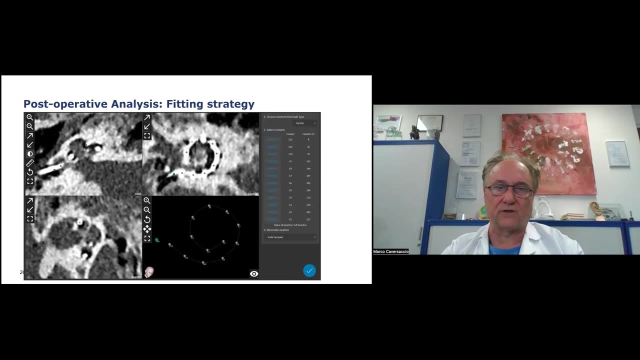 you make an extra, extra relation in fact to go through, because sometimes it's not visible, also to see it on the CT scan and it's clear. here you can make all the calculation to the fashion of this distance, Especially to have a good trajectory and optimize, and is clear, what we have already. 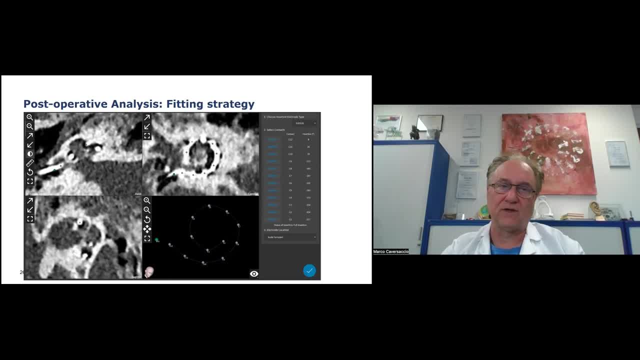 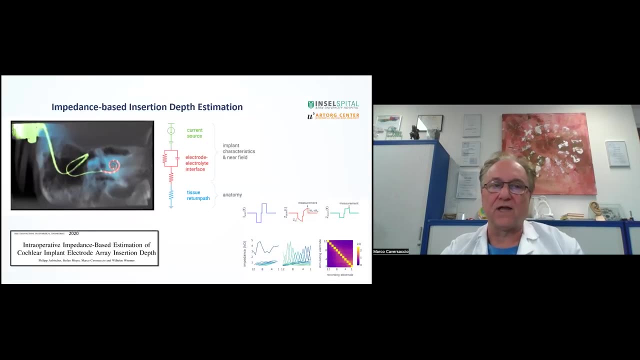 seen is the fitting strategy postoperatively to have a look about this, to see where are the different platines to a stimulation of this 12 electrodes, what you can see here on the right side, because also, perhaps also in the future, it perhaps you can replace. 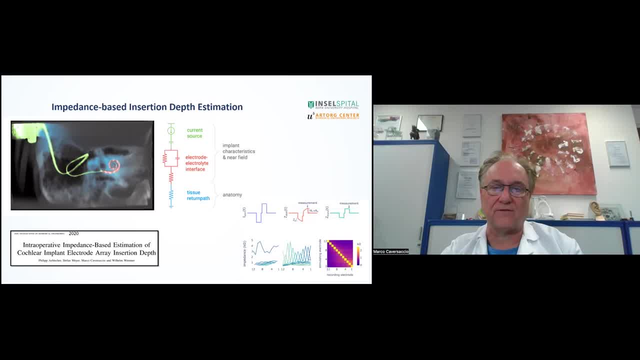 it to the CT scan if this impedance based insertion depth estimation. but we will see it in the future if it's possible to exclude the CT scan postoperatively. Here is the drill bit: where we go through is 1.8 millimeters. 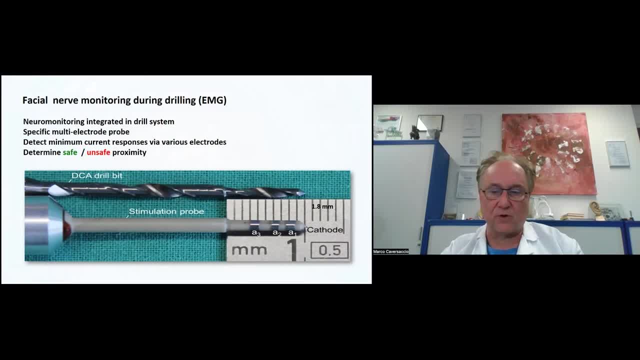 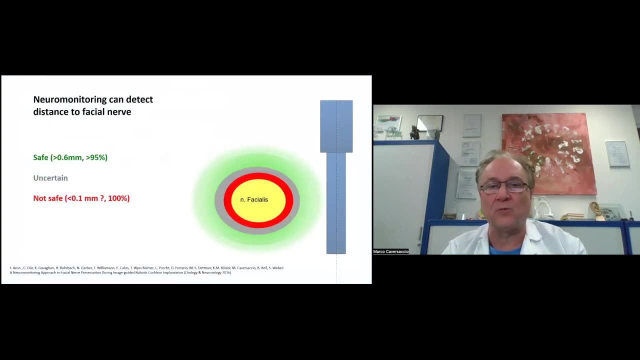 And what we have also is the probe. This is the facial nerve monitoring in the keyhole procedure. we cannot use a Norman nerve integrating monitoring. what is what is coming from other companies? The question is over there at the normal thing: what is safe? 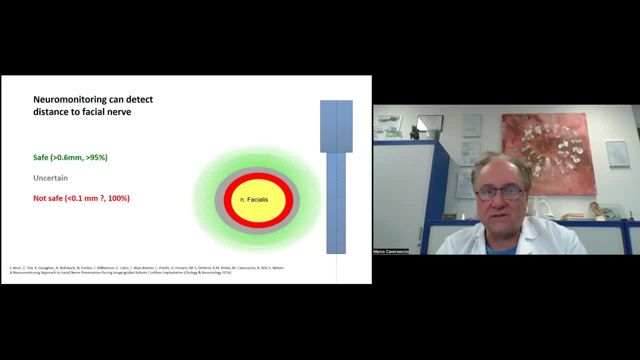 What is not safe, need to face nerve. We know that this is more than open six is 95% not safe history. open one millimeter. The question is open three. open four is enough. It depends a little bit. What I told you was on the electricity on the bone. 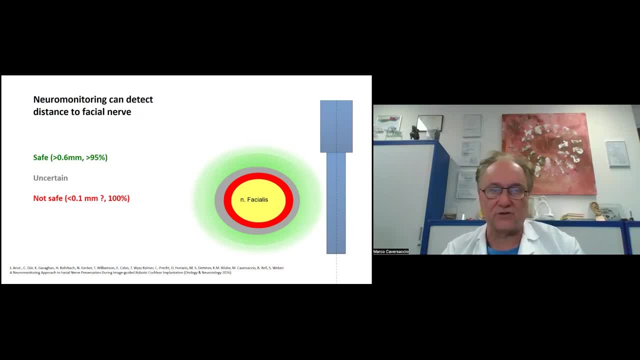 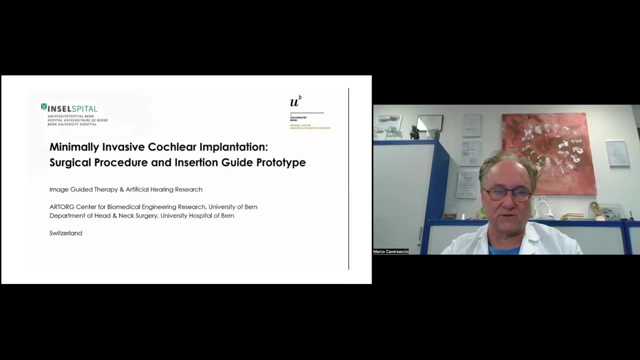 It depends on the heat. What is the temperature on the bone, and especially if you have muscles around the facial nerve? but this is one question and also perhaps in the future. And this is one question And also perhaps in the future: Instead to have a 1.8 millimeter, you have a little bit of 1.5 millimeter. 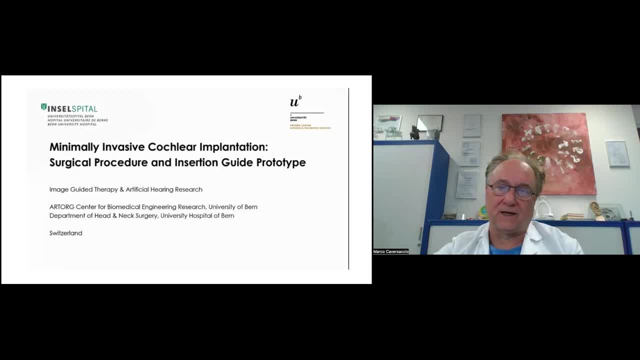 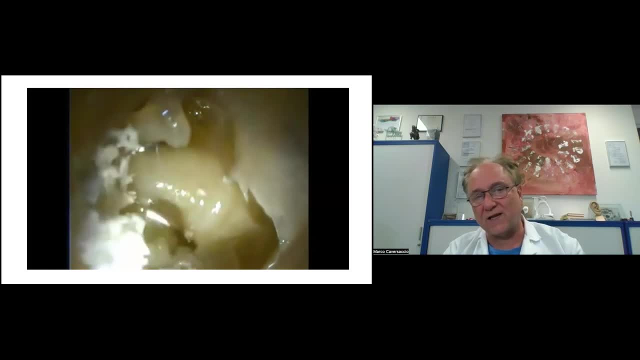 This is only one of the first. what we have performed Operation is only to go to the interior access. this will be. you see it, we drill it, but we have a 1.8 millimeter. we drill it and really, the way this canyon or the overhanging, 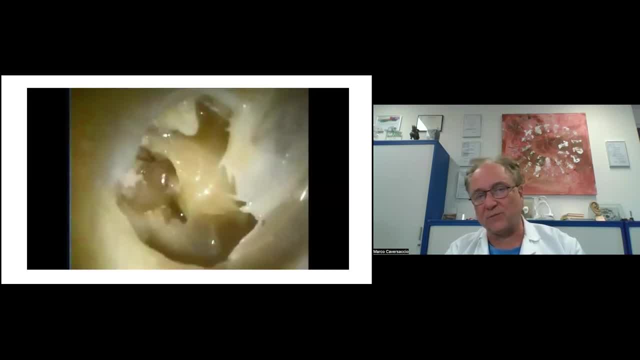 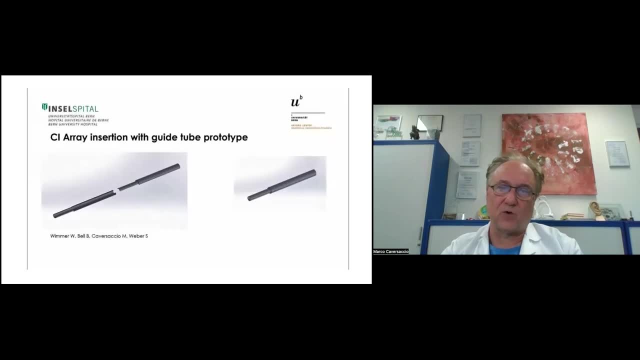 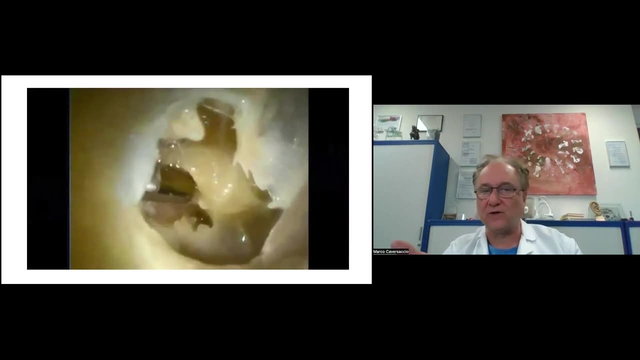 to the round window. This is also possible As a control, The control on the endoscope here. Good, And what is important is this guide to prototype, that you can see it, especially the shoe. It's like a shoe where you can put in the electrode completely in the injury. 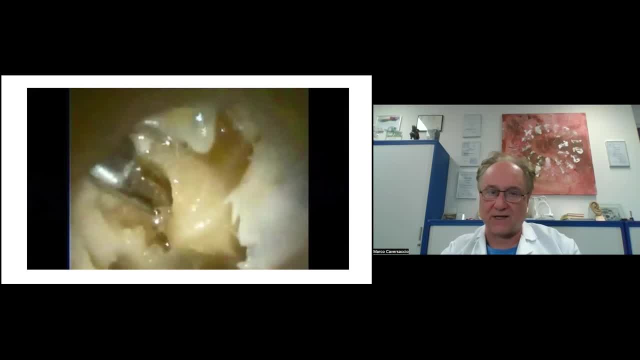 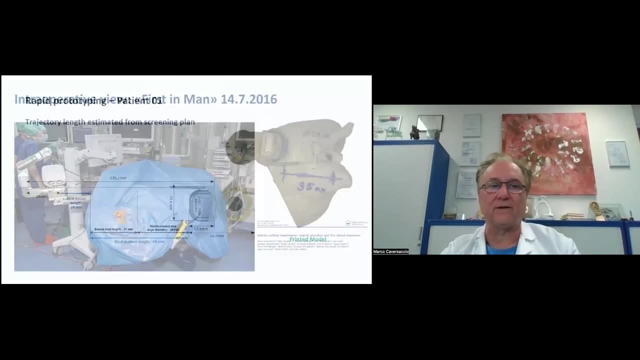 It's here. It's really rapidly. It's not open one millimeter per second to don't destroy this color company and to enter this color vestibule, but it's now better. Okay, Here We have performed 2016, the first operation on it. 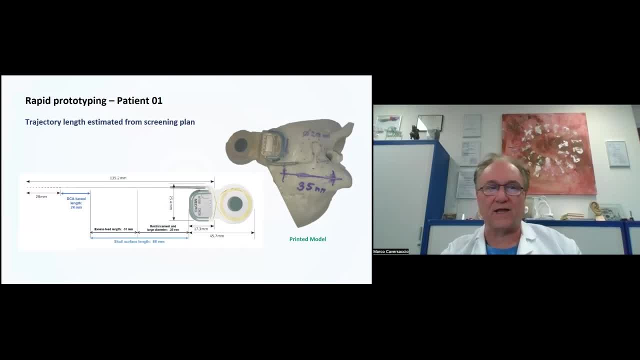 We have looked about trajectory events, about the rapid prototype, And you have measured the all of what is too much and what is normally the distance. But when you have a tunnel to the injuries, about what you can see, it here is about 24 millimeters. 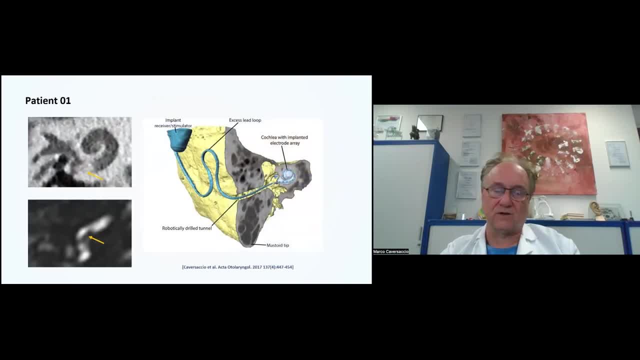 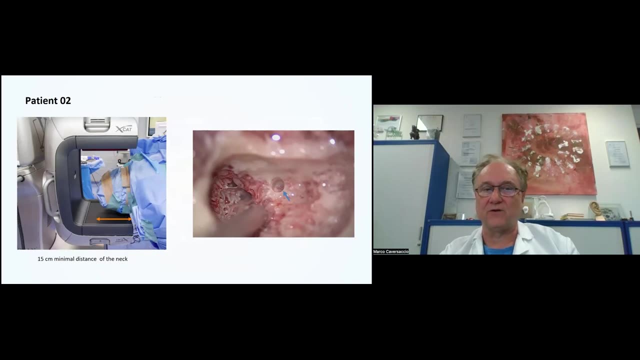 Sometimes it's 26 millimeters. The question is also if you must change it. I also told you you can change it: the, the ci, the, the size, etc. and the excess of the lead loop, what you can see it here. what is also must mention is sometimes when you have a neck who is too small, etc. 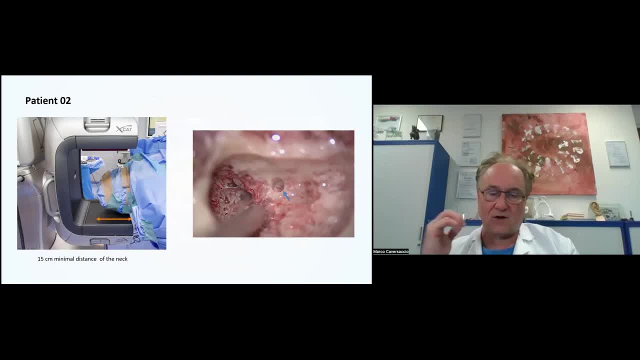 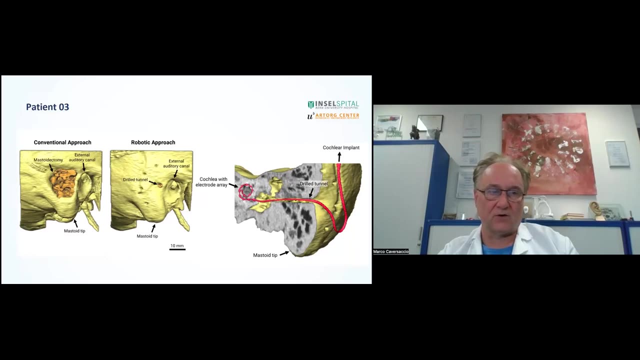 it's very difficult to use here the x cat. it exists now the large one, what is used also in uh by professor top sacral and. but in this case you have stopped the operation because you have not had the control during surgery. here on the left side you see a normal, conventional one. 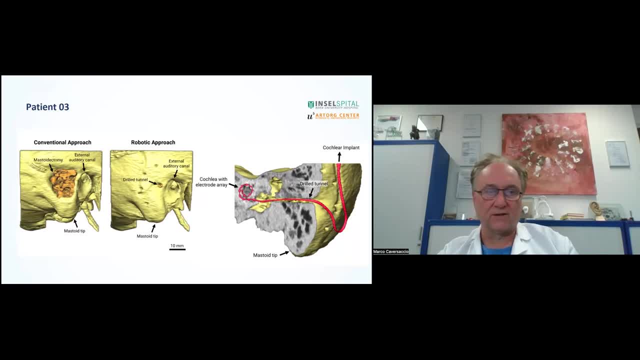 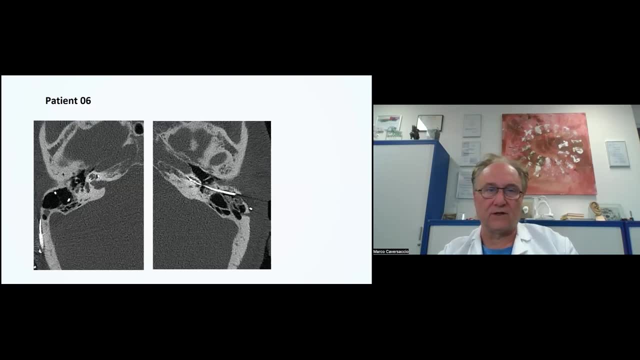 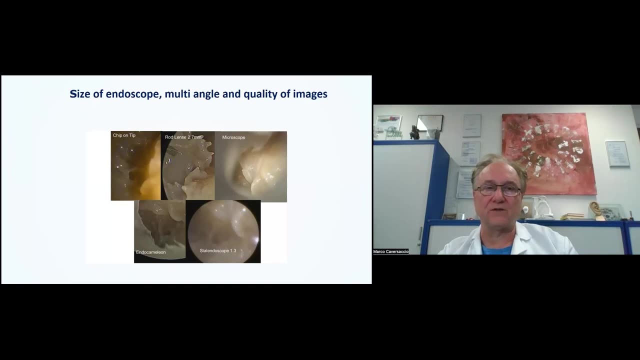 then on the on the other side, was performed the robotic drilled tunnel here, the city scan, normal mastoidectomy on the left side and on the right side. you see this tunnel procedure. what is also important, perhaps also for the future, is the uh, what kind of endoscopy can use? as you know, we 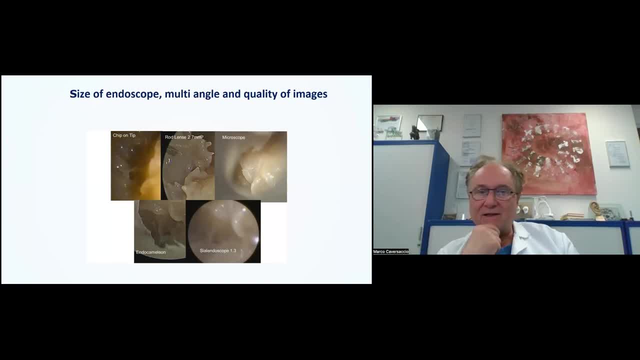 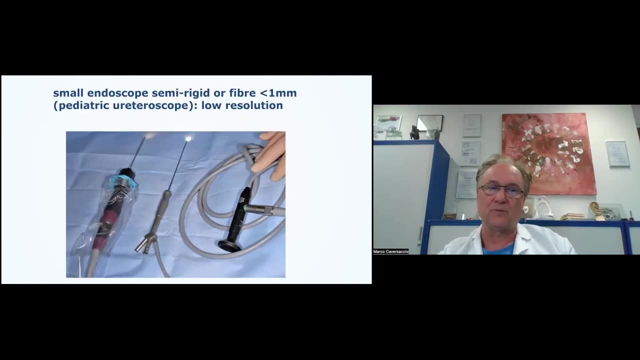 make uh till now a typical metal flap. they have looked also what kind of endoscopy can use. we have the cl endoscope. you can also use chip on the tip, roadlands microscope and also to look about the quality, what you can have with your endoscope. they have used also pediatric ureteroscope. 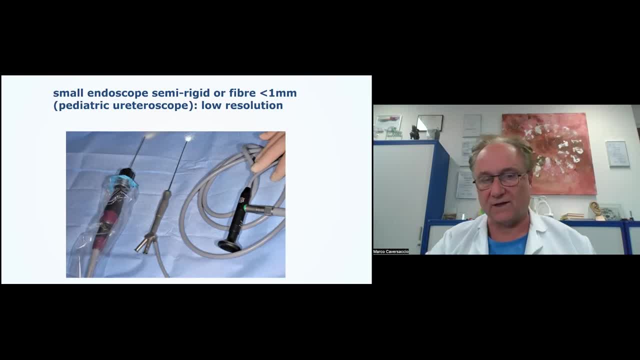 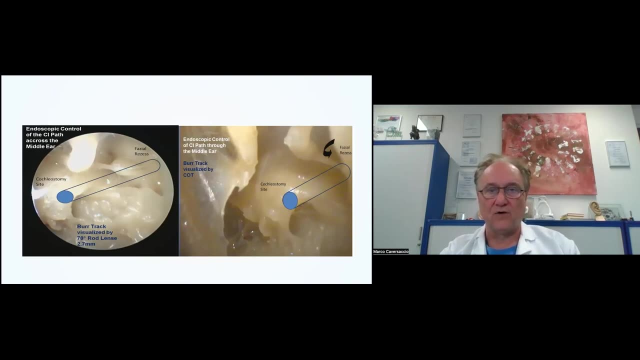 below one millimeter. the people who made cell endoscopy know exactly that we have a low resolution since many years and we have not a high quality of resolution. you can also look about how to control it and just copy control of the ci path through the middle ear. it gives you a little bit more information. 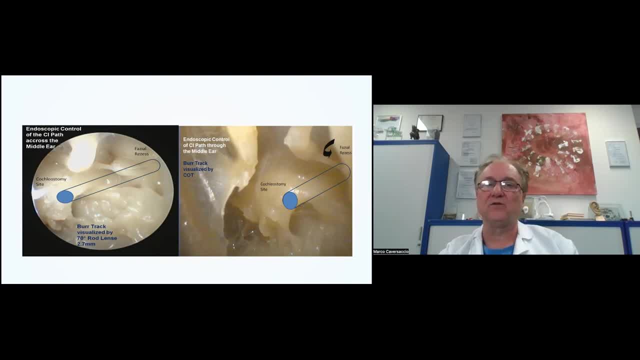 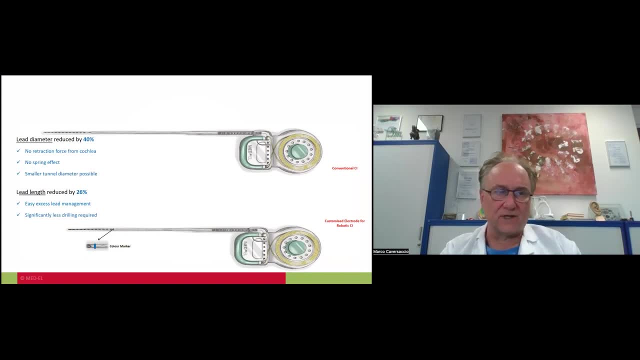 about the middle ear is not necessary, but it gives you more anatomical information here to have looked about the to reduce the lip diameter as well the lead length, to have not excess lead or loop. here you see, then, one patient has had a very good result in this case. 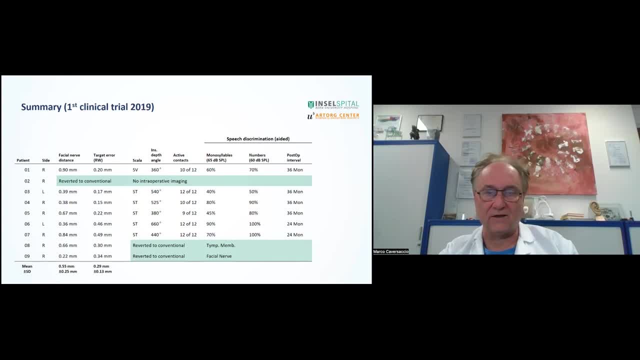 here. the results of the first clinical trial have stopped three cases in this. but when you look about the target error- and this is important- it must be below 0.5 millimeters and i've also looked about that. we have a good distance facial nerve distance of 0.5 millimeters. it's clear perhaps 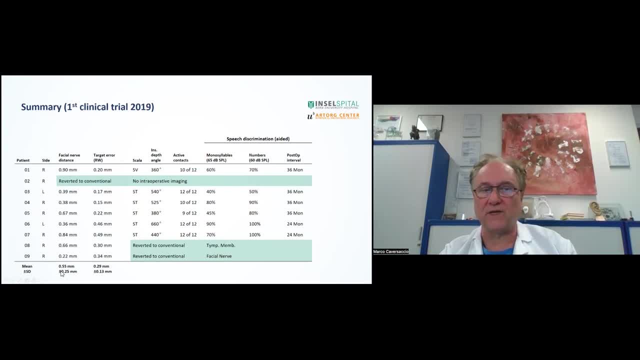 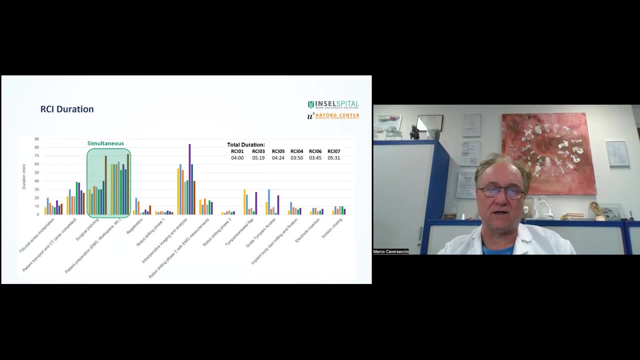 you can go a little bit more low. this means oh plus minus 0.25. this mean in one case we were about 0.3 millimeter from the facial nerve. what we see is here is the duration. it's clear it's still an ongoing work. we need a lot of time for the planning system, patient preparation, local. 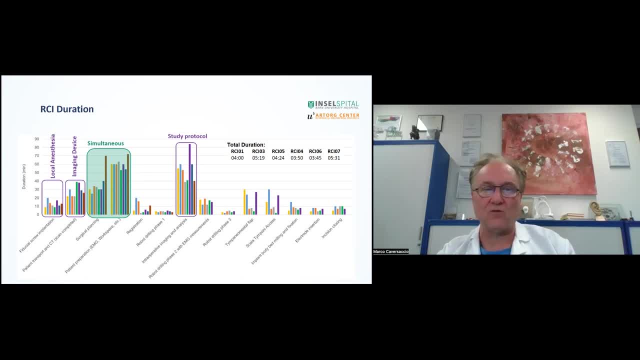 anesthesia and imaging guidance. we have had four hours. we know that some groups has only have 2.5 hours and i think this is very good, but we have integrated a lot of safety procedure, as you have seen with the intraoperative city scan. we have medical engineer peer groups. we 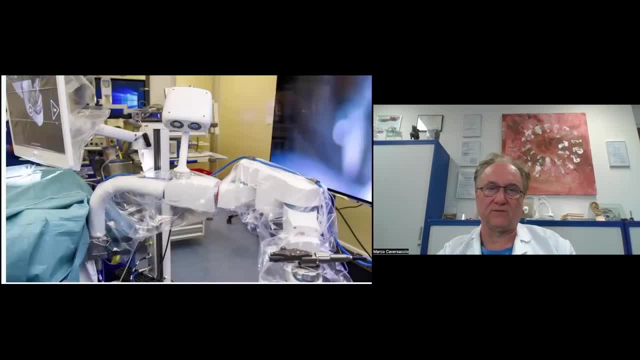 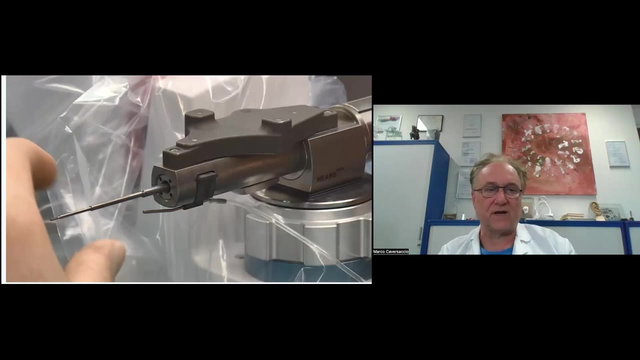 have new radiologists as intraoperatively, and that was mentioned i. i think the beginning by nicola and professor vedatopsakar is the inner ear approach, what they have already shown you, but what you have now is a one millimeter- uh, bird, a diamond that you can have. 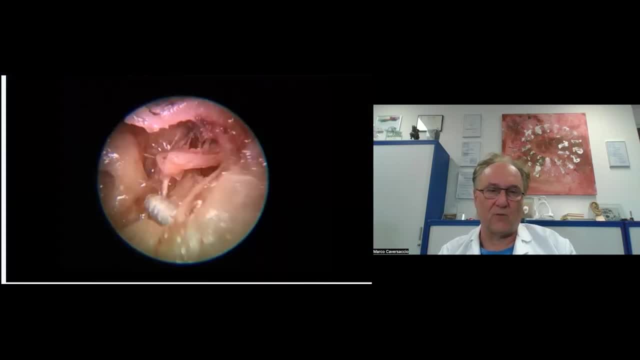 and you can uh drill away. in fact, uh, here, the overhanging, or the cannon, as was mentioned by vedat to open. here i'm going to the inner ear. this is the mean. the step three to go inside here is also on the control of the endoscope. you must change a little bit the head. 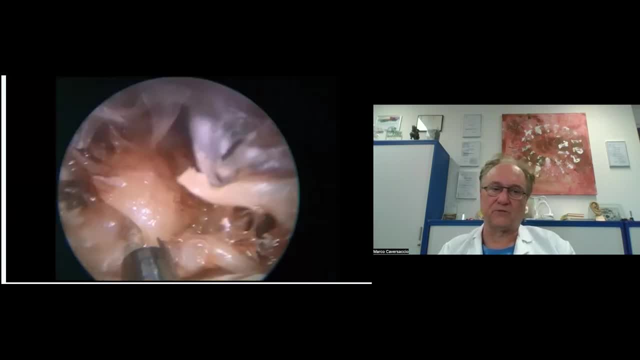 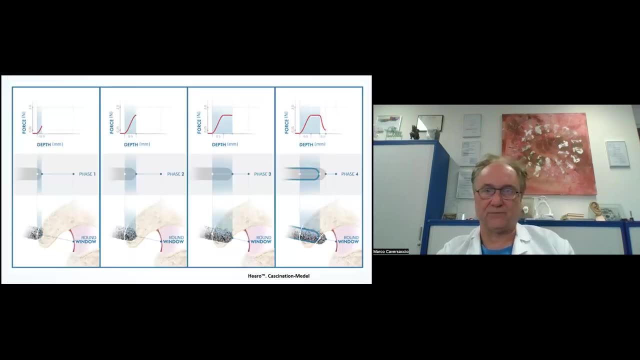 because normally endoscopic slurter you perform on a flat head when you make a microscope search is more on a hyper extension here. this is this uh visualization again of this uh round window approach. you can measure the fourth step that you see on the top and you know exactly when you reach. 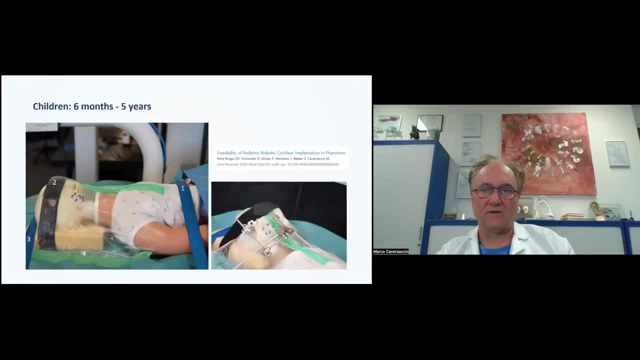 the membrane of the round window. we have also looked about children. theoretically is possible, because, uh, but what you can see, did the screw. that's very big one, and this is, uh, one of this problem. what we have, we have also not- it's clearly not cut our head for- of children that we can use. 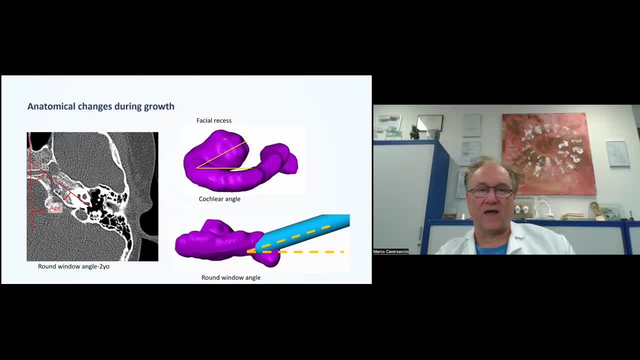 it, uh, to make some experiments. we have also what is important when you look about operations: young children cochlear angle, and then the young children cochlear angle and then the young children cochlear angle. random wing angle is not the same when you operate a child of four months than an adult of 20 years. 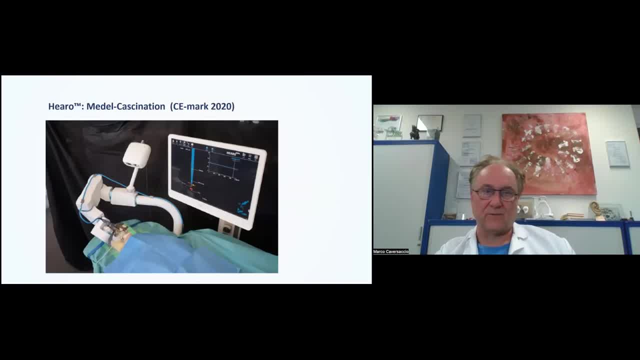 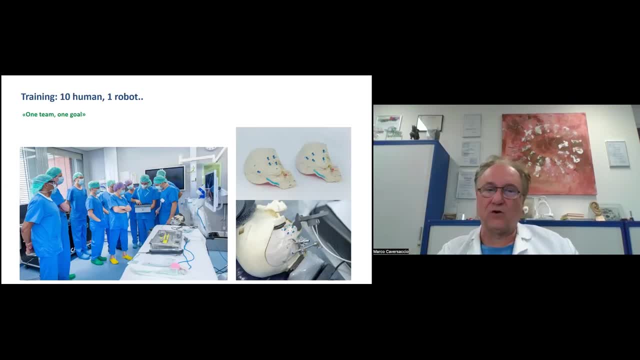 old then was the 2020, the metal cast in nation, the hero one, uh, one thing i show you here 30 years ago was one man, one show, uh, the one goal. today you have one team, one goal: you must integrate medical engineer, anesthesia staff, et cetera, et cetera. this means you have more and more people. 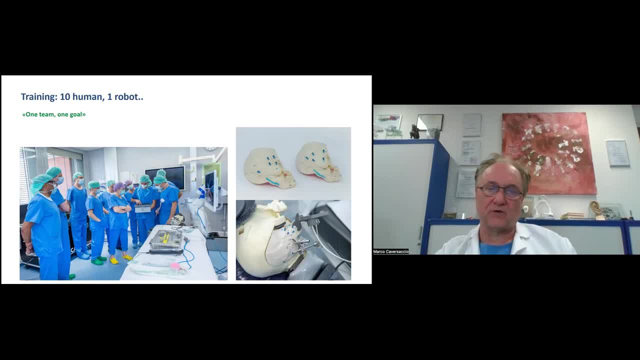 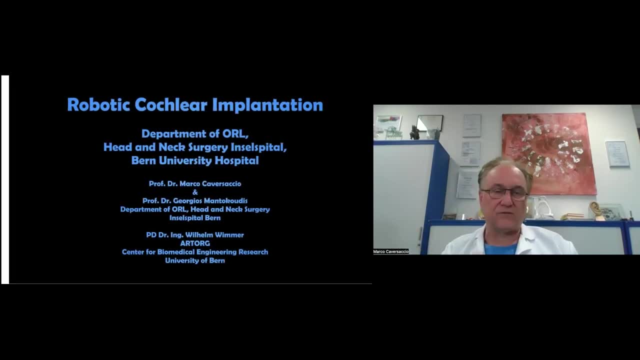 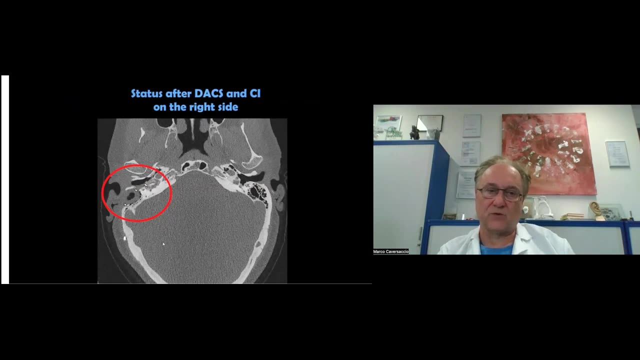 in the, in the or and preoperatively than perhaps 30 years ago, as we formed the clinical trivalent trials. and i show you one of this operation we have this advanced auto sclerosis we have on one side was operated with the ci and especially with ready to have a direct acoustic cochlear. 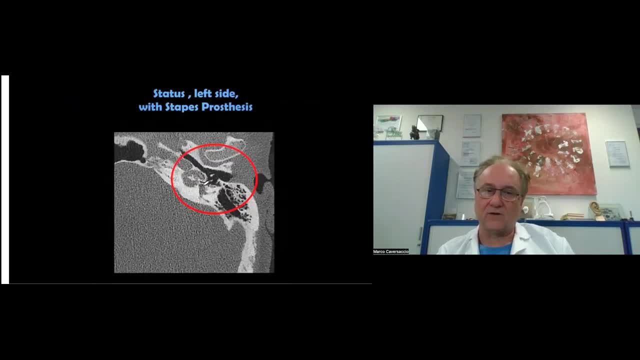 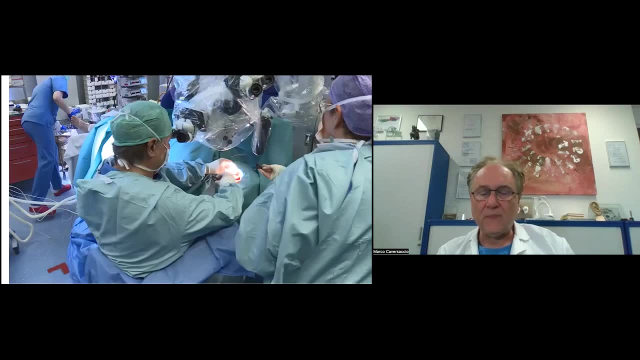 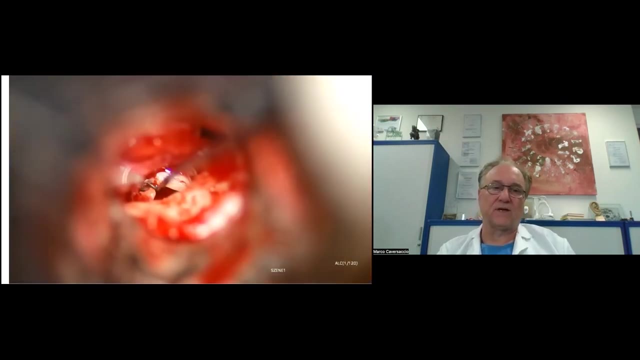 and on the left side you see a destroyed inner ear of the cochlea with a piston in place. this is the audiogram just before the operation, and the first thing, what you take away is during the surgery. this is the stoppage procedure. it's clear. you can let it inside. perhaps you have then. 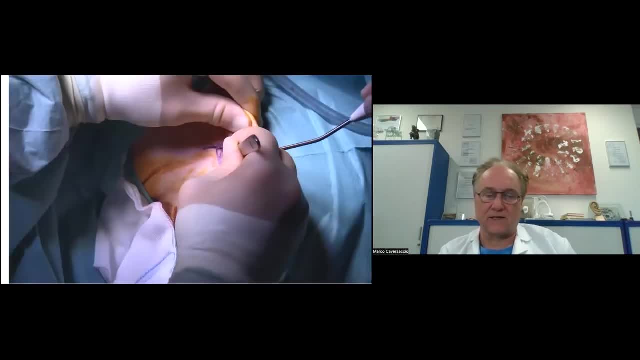 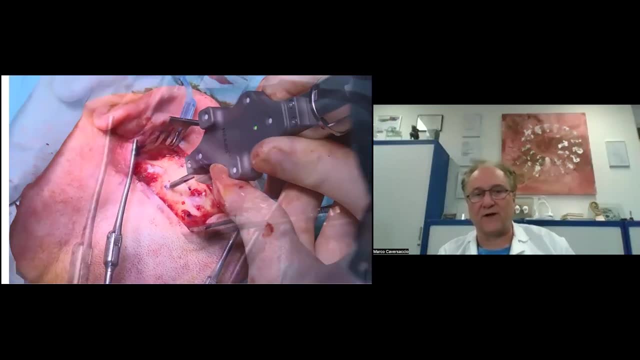 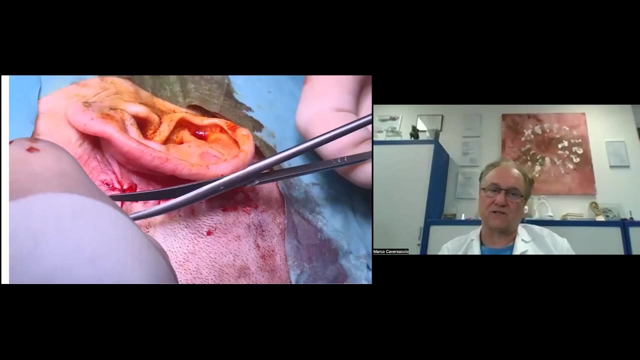 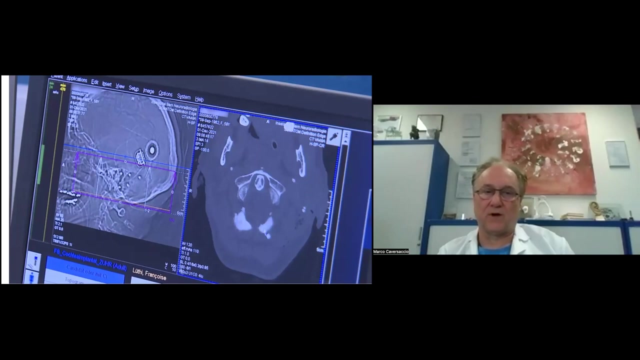 uh yeah, problems with the, with the disequilibrium or vertical. then you open, uh, the skin and you put here the five screws is four screws and one is for the dynamic reference space. the dynamic reference space is important and especially that the navigation control, uh, navigation system control, the robot system. here you look about the. 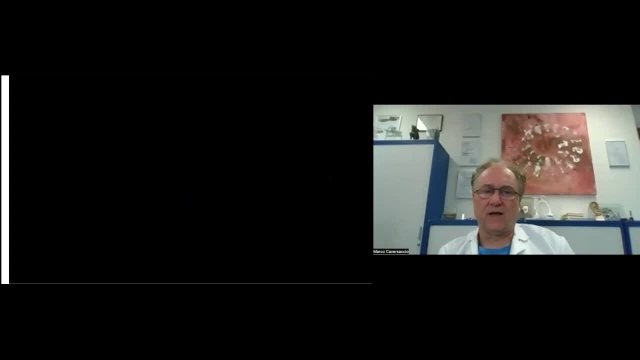 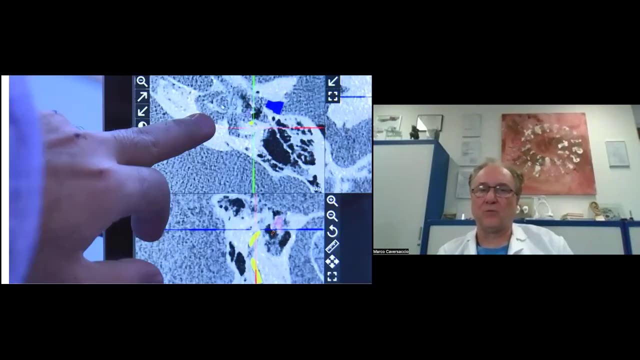 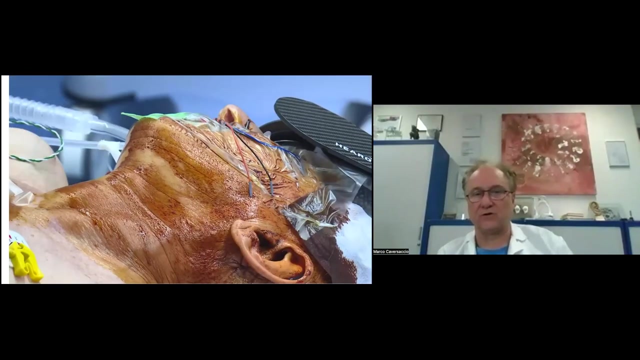 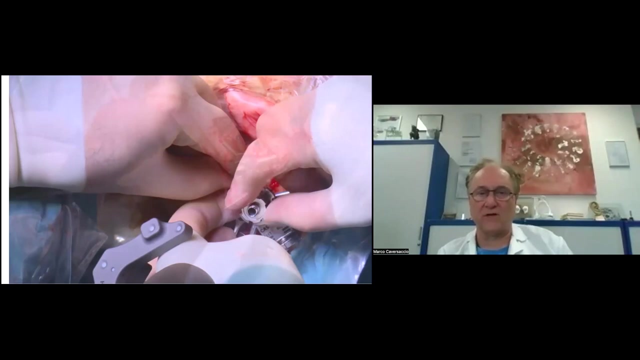 screws. that is in exact position. and here was this important medical engineer. this is a semi-automatic segmentation. it's not completely automatic segmentation- to look where is the best way, the trajectory in this, uh, during the surgery. here you see the facial nerve monitoring. here see, you see the axles camera. this is for the navigation system. here. 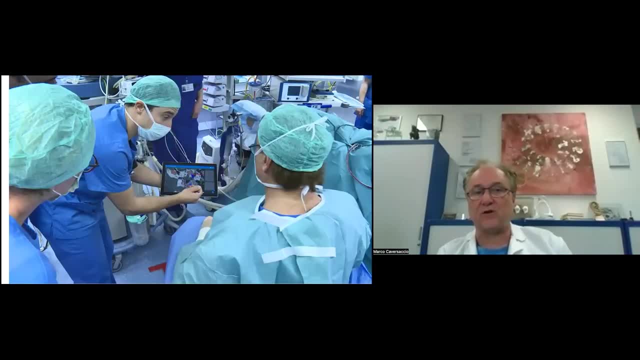 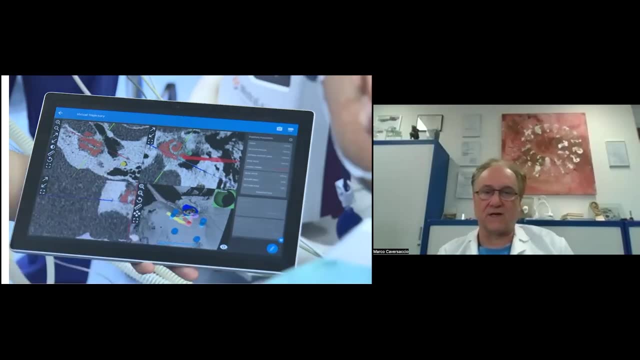 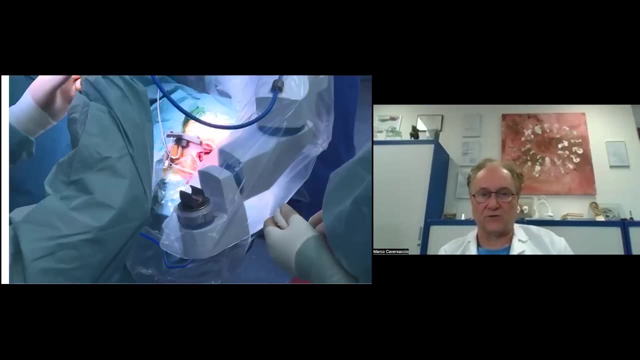 you put the dynamic reference base and here we discuss again about the trajectory, what, what is the best way? you have, uh, three piers in fact, and then we discussed then, especially to know exactly the different way, and especially the distance of the facial nerve, and this is clear. 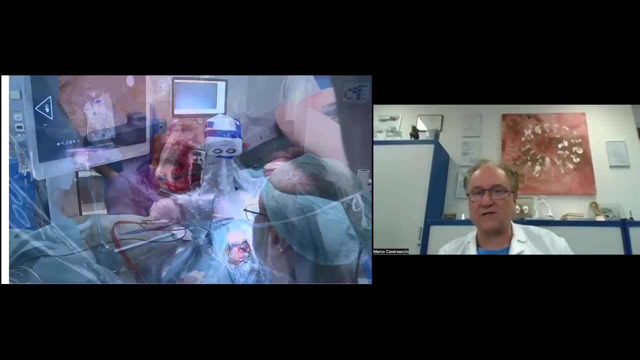 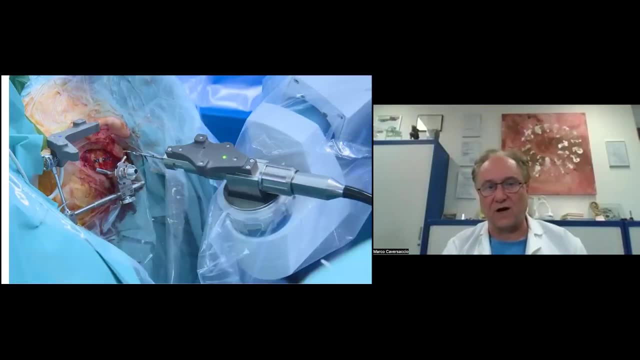 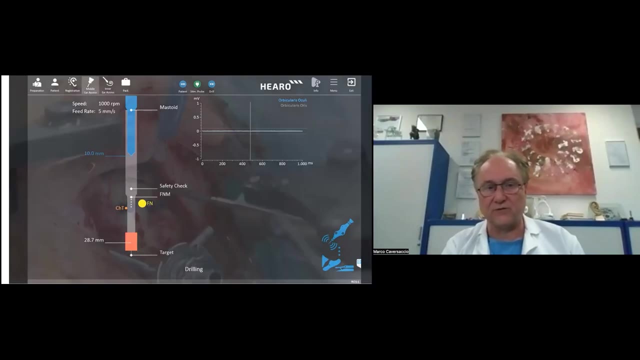 at the beginning you make also a registration. this is important to look about the accuracy, the precision of the system. and then you start, and this is a certain task: autonomy. here you can visualize on the monitor the distance to the fashion, love to the quarter, timpani and you. 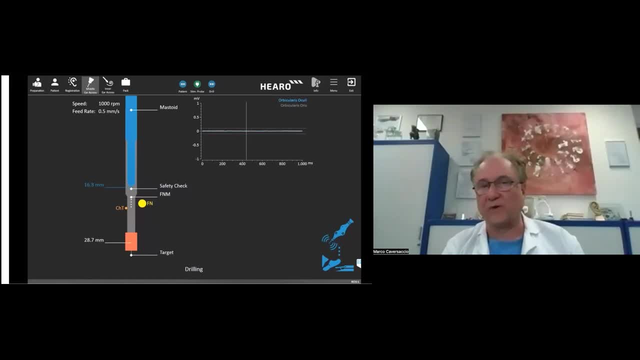 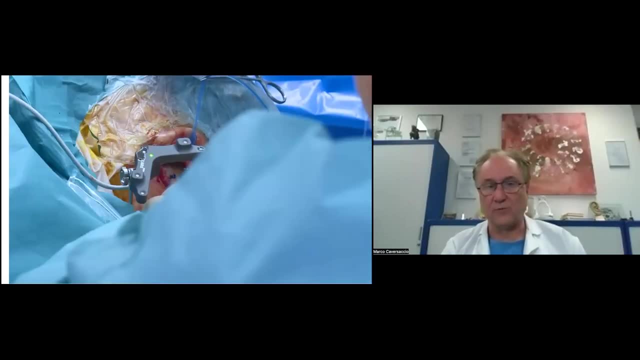 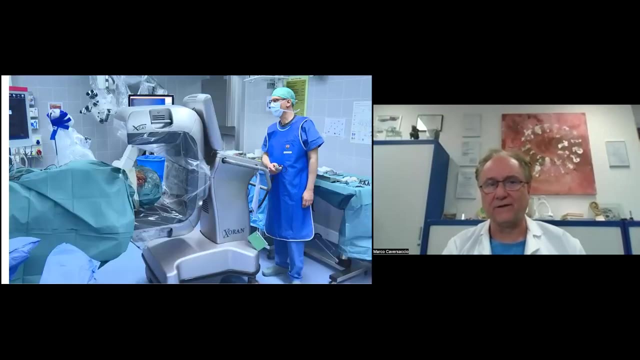 progress here shortly, with a thousand round per minute, it's not thirty thousand. when in then you make a safety check before you enter the posterior tympanotomy, you take away the dynamic reference base, you make what i've shown you, the xcat, and then we continue again. you make: 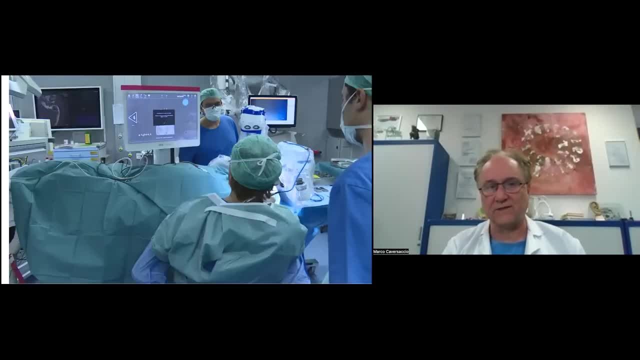 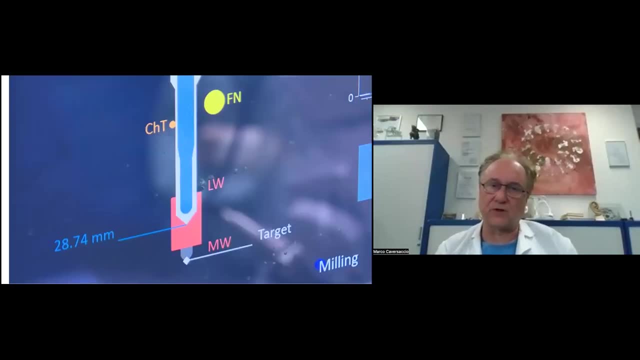 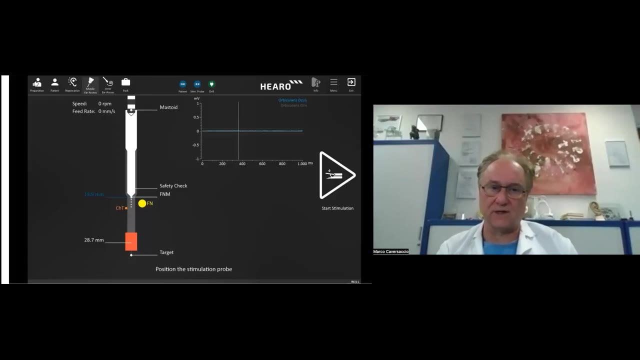 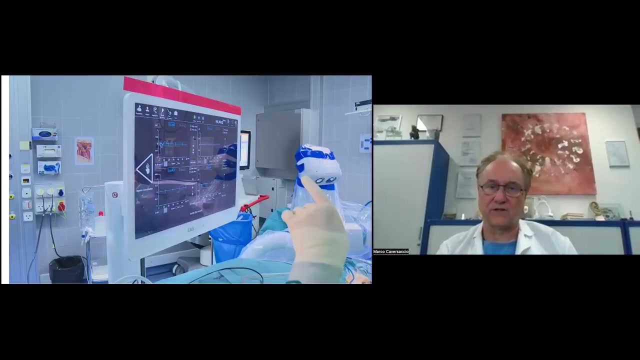 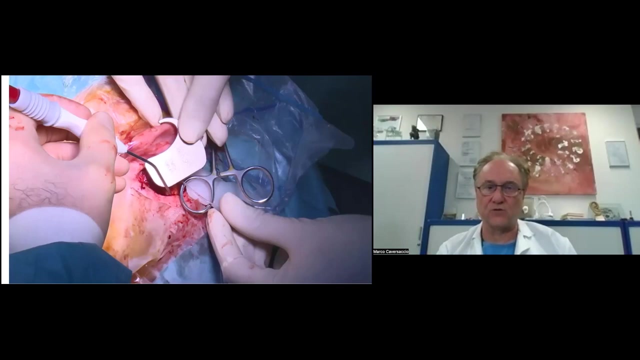 this a registration again to visualize this. and then we continue to make the small steps during the posterior tympanotomy and we control them also with the vaginal nerve, monitoring what you can see here to look about if you have good results that you are not aware inside of going to the facial nerve. and then we put this ci in this one with this guide tube and 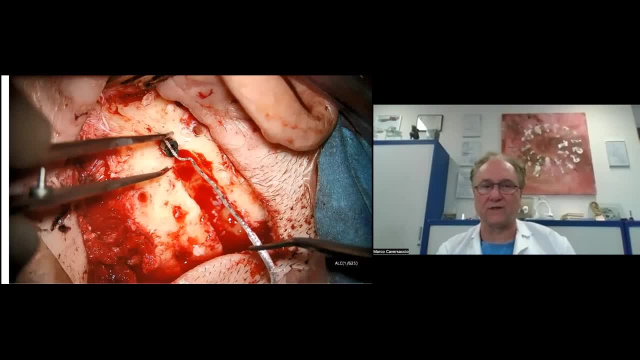 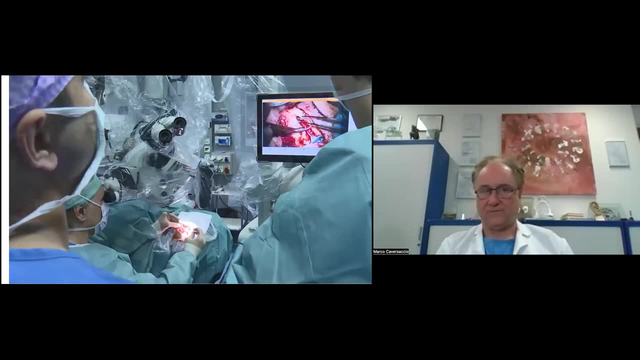 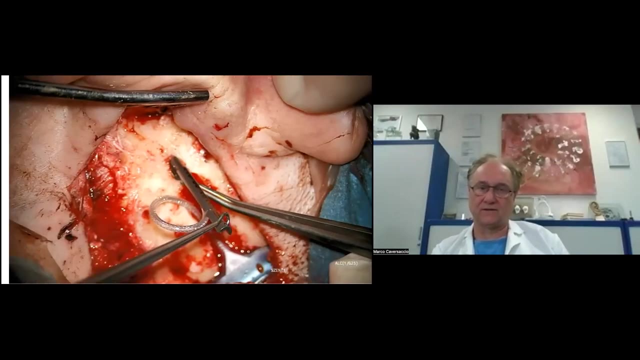 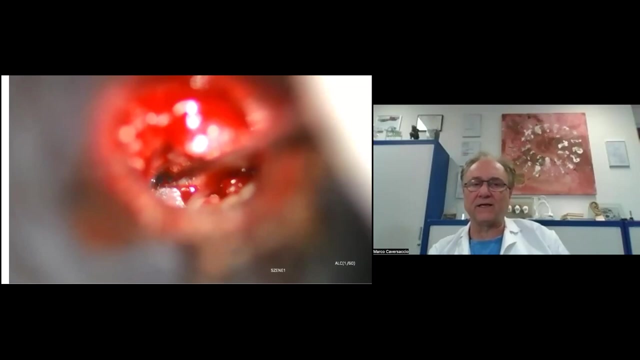 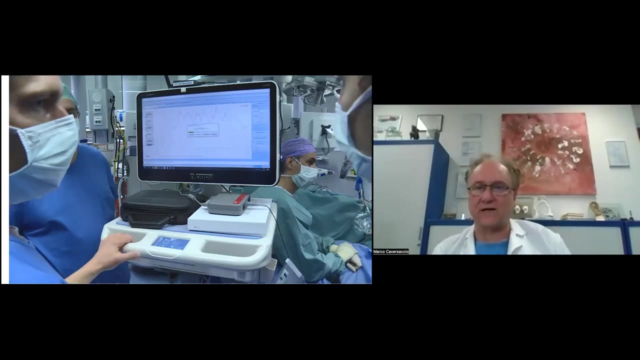 neutral the bed inside and take it out and in this case we put in the electrode inside the cochlea. how we perform in this case and we take here away the guide tube, how we can see it and it is clear at the beginning: we have, we have not had a result, good results during the surgery. sometimes you have air inside the fluid. 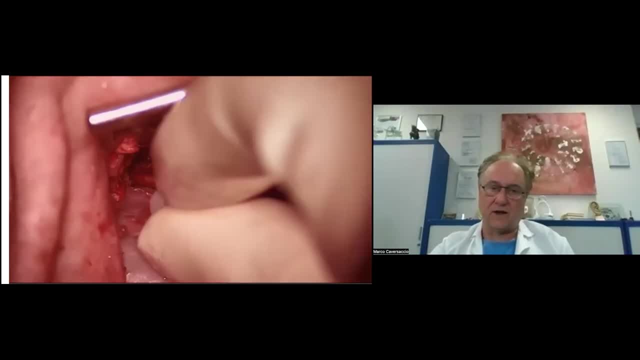 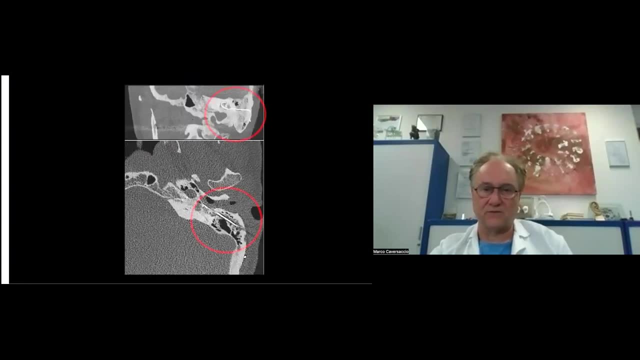 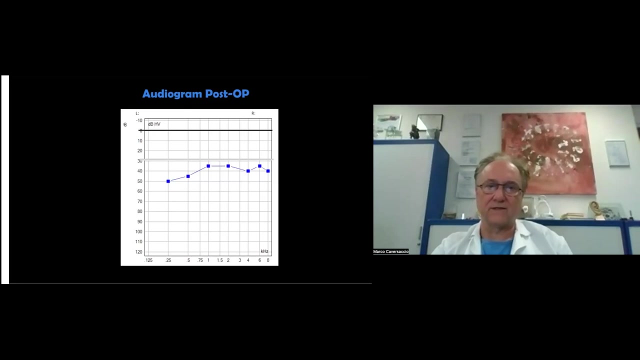 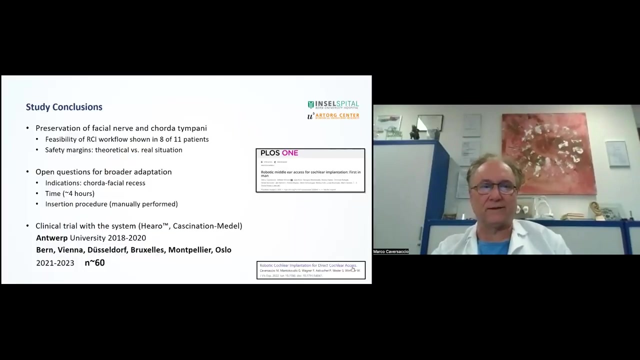 etc. and we have then, after the operation, we perform also a ct scan or the cone beam ct to visualize this, and we have had a good insertion on this side and we have also had a good result in this case. good now, this is our study conclusion. we have had, we have now 12 patients. the feasibility is. 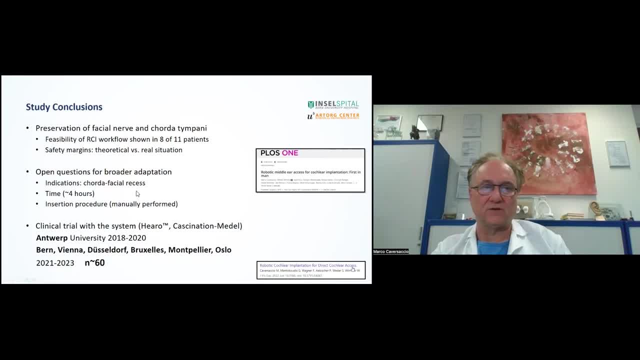 possible. it's still. we have open question about the court of facial recess. the time when you take away or all the security is clear. perhaps you can perform this in two hours is possible. uh, what we have seen is now: uh, antwerp group then is burn, is vienna- i think i've performed six cases- bristol montpellier. 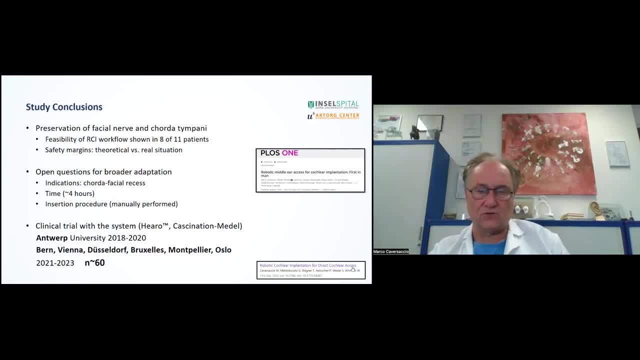 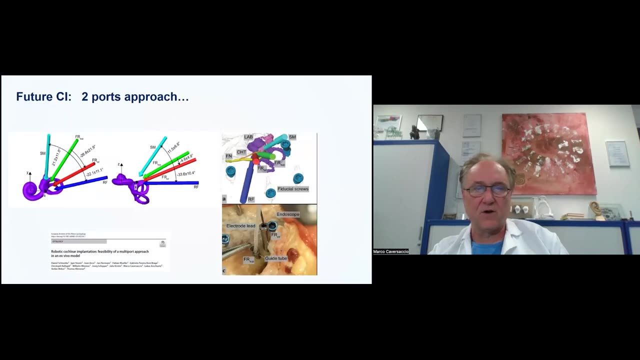 and i think last week oslo. i'm not about uh sure about the number, but what i know from massoud is between 50 and 60 cases now in europe. for the future is the question about the two port approaches, if this is possible to get in also an endoscope or make a total surgery or only concentrate on. 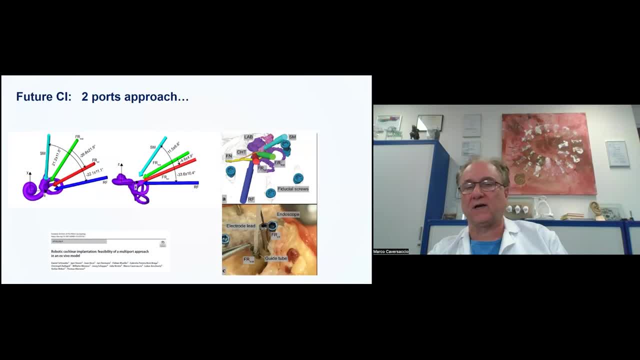 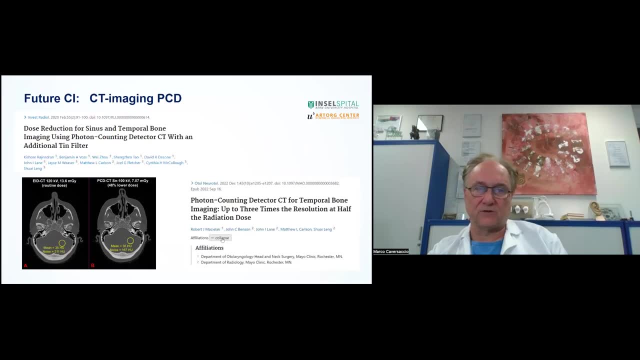 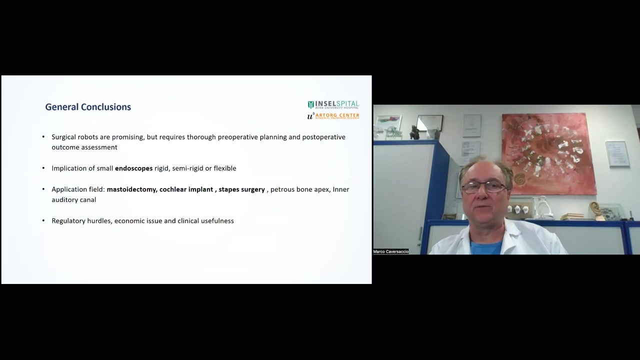 the last step. this mean a partial robotic assisted surgery to make for hearing preservation surgery. another possibility is also for the future to to better have results is perhaps the city imaging with this new photon counting detector. a general conclusion- uh, these are the robots are promising- is clear implication of small endoscope. uh, also in. 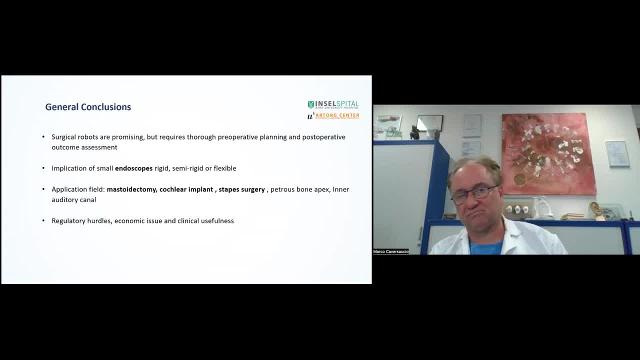 the future. the question is also remain: a keyhole procedure or a mastoidectomy? a total robot approach or only a partial robotic approach? what is performed until now by yota motion? it is clear the regulatory economic issue, the reimbursement uh must be performed and the clinical use for an 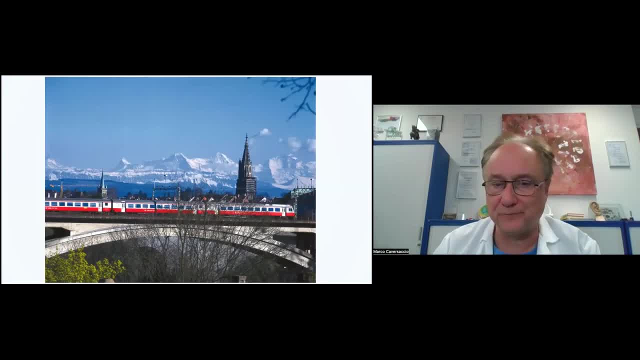 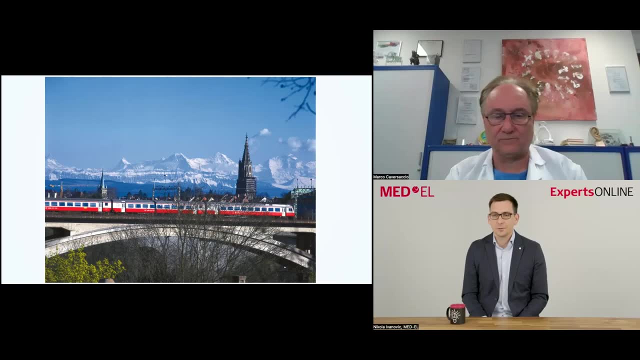 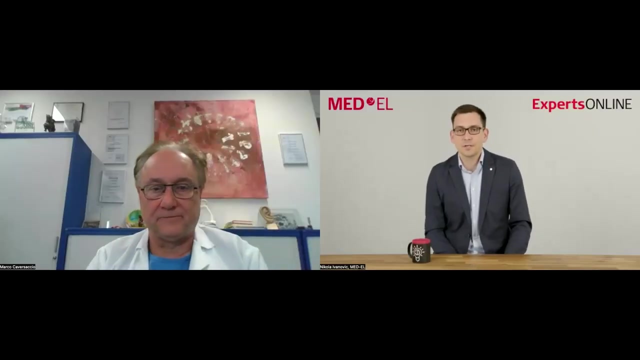 off. thank you very much and i open for question. thank you so much, professor carlos, for this uh, not only comprehensive uh journey through robotics and ontology, but also through history. um, we have one question in the chat. it's for you, but uh, maybe professor topstar could also give his opinion um after you, because it's it's. the question is. 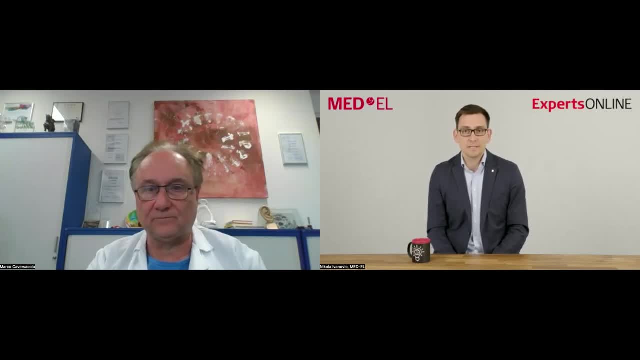 do you have any problems in electrode array migration movements? after in surgeon, while pulling out the insertion tape? we saw that in some of your videos. so once removing uh the insertion tube, is there any migration happening on the electrodes? i think it's. it could be possible. i agree with if, uh, when you look about the 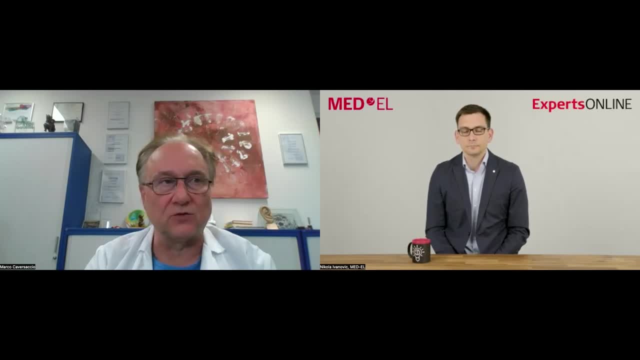 the video etc. it could be one or two electrodes. it's not so clear because we have not completely controlled, but we see the same that you pull back a little bit in other cases. i've also seen with robotol one time that also with robotol you have. 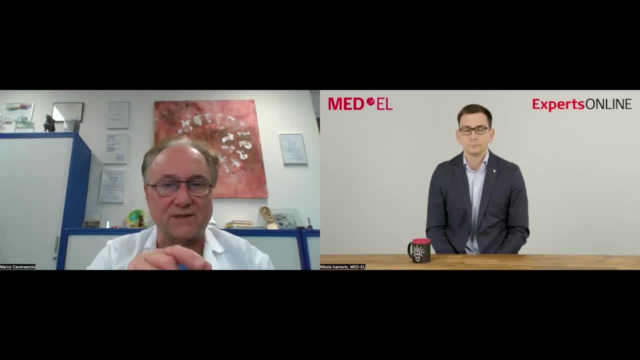 not completely because you have this clamp, etc. it must be the same- what i have heard also from the us also: sometimes when you put it in, when you have some resistance, then you must put it back, etc. i think this remain a problem, but also in the future, because when you need, then it's like a 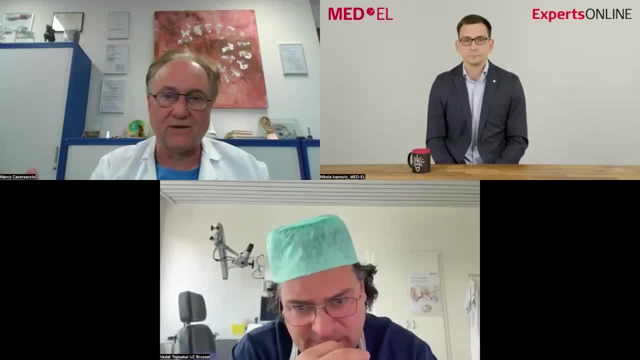 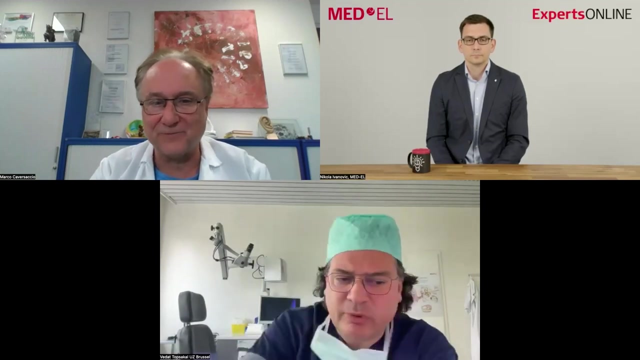 push on to close completely and go away, and uh, that's what i think it's, uh, but it must be perhaps one electrode, but not in each case, but perhaps that could also uh say something about this, i don't know. no, i fully agree and and thank you for a really very comprehensive overview, it's. 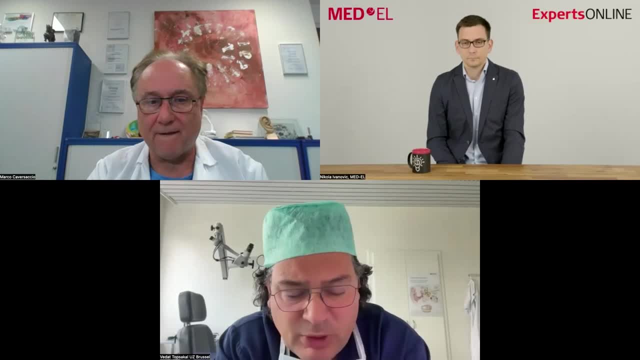 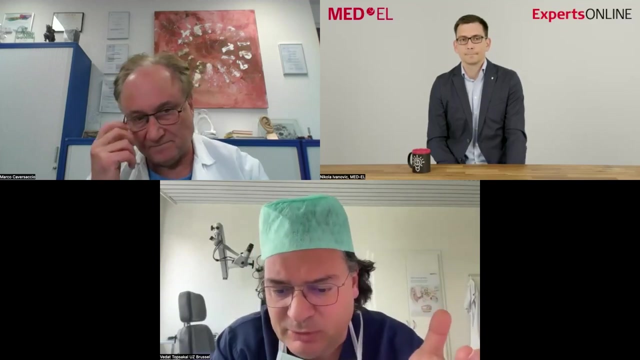 very enjoyable to see what has been performed before and where we are now. and to come back to that delicate step. yes, it's technically possible, but we've also seen you take away the piston. you know we play stapes pistons. you have to be careful and in an unattentive moment this could happen. but if you take care of it, i have to say. 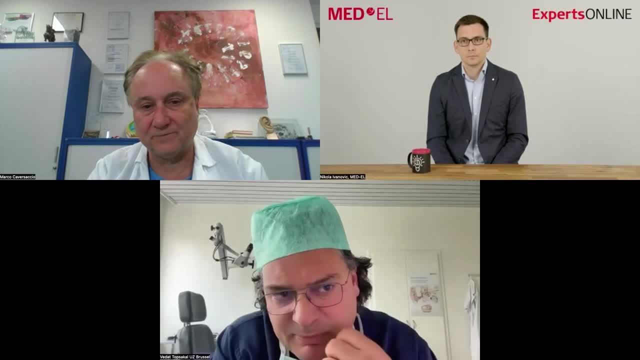 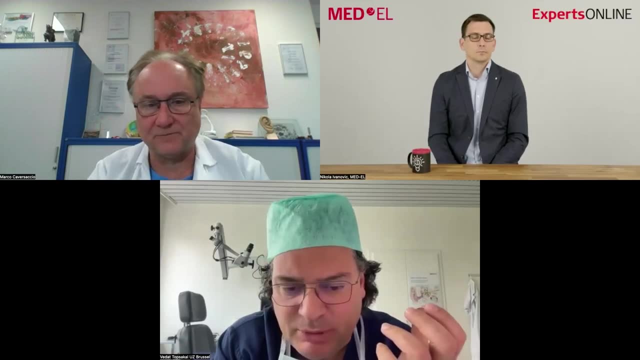 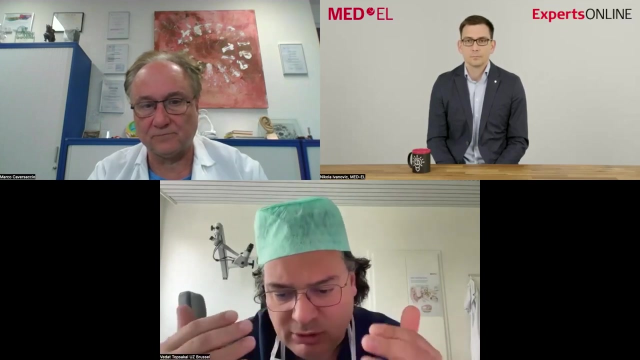 it was not a big big issue, but it technically could happen. um, i mean, yeah, you also see that it happens because we immediately perform a post-operative combi ct. um, i don't think that was the problem, but i have to say it was one case where we could not really have a full 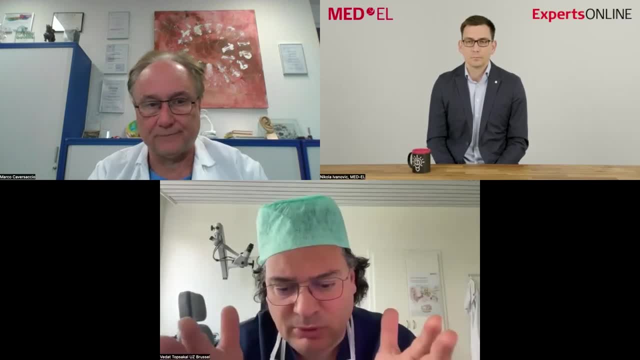 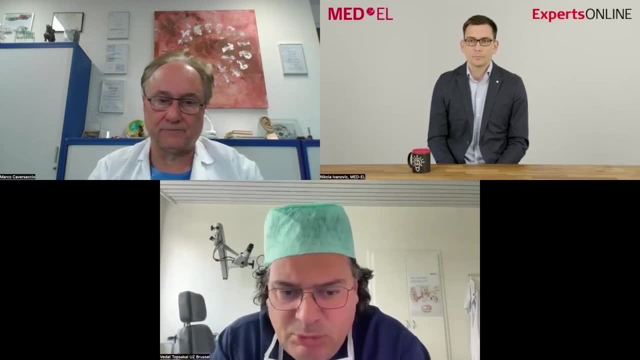 insertion and and then yeah, there is no time to also adjust that trajectory or manipulate in the depth. that's make a problem. when you have a little bit of inaccuracy, that's a bigger problem than dealing with the- uh, let's say, insertion tube to take away. thank you. there's another question: how? 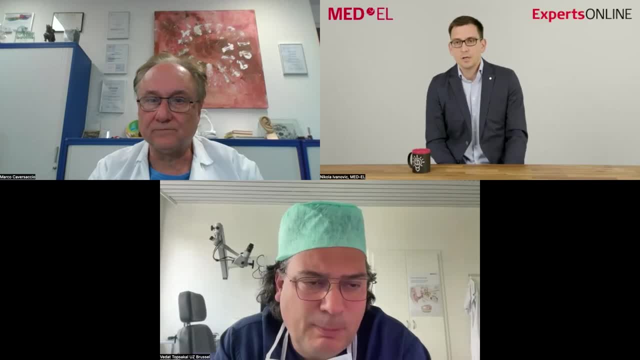 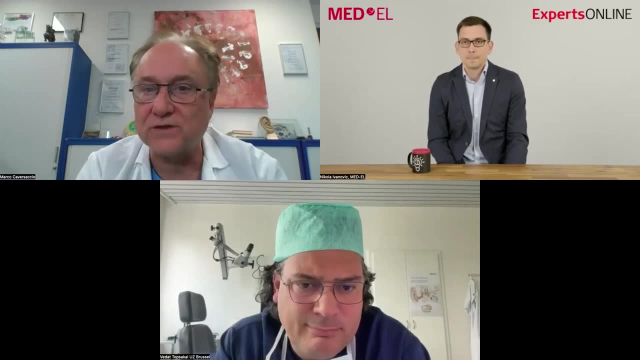 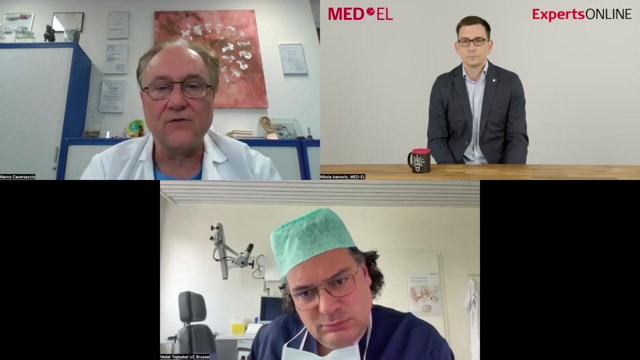 frequently intraoperative cbcts are used for navigation and electrovisualization during ci surgeries. i can say normally we don't use it when only in children, but where we have young children, because until now for the fitting strategy we still use ct scan and when we have small children until five, six years instead to make post-operatively. 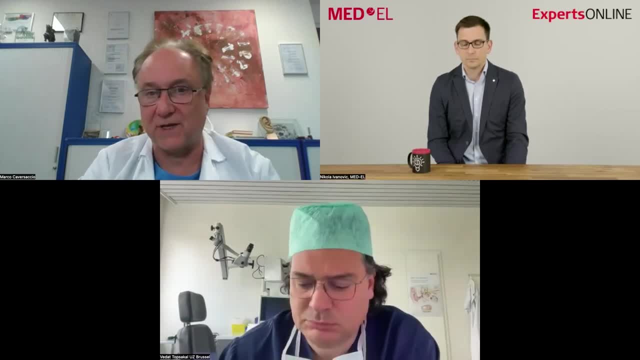 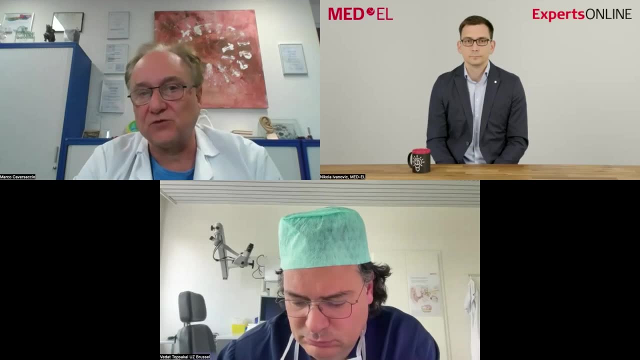 a city scan we do during the surgery. does it mean after the surgery we make a combi ct directly in the oar? like this we have to result. perhaps in the future it is not more necessary. we can all everything based on impedance, but until now we use it to especially during children in adults. 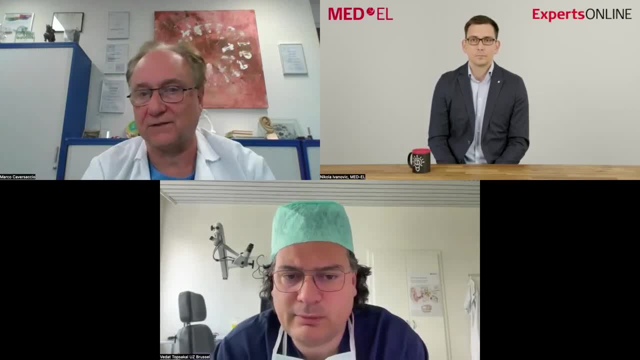 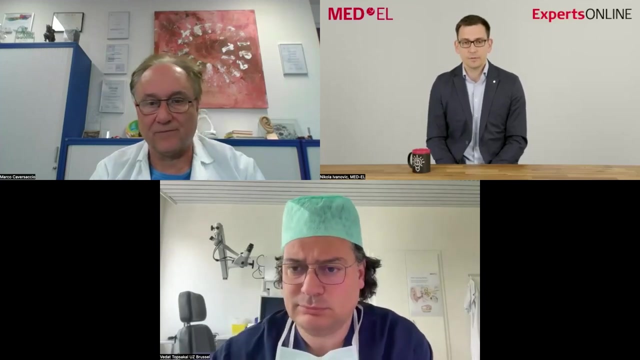 you can perform this later on, several days later. thank you, okay. we don't have any further questions and it's 4 pm. once again, thank you so much, both of you, for for sharing your your enormous experience in this field and all the findings um. I would like just to ask participants if we 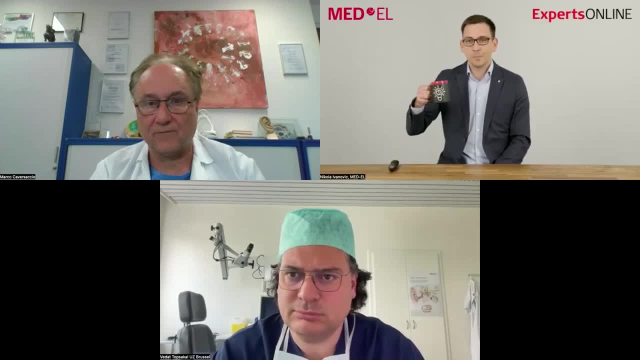 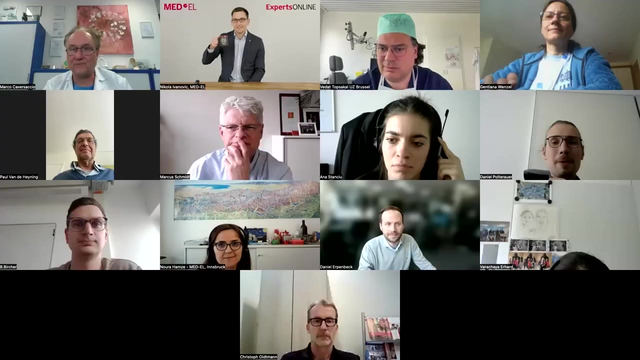 can switch on the camera just shortly and have the digital virtual group picture together. um, so please switch on your cameras. this is a tradition that we are trying to maintain and the video you saw in the beginning actually came from one of those pictures. excellent, thank you so much, and I encourage you all. 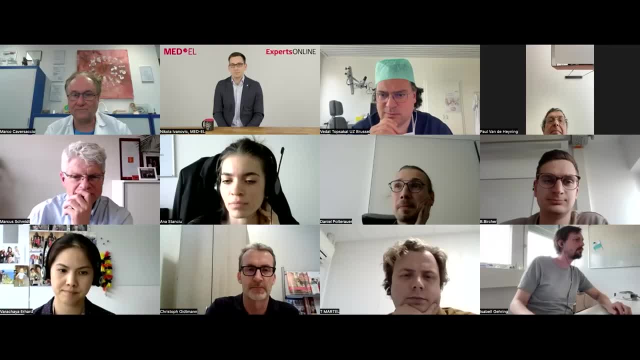 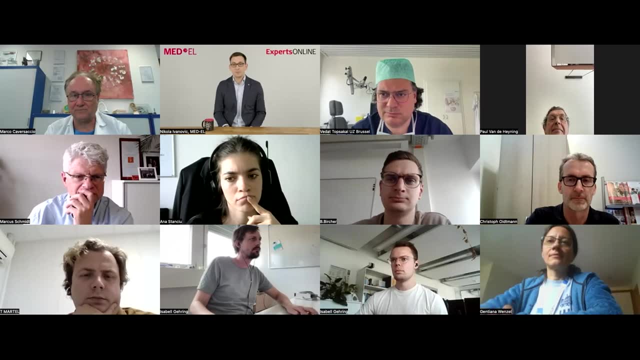 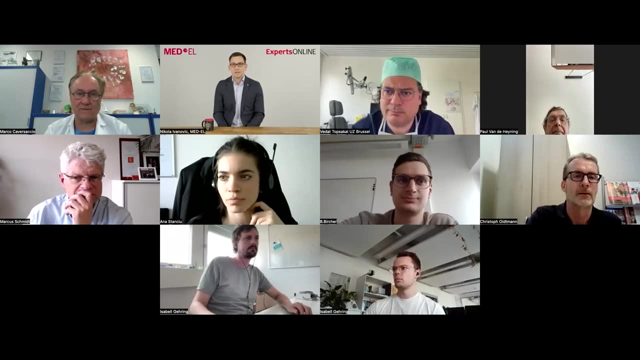 um our, our participants here, to uh look for all the the publications that were cited throughout this um this session, because there are a lot, covering many different topics, all the cases treated with hiero, autoplan, validations and many, many more. once again, thank you, Professor kavasatcha. 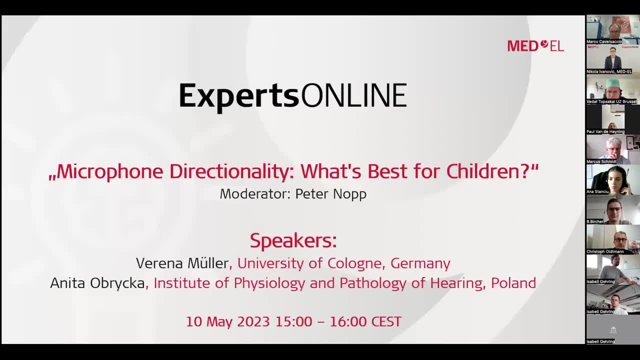 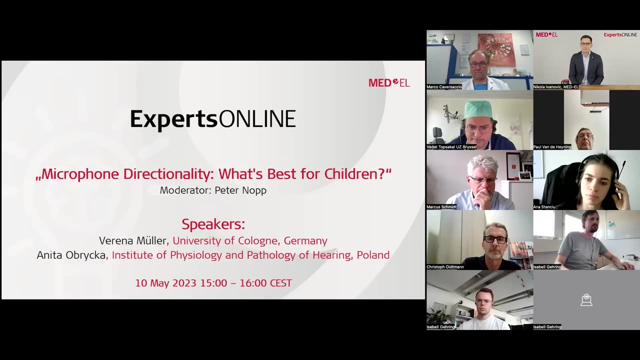 thank you, Professor top cycle, for your for your time and your presentations, and I would like to invite you all um for our next experts online session, which is in two weeks, where we will have the topic of microphone directionality. um Peter Nob will be the moderator and we will have speakers Verena Muller and Anita obitska.